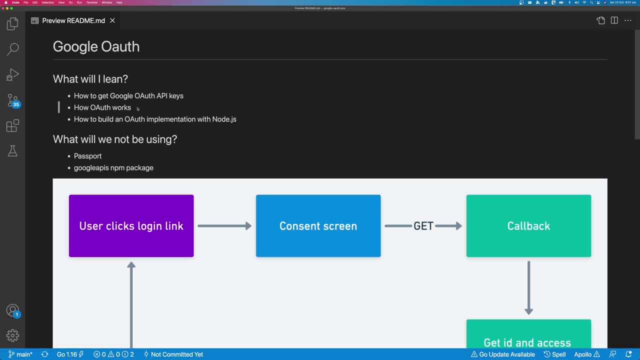 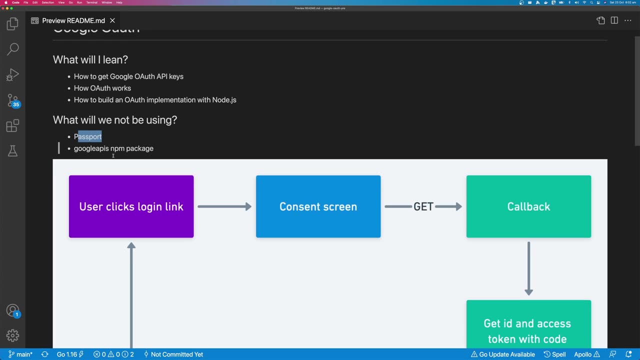 API keys. You're going to learn how OAuth works And you're going to learn how to build an OAuth integration from scratch with Nodejs. So what will we not be using? We're not going to use Passport and we're not going to use Google API's npm package, And the reason we're not going to. 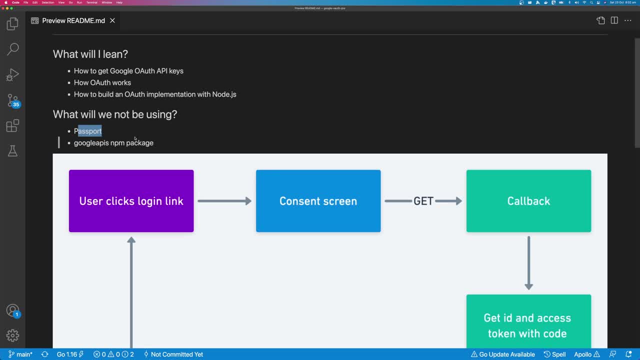 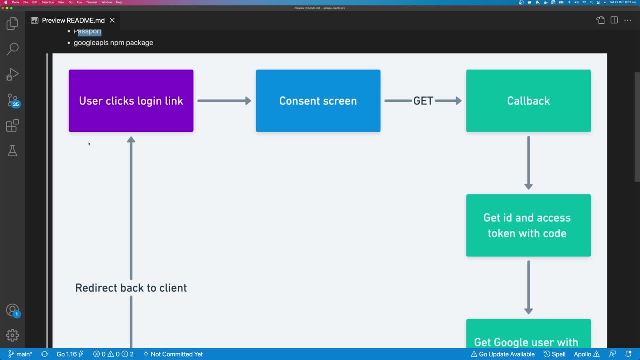 use either of these is because, if we don't, you'll be able to see every single request that's happening behind the scenes and you're going to have a better understanding of how OAuth works. So, before we get started, let's take a quick look at this diagram that just 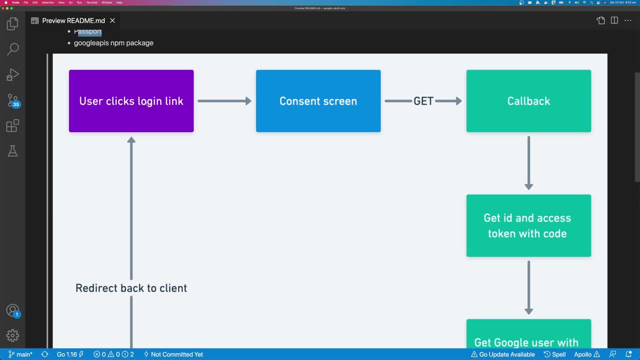 shows the flow that we're going to build. So the user is going to click a login link And when they click that login link, they're going to be sent to a consent screen and this consent screen is hosted by Google And once they give their consent for our application to have access, 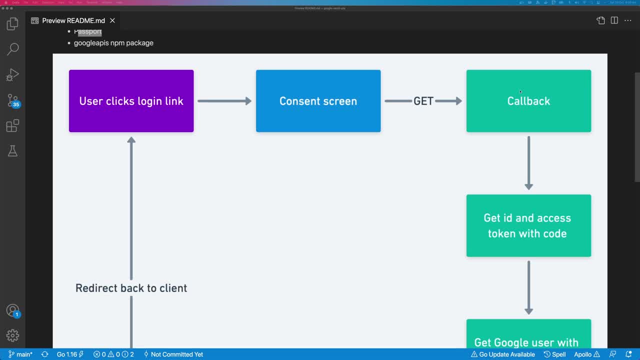 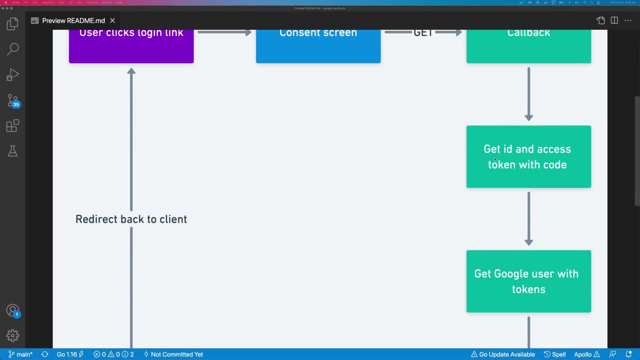 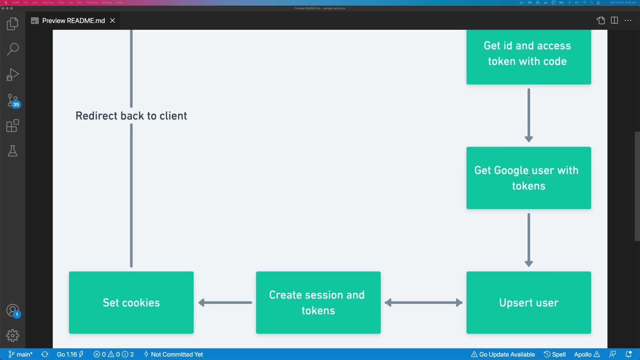 to their account. they're going to make a get request to our callback endpoint And this get request is going to include a code. So then our application is going to use that code to get an id and access token. Then we're going to use that id and access token to get the Google user. We're 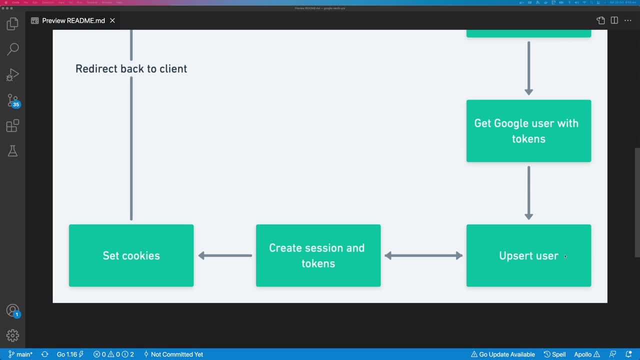 going to use that ID and access token to get the Google user. We're going to use that ID and access upsert the user into our database. so upsert means that we're going to try update the user and if they don't exist, we're going to create them. then we're going to create a session and 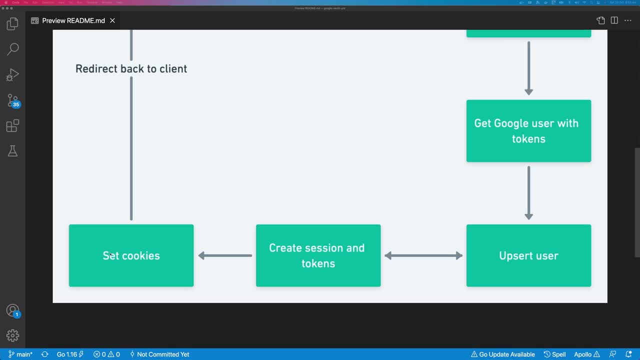 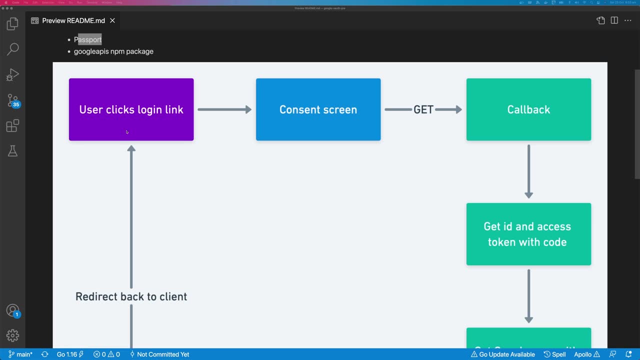 we're going to create access and refresh tokens, we're going to set some cookies for the user and then they're going to get redirected back to the user interface. so this tutorial follows on from a rest api tutorial that we've built earlier on. if you're coming from those tutorials, welcome back. 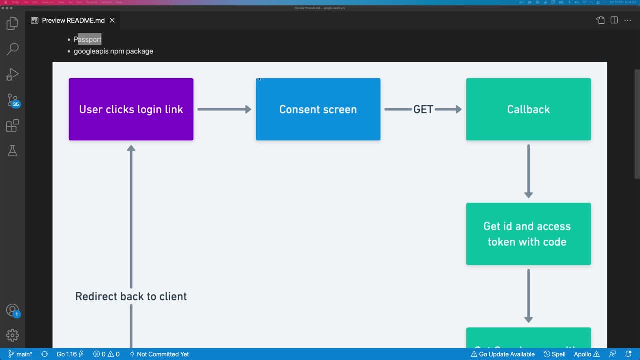 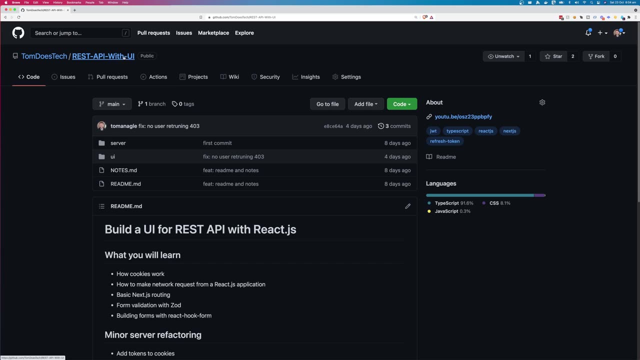 thank you for sticking with me, but if you haven't watched any of those tutorials, that's okay, you can still follow along. i'll give you a github repo to clone. so let's get started by cloning that repository. so i have this repository here and it's under tomdoztech rest api with user interface. 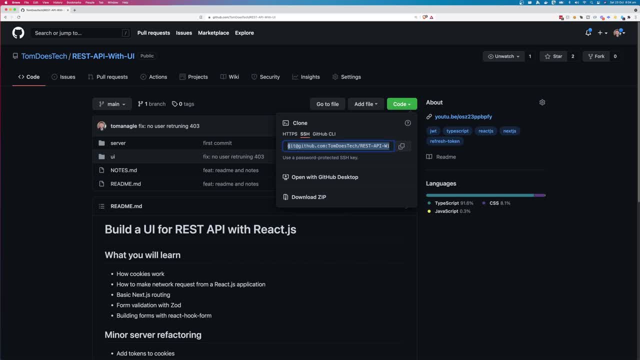 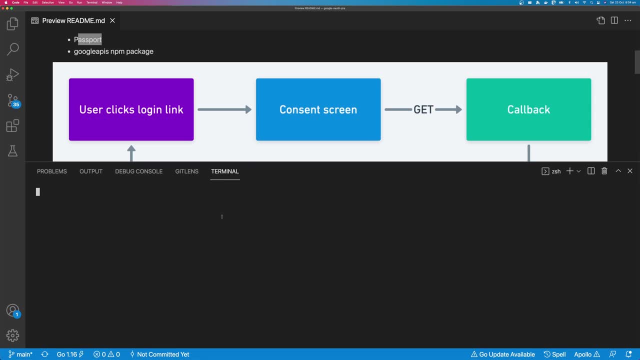 so i'm going to copy the ssh link here. you might want to use https, but i like to use ssh. i'm going to come back to vs code. i'm going to open a terminal and i'm going to type git clone and i'm going to clone this repository into a new folder called. 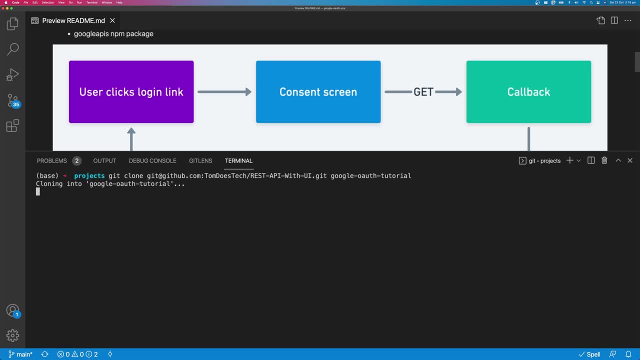 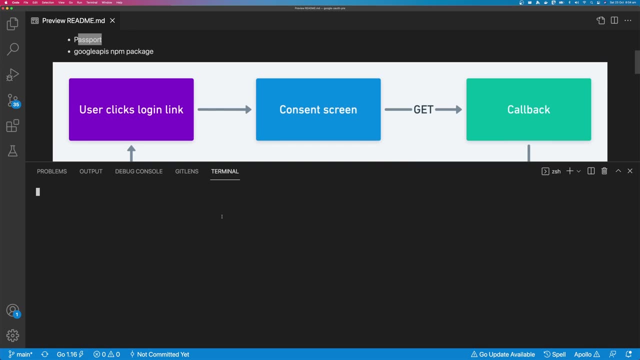 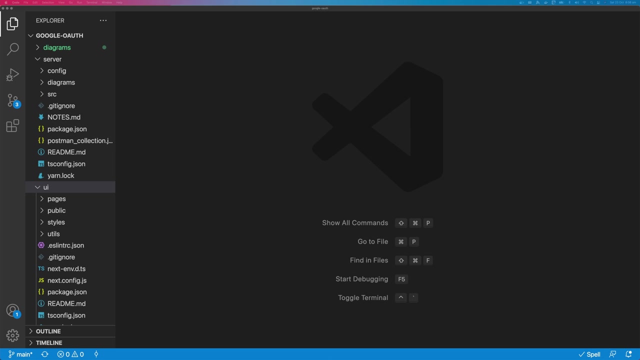 google oauth tutorial. once that repository has finished cloning, i'm going to cd into google oauth tutorial and i'm going to open this in a new vs code window. so we're going to go ahead and start the server. so to start the server you need to have a running. 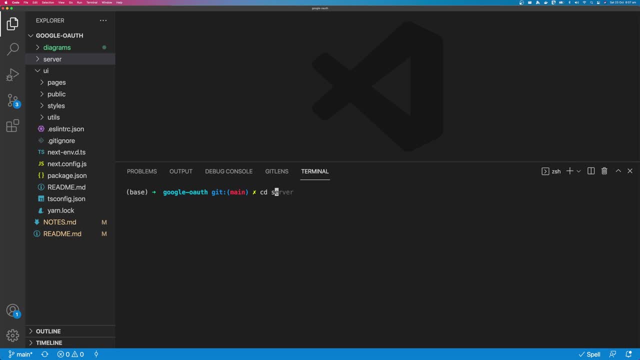 instance of mongodb, i'm going to cd into the server and i'm going to type yarn to install all the dependencies. and while they're installing i'll split my window here and i'll install the dependencies for the user interface as well. so cd into ui and we'll do the same command, just type yarn. or you could use npm install if you like. 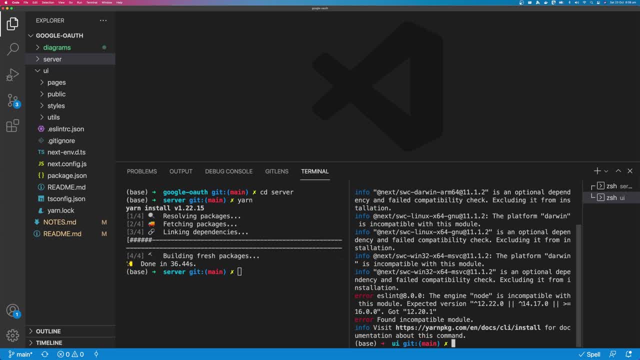 so the client expects a specific version of node to be installed. so it expects 12.22 or 14.17. i have this 14.17 installed with node version manager, so i'm going to type nvm, use 14.17.0. if you're not using node version manager, i highly recommend it. it is really easy for you to do that. 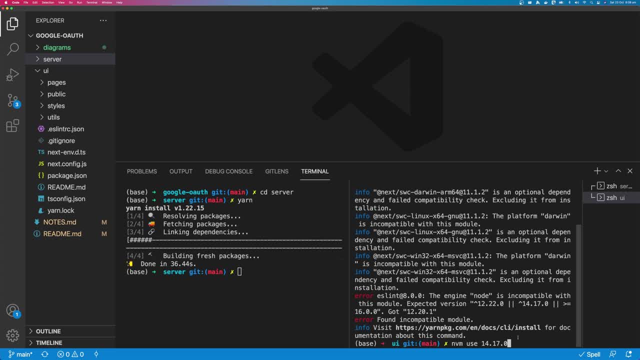 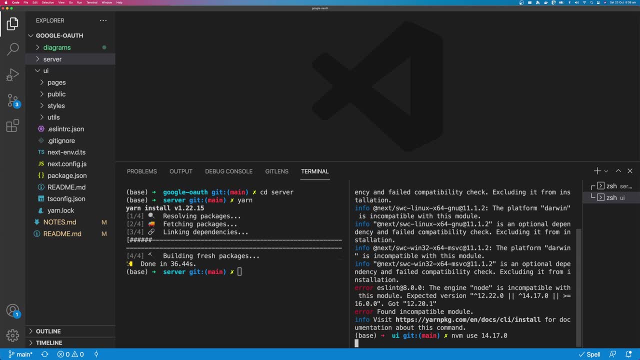 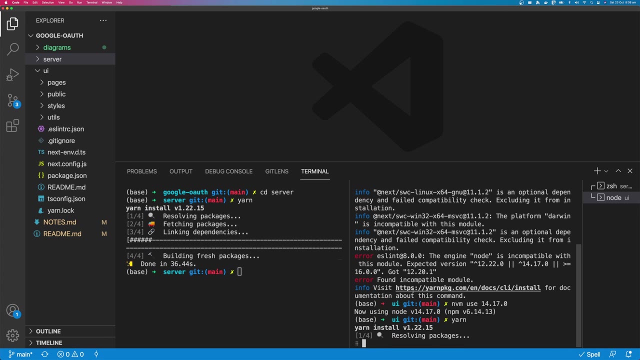 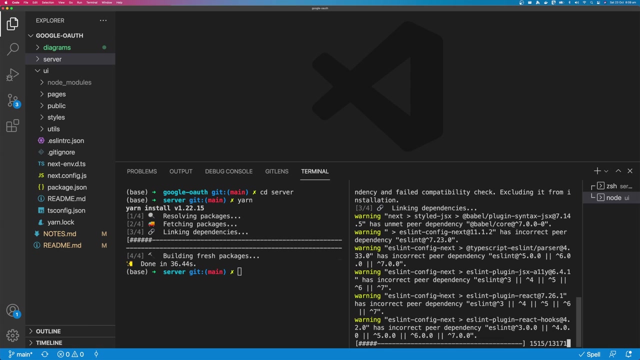 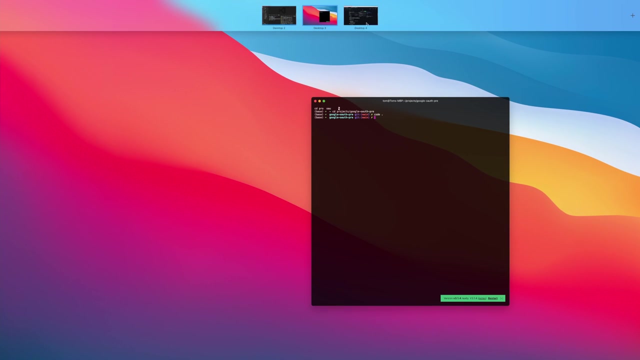 things like this. if you would like a tutorial on installing that with mac or windows, please let me know and you can see there. i've switched my node version, so i'm just going to type yarn again and these dependencies will install. so while these dependencies are installing, let's go get our google aworth credentials. 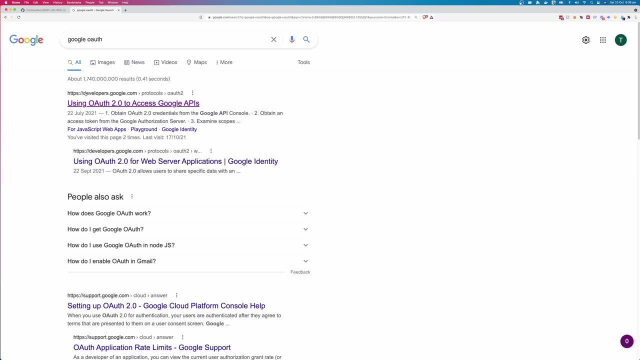 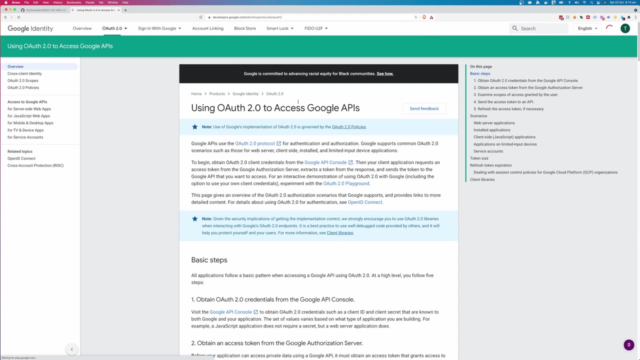 so i just come over to google and i just typed in google aworth and this first link here is some instructions on setting up a google aworth integration. so you can see, here this is about getting the access keys, so let's skip all this and the one. 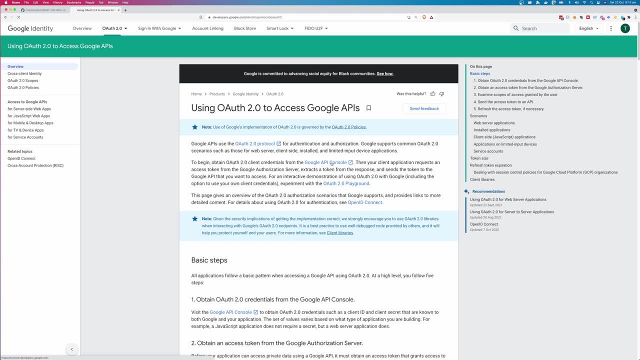 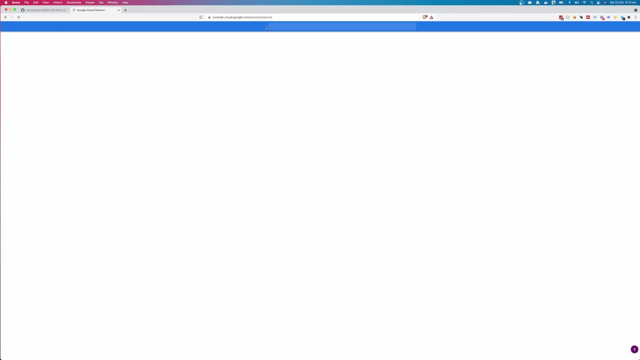 thing we need from this page is this google api console so we can click on that, and you need to have a google account, obviously. so i'm going to give you a warning about this console page. it is a little bit complicated, pretty annoying, it often doesn't work and stuff is all over the place, but it's better than. 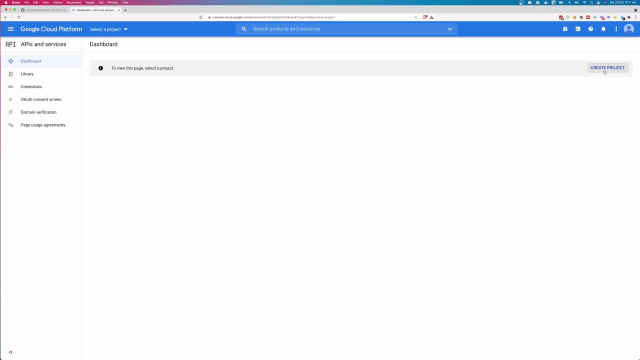 other providers, such as azure. so i'm going to click create project and i'm going to call my project google aworth, and i'm not going to have an organization. i'll explain a little bit about what organizations do in a minute. but if you're creating a public, 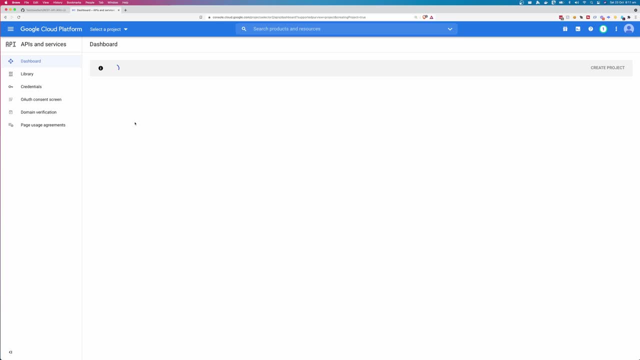 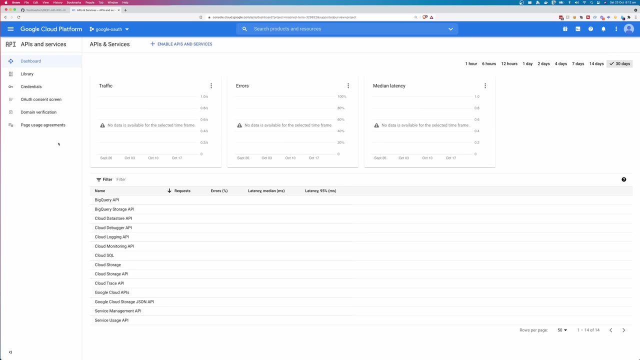 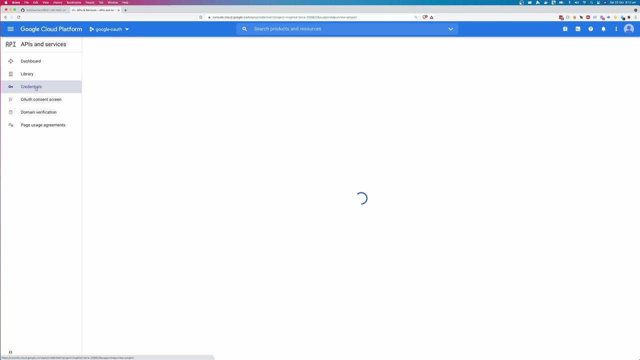 facing application, you don't need to have an organization. so my project has created here and so i'm going to come down to credentials and you can see up here we can create some credentials and they will go down in this aworth to client id section. but before we can create credentials we need to create a consent. 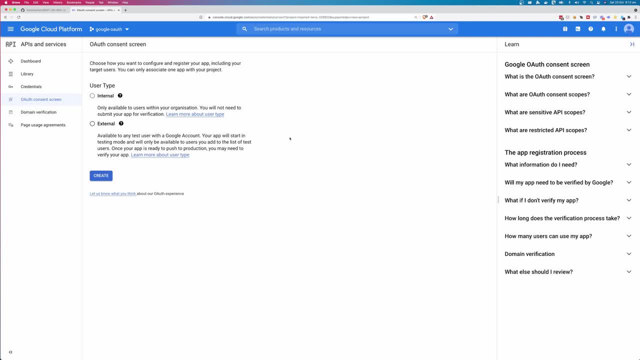 screen and the consent screen, if you remember from that diagram, is where the user will get redirected to after they click the link on your website. so we want to choose the user type. so internal means that only users within the organization that you selected will be able to get access. 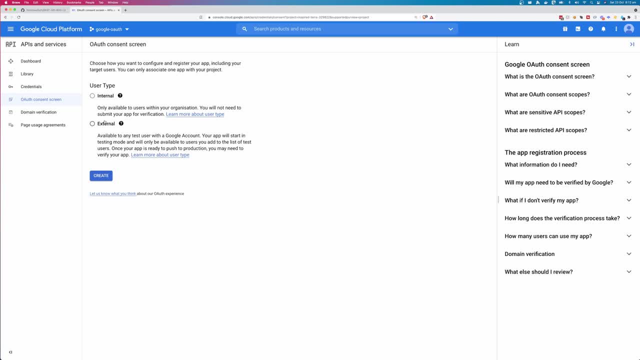 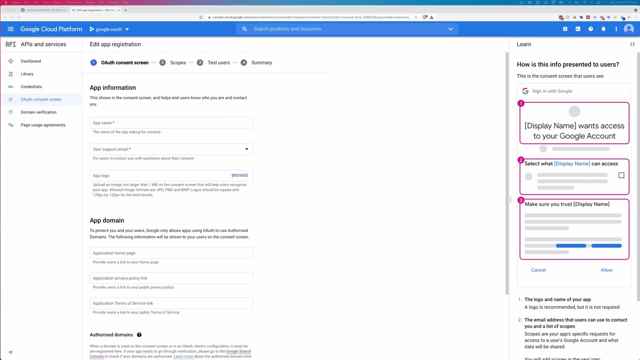 to this application and be able to log into your application. if you want to make a publicly facing application, which i assume you do, you need to create an external integration. so click create and i'm going to give my application a name. so i'm just going to call this google or tutorial. 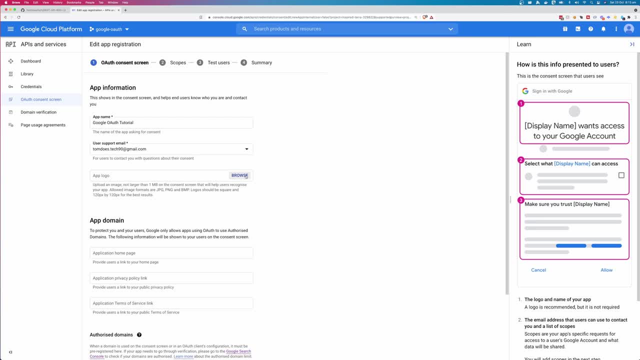 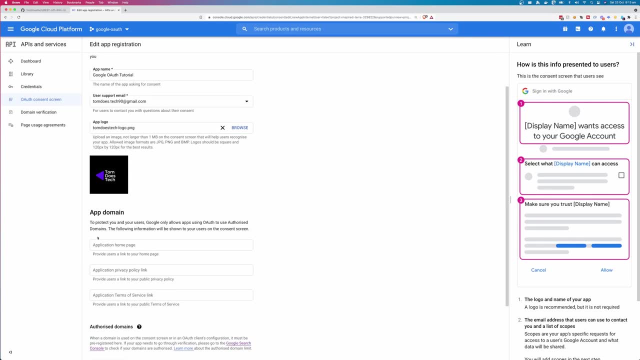 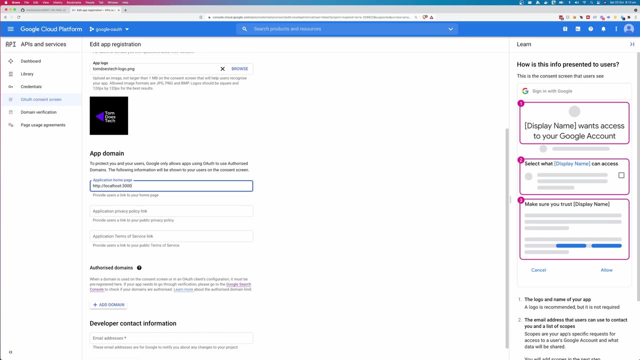 the user support email is just going to be your email address. you need to upload a logo. so i have this expertly designed logo here. application home page. so i'm just going to put in my local host address. i'm going to do localhost port 3000 and this is the port that our client. 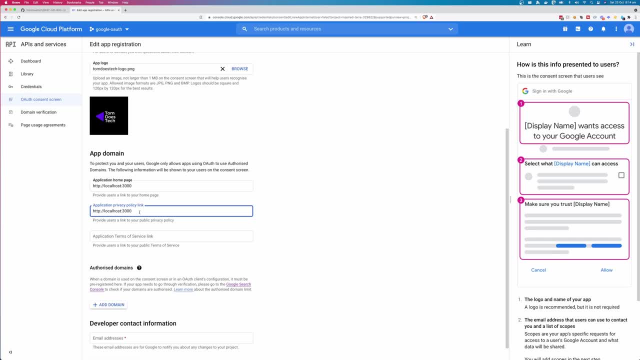 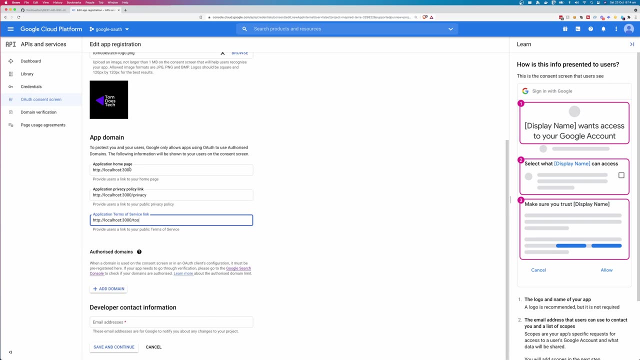 will start on. so for our privacy policy link, i'm just going to say localhost, port 3000, slash privacy, and for terms of service, i'm just going to do the same, but i'm going to call this tos, so we don't need to add any authorized domains. and for the developer contact information, we're going to do. 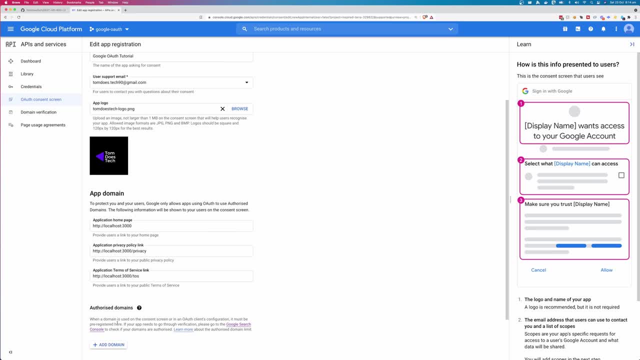 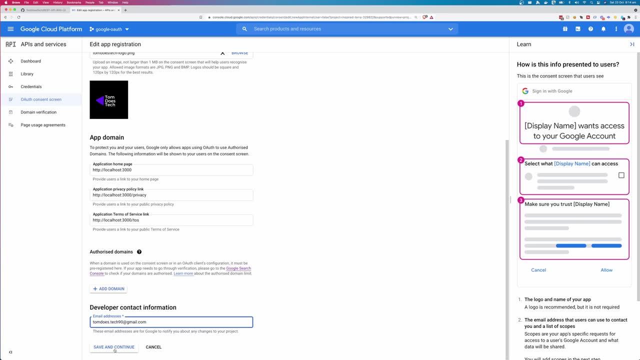 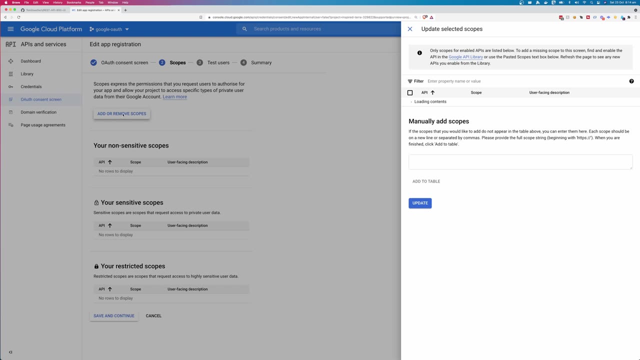 So I'm going to create my own domain contact information. I'm just going to use the same email address, TomDarzTech90 at emailcom. Please don't send emails to this email address, because I never look at it. Okay, so we need to add some scopes. So there's lots and lots of different scopes that you can. 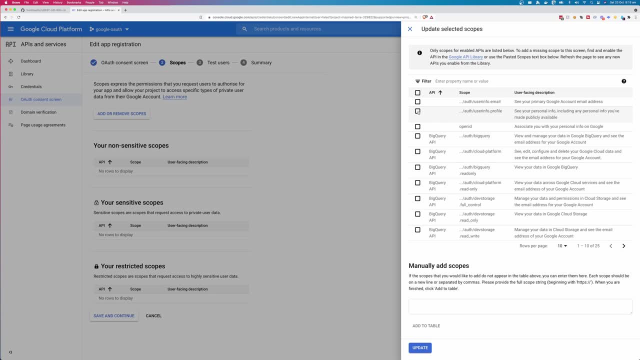 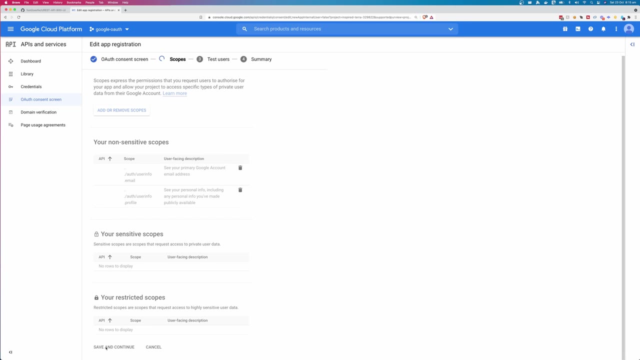 add to your application, But the only ones that we need now are going to be this: or slash userinfoprofile and userinfoemail. So let's update that And let's click save and continue. Add a test user. So this is a user that will be able to. 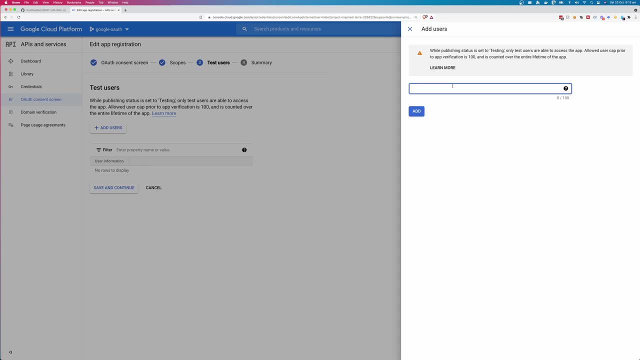 log into your application while it's still in sandbox mode. So this is quite important. So I'm going to add my email address, TomDarzTech90 at email, And this means that you can test your application without bringing it out of sandbox mode. 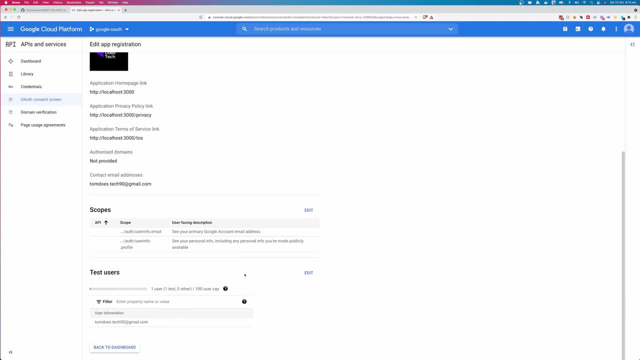 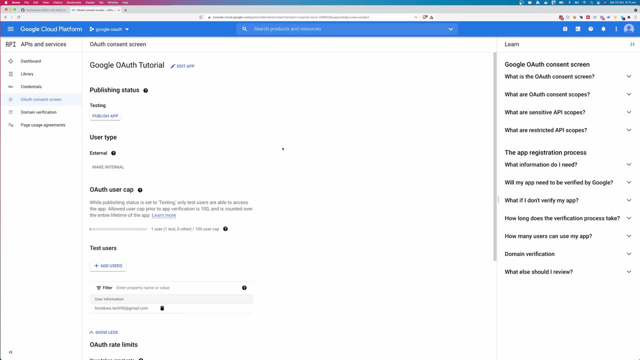 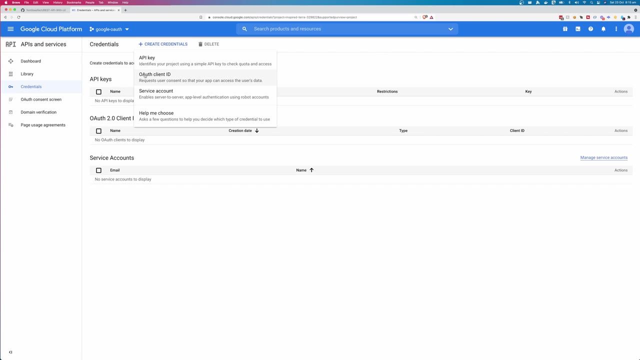 I'm going to click save and continue And let's go back to our dashboard. So now we have our consent screen configured, We can go back to credentials And I'm going to click create credentials. And we want to create an OAuth client ID. 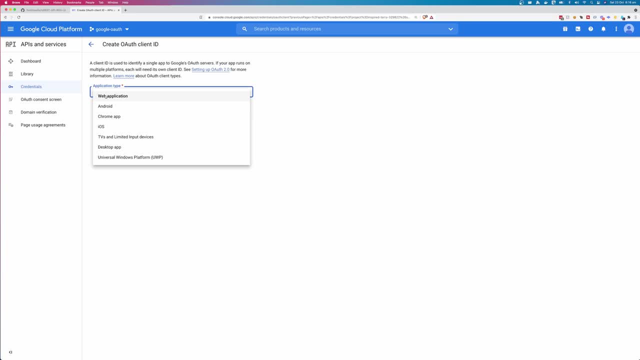 So the application type is going to be a web application. I'm just going to call mine Google OAuth tutorial threads And we need to add an authorized redirect URL. So I'm going to say HTTP colon, colon, colon, slash, slash, local host and port one through three, seven, because this is our server. 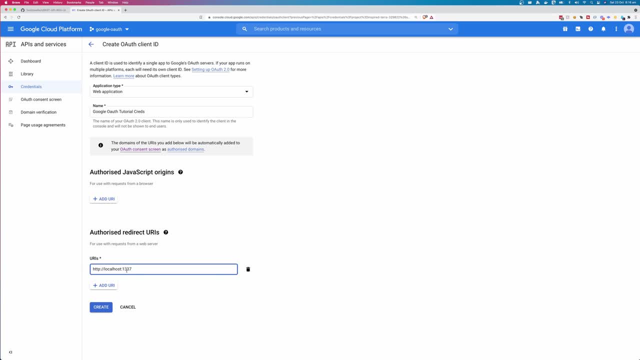 different ways you can do this. you can redirect back to your client and from your client make another request from the server. but i find it easier to make this: get request straight from the consent screen. it works out a little bit quicker. so the redirect url is going to be the. 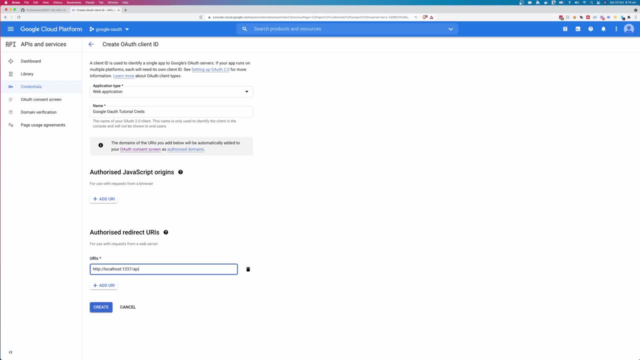 service address: slash api, slash sessions, slash oauth, slash google. so you can make this path whatever you like. obviously you can make it google redirect, uri. but i think this path makes sense because we're going to create a session, we're going to do that with oauth and then here, 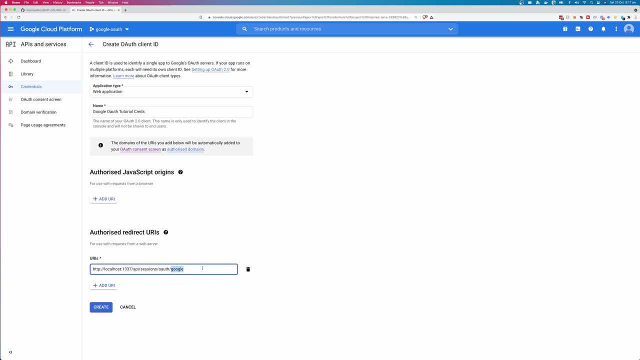 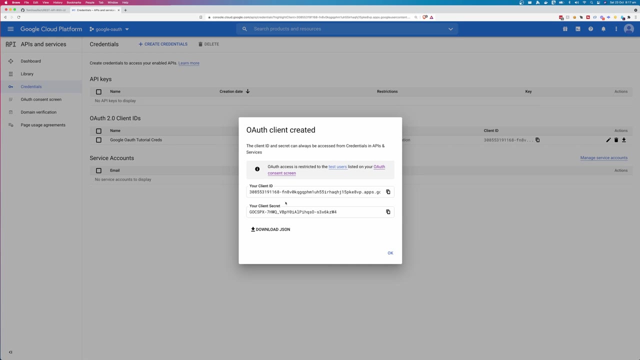 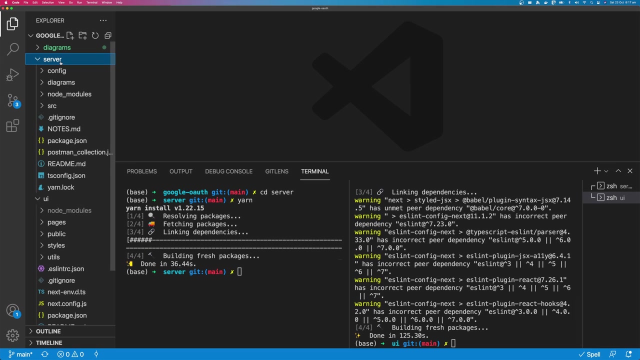 we have the provider. if you have multiple providers, such as azure, you might then want to have a redirect url that is azure, but we're going to make this one slash google. so click, create, and here we have a client id and a client secret. so i'm going to copy this client id and i'm going to come over to the server. 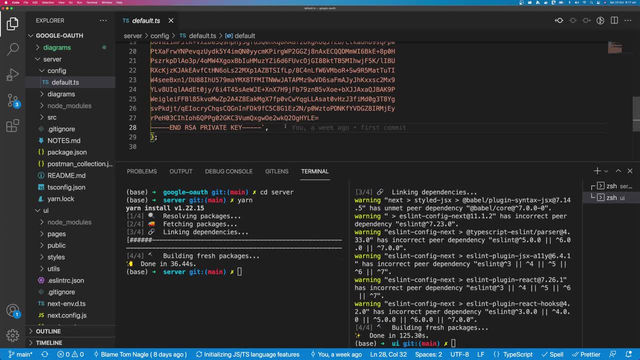 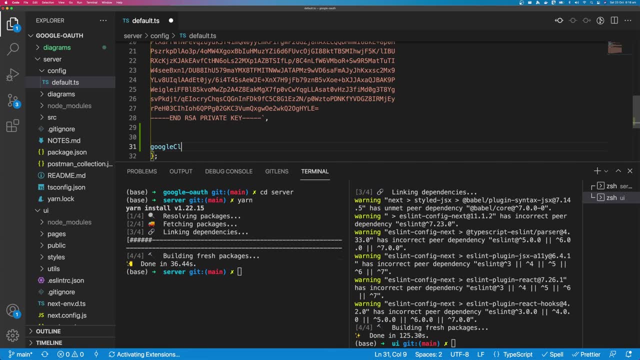 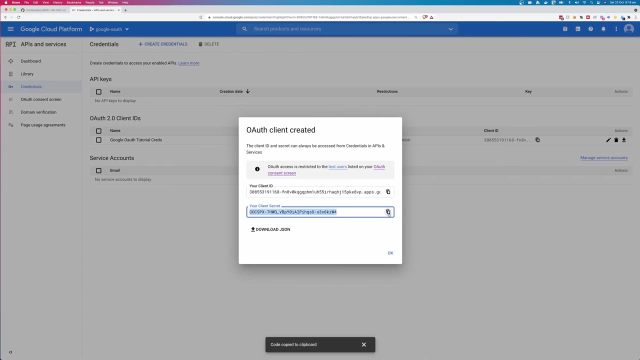 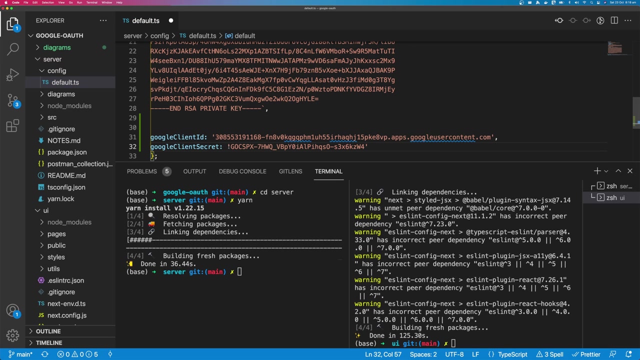 and in the config i'm going to add this client id, so i'm going to call this google client id and then i'm going to do the same with the secret. so this secret is obviously a secret. you do not want to show everybody this, like making a youtube. 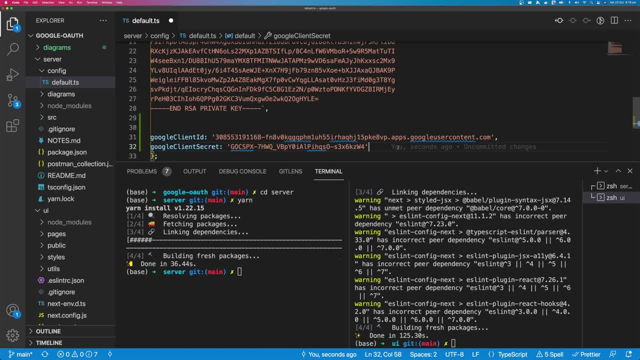 tutorial where you display this publicly is probably a really bad idea. so if you're going to commit this package, you don't want to just hard code this into your config file and then send it up to your source control, such as github. you'll want to put this in an environment variable. 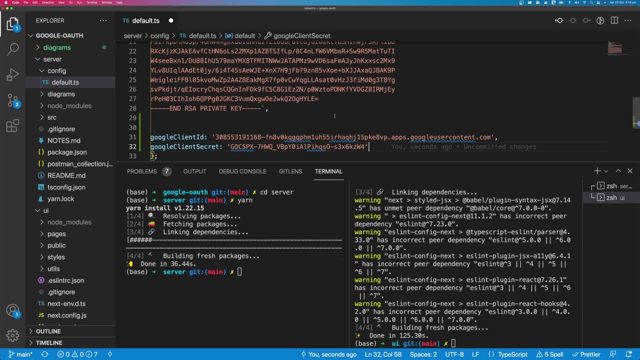 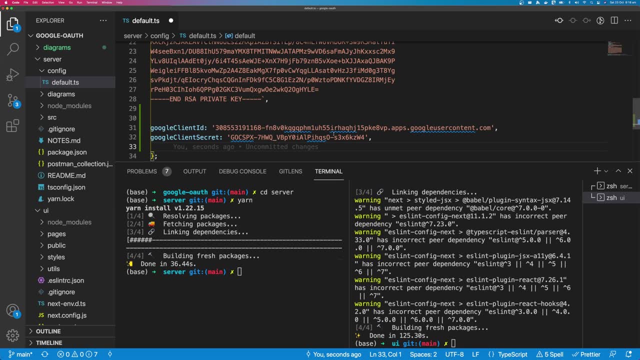 and store it only locally. but i'm going to delete this application and then i'm going to create a new one after i finish making this tutorial, and so you won't be able to use this secret. so in here i'm going to also make a google aworth redirect url, so i'm going to say google. 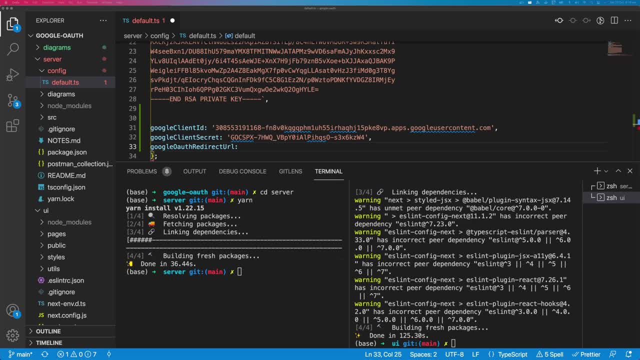 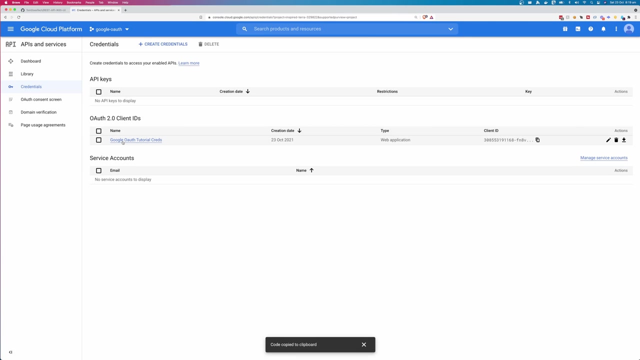 aworth redirect url. i'm going to make the value of this aworth redirect url the same as we did when we created the credentials, let's say http, localhost, 1, 3, 3, and actually it's probably better if we come back into our client ids and we just copy it from here. that's going to be much more reliable. 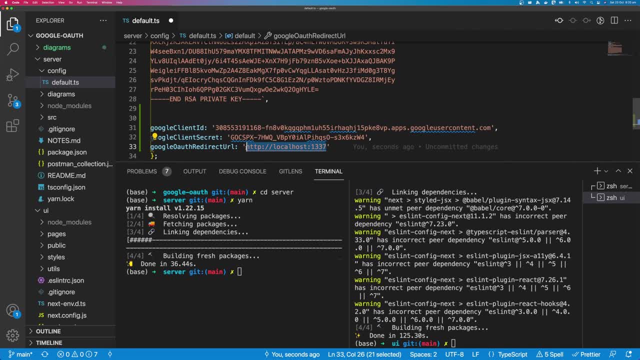 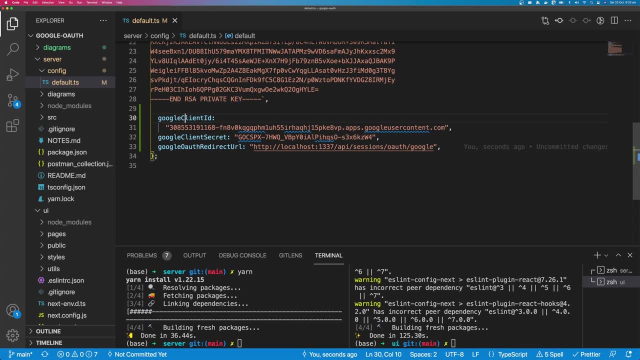 let's grab this and i'm going to paste it in here. so now we have these credentials set up on the server. on the client, we just need to add the client id. so you obviously don't want to put this client secret into your client application, So we're using Nextjs. So I'm going to create an environment variables file. 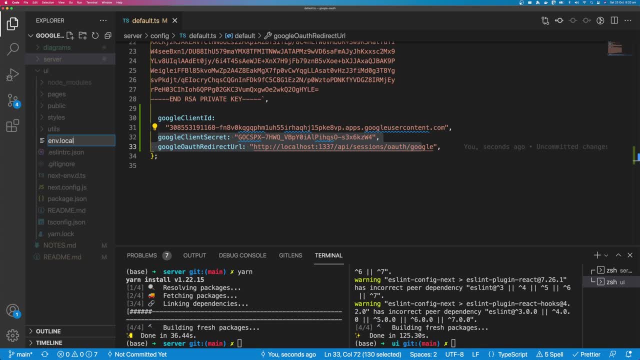 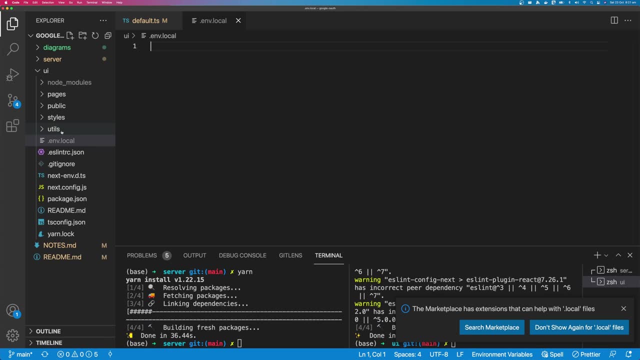 called nvlocal. This is supposed to be nvlocal. So in here we're using Nextjs. So this is just going to work out of the box and we need to prefix public environment variables with next public. So I'm going to say next public underscore. I'm going to copy that three times because we need. 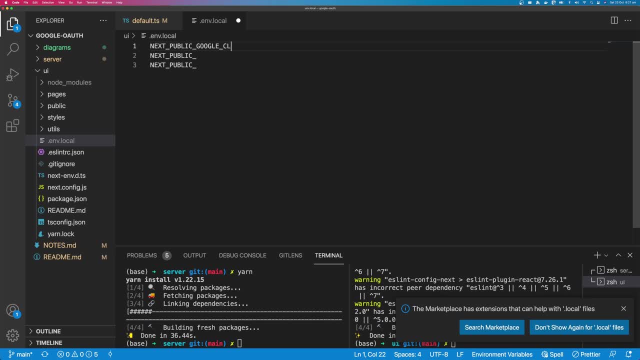 three of these. I say Google client ID equals. The next one we need is a server endpoint. Server endpoint equals And we need the Google OAuth redirect URL. So I'm going to say Google OAuth redirect URL equals. So this Google OAuth redirect URL is the same as we put in when we 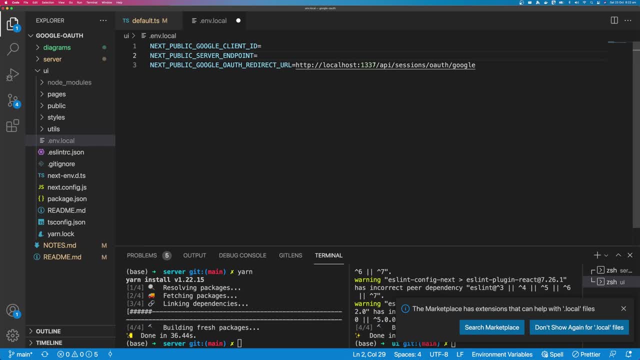 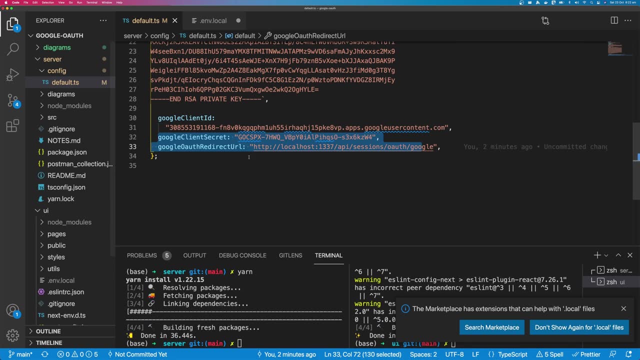 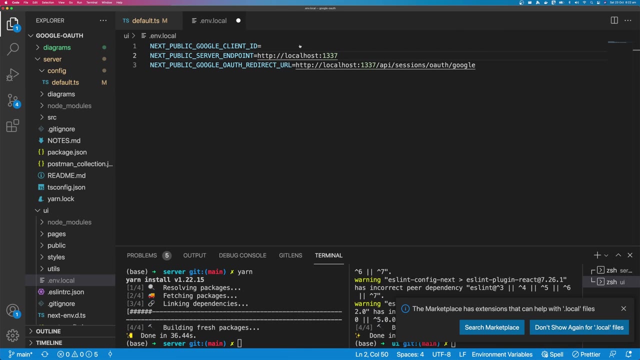 created the credentials. The server endpoint is just going to be this portion of the URL, And then we can get the client ID from our server, So it's going to be this long string here. Okay, great, So that is all of our credentials that we require, So I'm going to start the server. 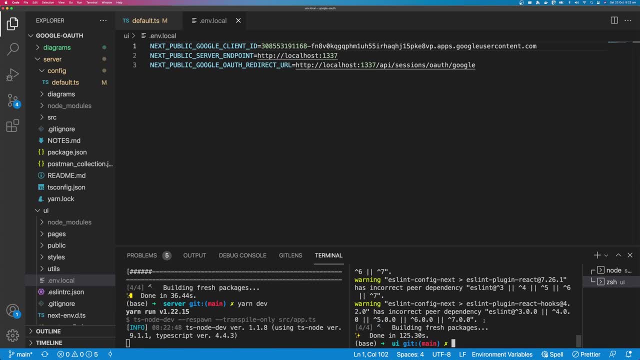 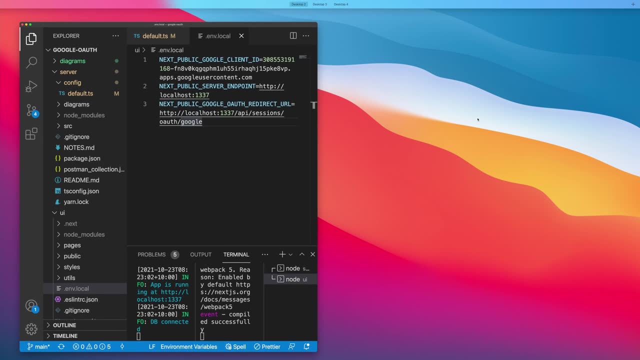 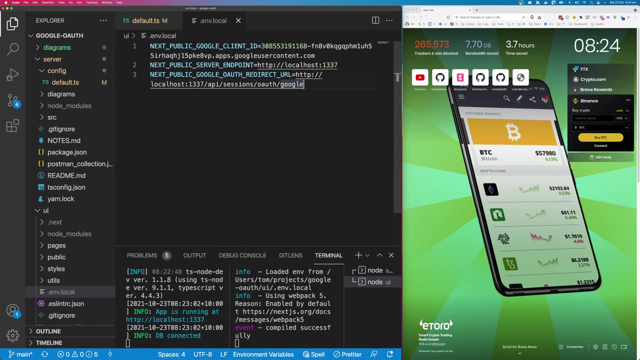 with YarnDev And I can start the client with YarnDev also. So I'm going to split my window here and put a browser on the right here so we can see what we're working with. So in the browser I'm going to go to localhost port 3000. 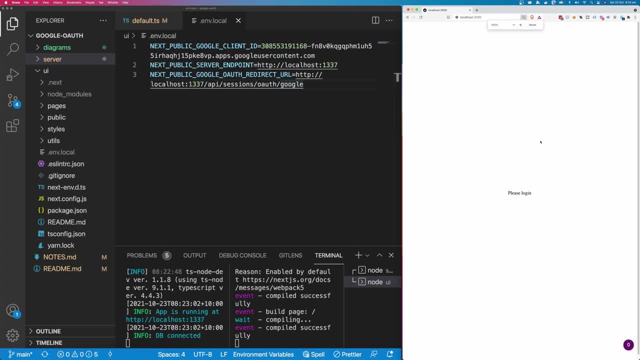 And you can see in our client, we just have this: please log in text here. So we need to put a link on this page that goes to the consent screen. So we need to build that link based off our client ID and a bunch of scopes and stuff like that. So I'm going to show you how to make a function. 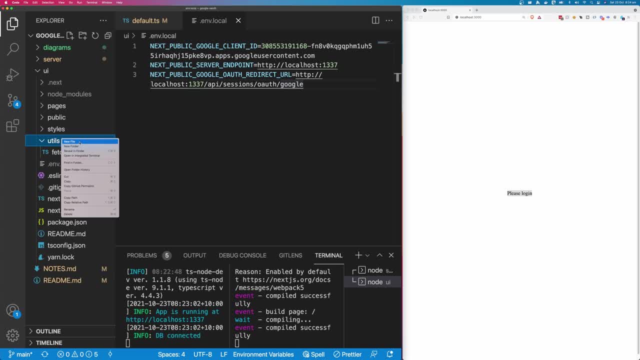 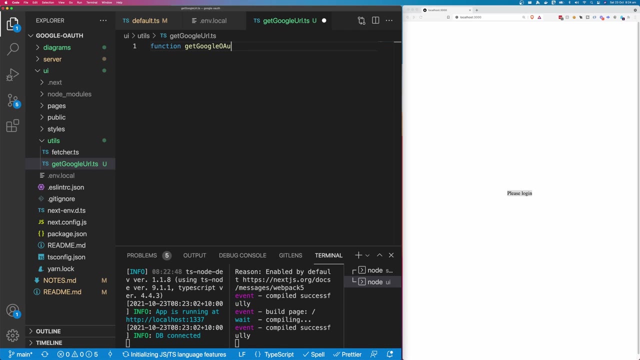 to build this link. So in the utils let's create a new file called get Google urlts And I'm going to say function: get Google oauth url. And I'm just going to export defaults: Get Google oauth url. So let's define the root URL. So I'm going to say const root URL. 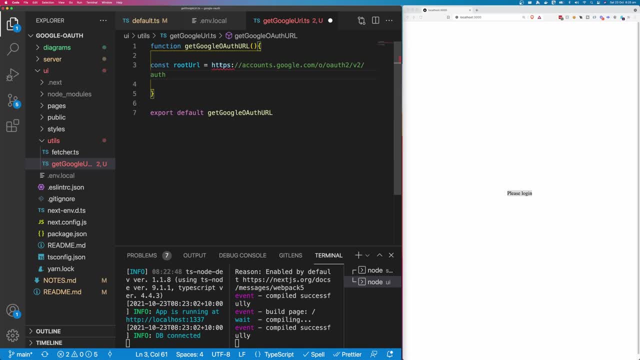 url equals And this is going to be HTTPS accountsgooglecom. slash o, slash oauth2 version two, slash auth, And let's define some options. So I'm going to say const options is equal to, and options is going to be an object. Let's define our URL search params. So what we're doing here. 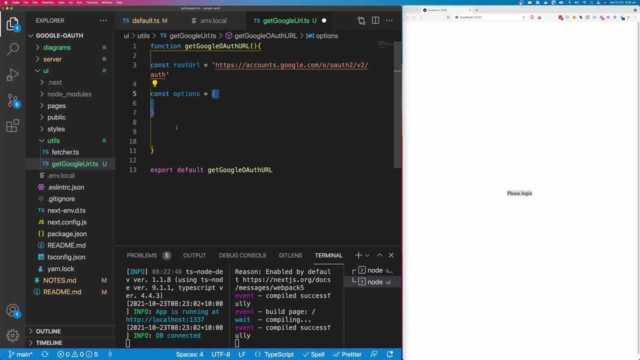 is, we're defining some options in an object And then we're going to add those options to a query string. So we need a way to build that query string. So I'm going to say const qs. So you used to be able to just import query string from query string. 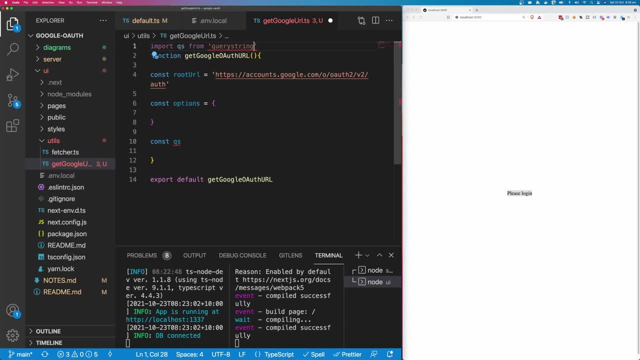 like this, But this is deprecated And we're going to use url search params instead, So we don't need to import that. So I'm going to say const qs equals new URL search params And we're going to pass in our options. 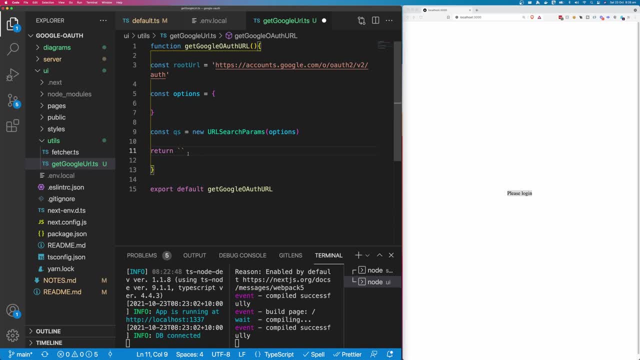 Then I'm going to return And I'm going to use our templating strings. I'm going to start off with the root URL And then I'm going to put a question mark because we're going to have some query strings here, And then I'm going to put in another template here. 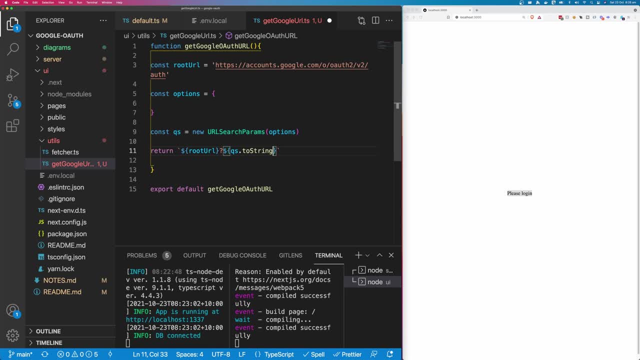 And I'm going to say qstoString And then I'm going to execute that. So let's start defining our options. So I'm going to say redirect URI is going to be processenv And we get this from this next public Google OAuth redirect URI. 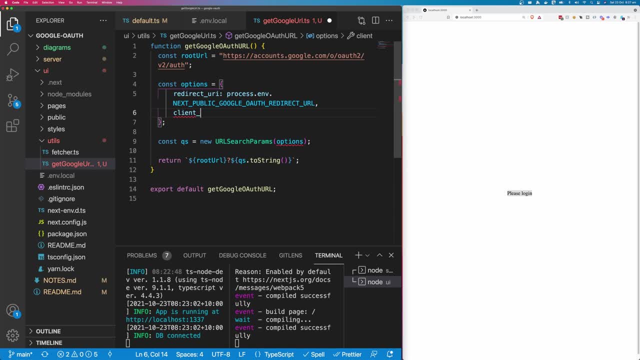 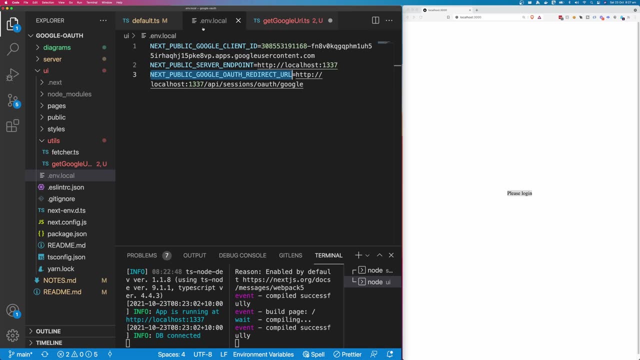 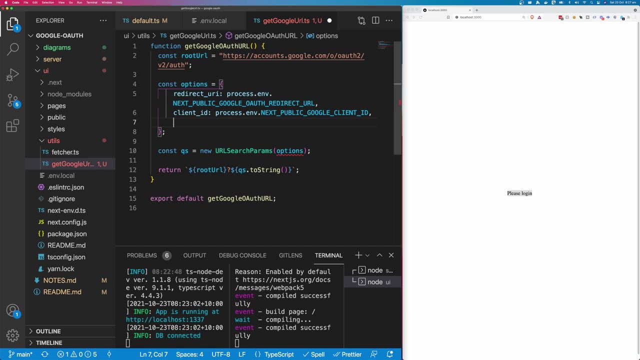 I'm going to pop that in there And say client Id is going to be processenv And we're going to get this from next public Google client ID. I'll say access type is going to be offline, Response type is going to be code. 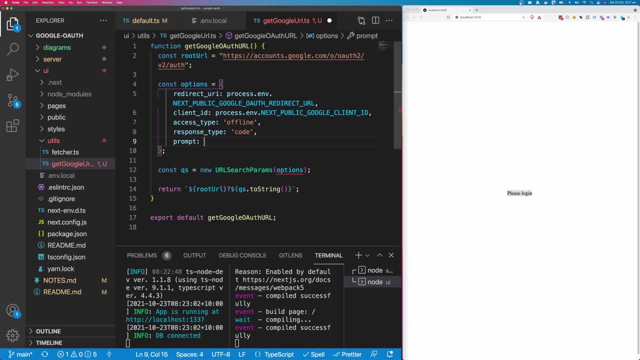 Prompt Compt is going to be consent and scopes is going to be an array, And these are the scopes we defined when we created our consent screen. So the first scope is going to be user info- dot profile, And then the second scope is going to be user info- dot email. 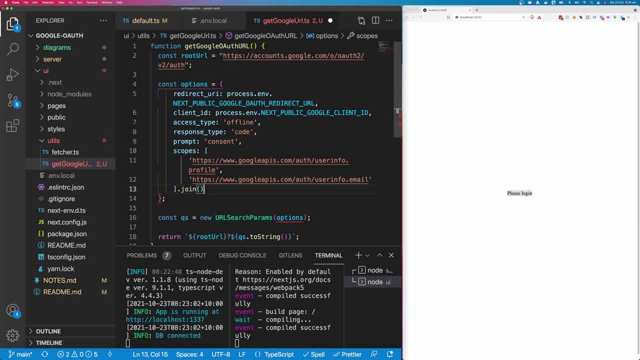 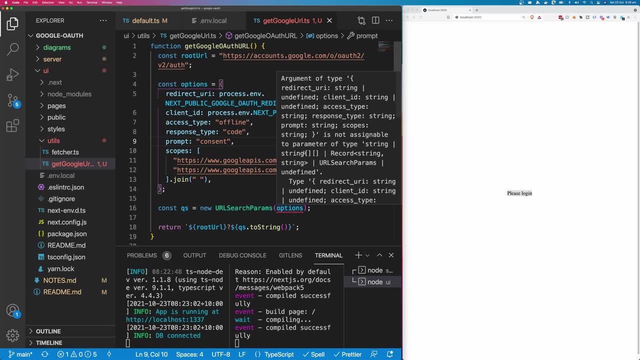 So we need to join these scopes. So let's call it dot join And we're just going to join these with a space. So TypeScript is complaining here, saying that client ID needs to be a string. So we know that client ID is going to be a string, but it says here that it's going to 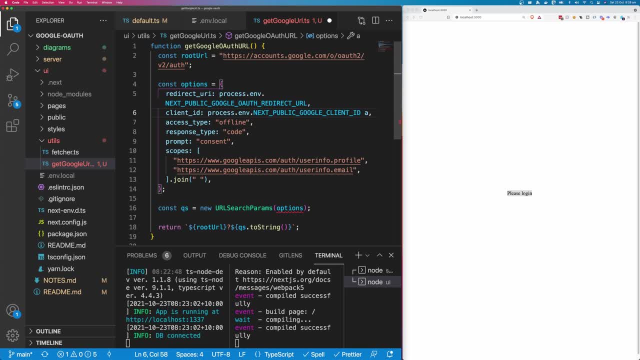 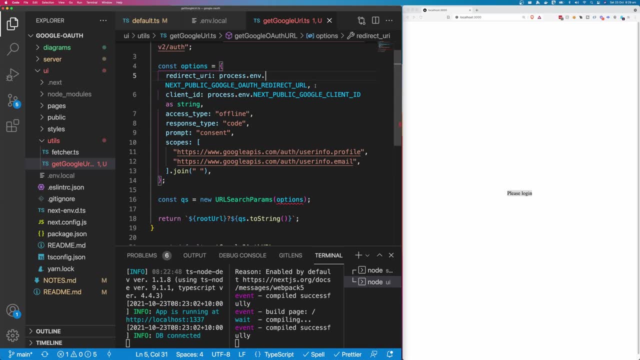 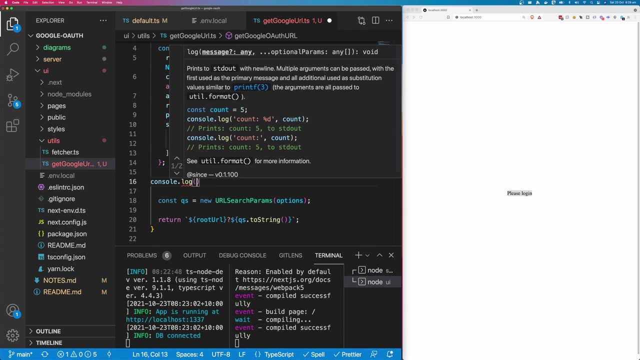 be string or undefined. So let's just say as string. And we need to do the same for redirect URL. So I'm going to say as string And TypeScript is now happy. So let's add a console log for these options. console dot log options. 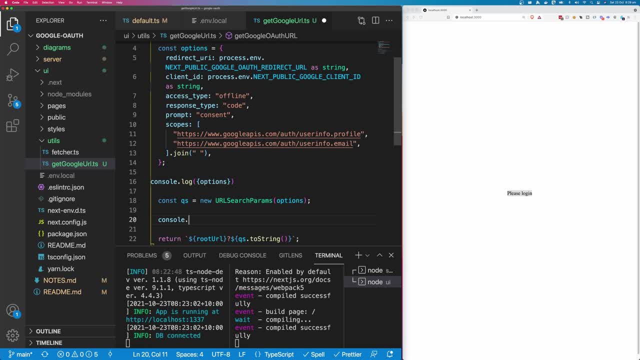 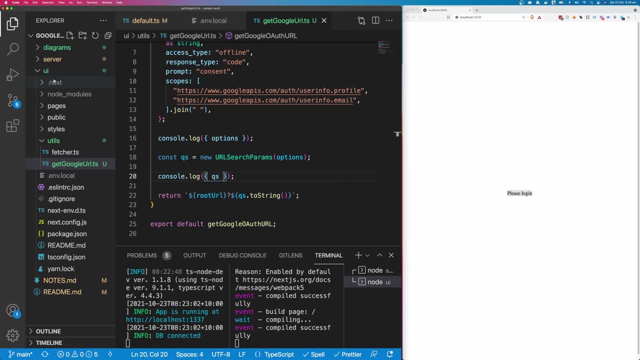 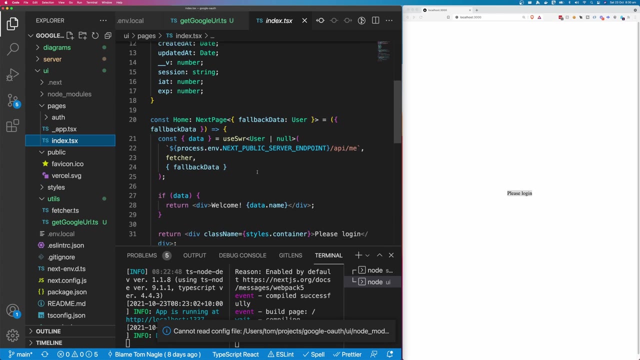 And let's add another one for this QS constants console dot log, And I'm just doing this so you can see what this looks like. And let's go to consolelog And I'm going to add a link to our index page. 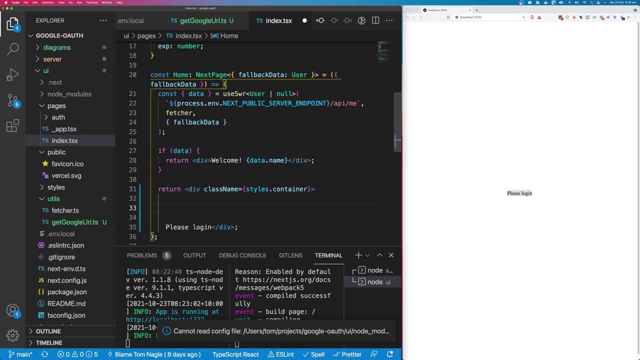 And where it says: please log in. I'm going to add a link, I'm just going to use an anchor tag And the href is going to be equal to our get Google OAuth URL, And we're just going to execute that function. 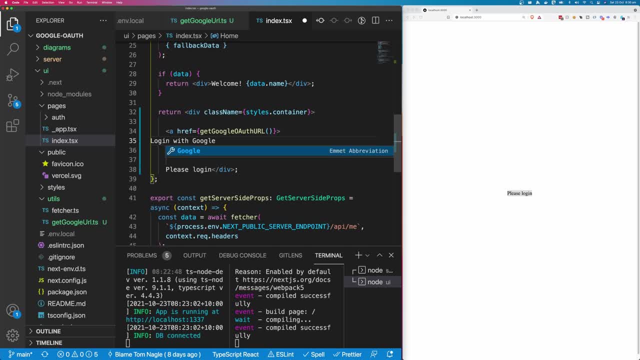 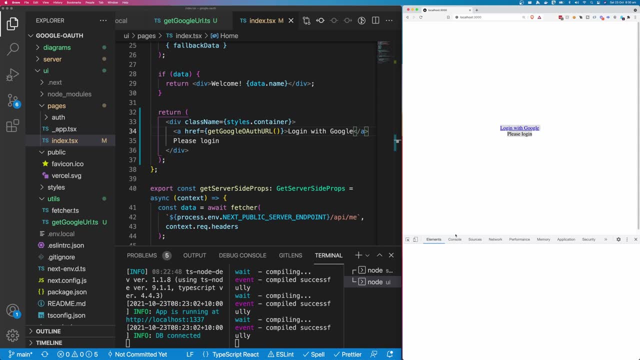 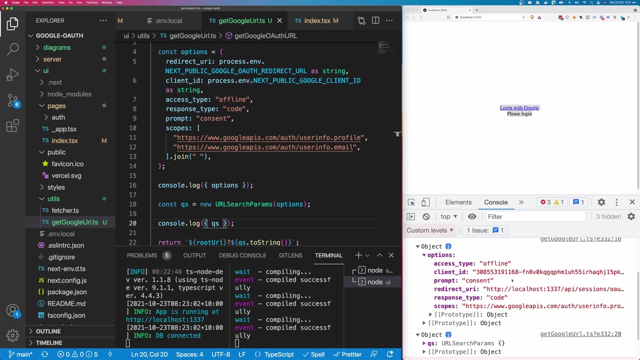 And I'm going to say log in with Google. Let's open up our console so we can see those parameters inside the get URL function. You can see, here we have our options. Let's compare that to this, And so our client ID has been successfully inserted and same as our redirect URL. 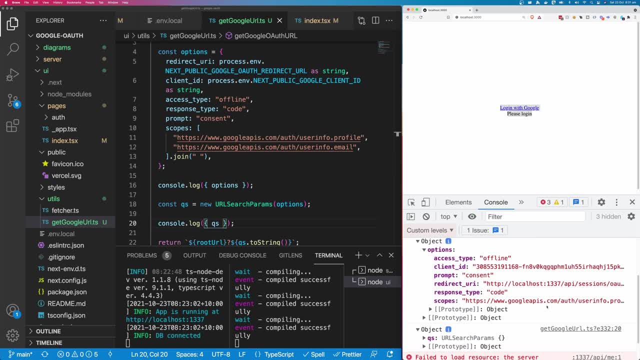 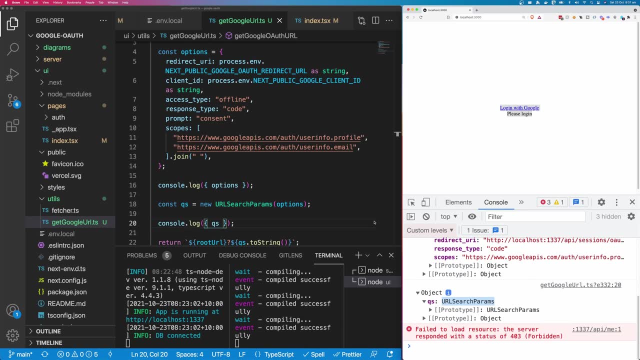 And we have all these scopes and you can see here that these scopes have been joined. Let's have a look at our query string And You can see it's just a URL search parameters constructor. Let's call dot to string on that here so we can see what it actually looks like in the URL. 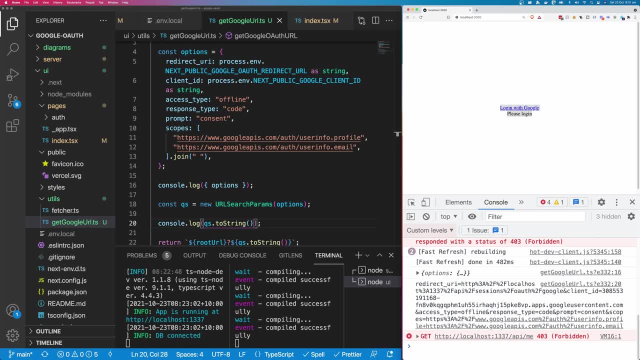 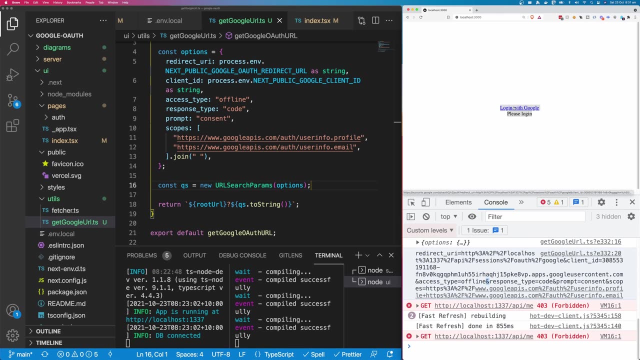 And you can see here that it combines all of these options and it separates them with an and symbol. Let's remove these console logs And I'm going to click this log in link And it should take us to a Google OAuth login page. 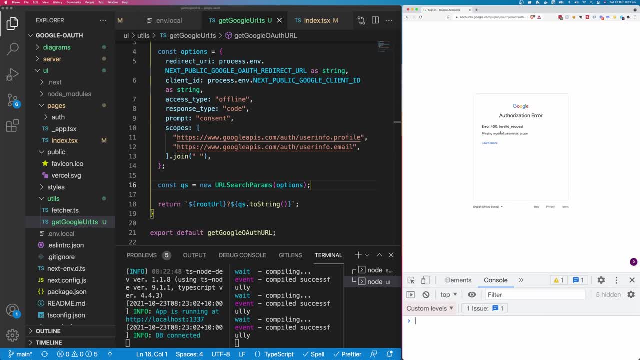 Let's click this And so we have an error here, missing required parameter scope. So the reason for that is because we've called this scopes instead of scope. So I've made this integration now probably 10 times in my career and I've never got this right the first time. 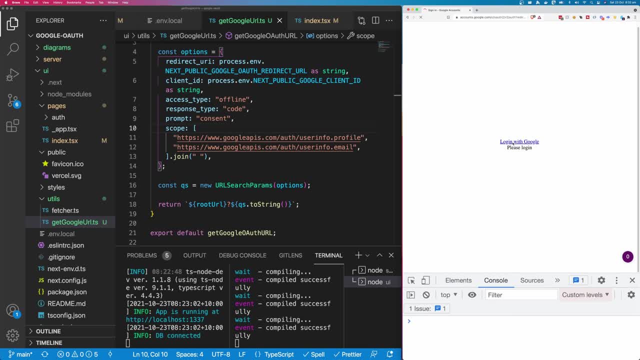 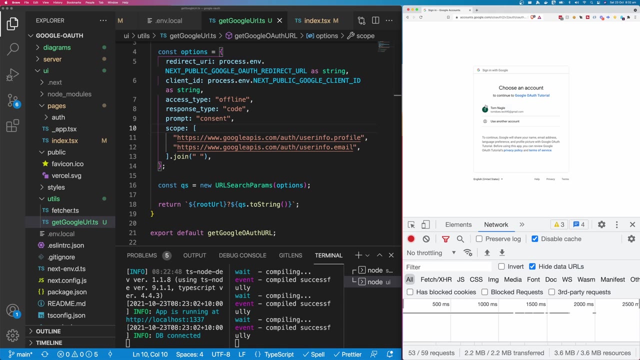 Let's try this log in link again. And here we go. We can log in with our Google OAuth account. So let's click this thing here And see what happens. So I've opened up the network panel And I've removed my filters. 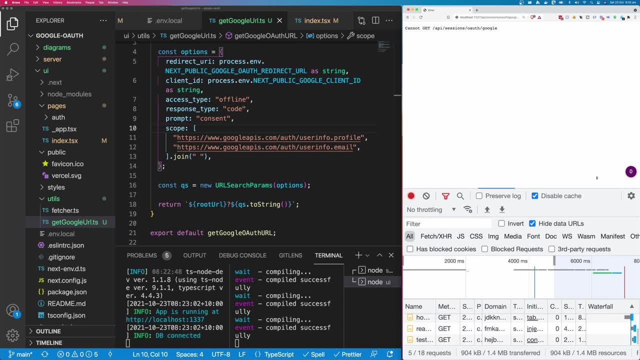 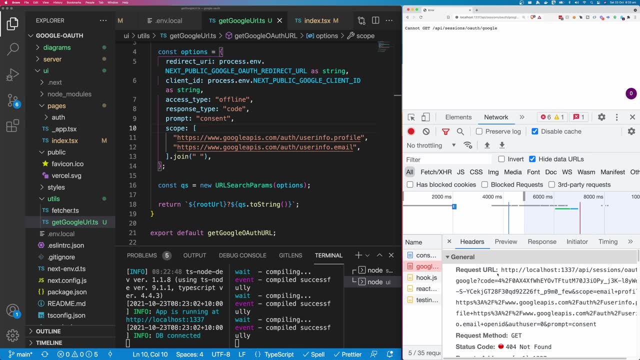 So I'm going to click this link And you can see we have returned a 404.. And we've made this request down here And this is a get request to localhost port 1337 slash API. And the interesting thing about this is we have this code on the query string: 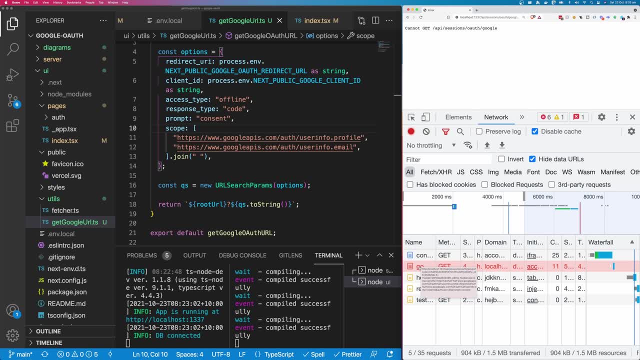 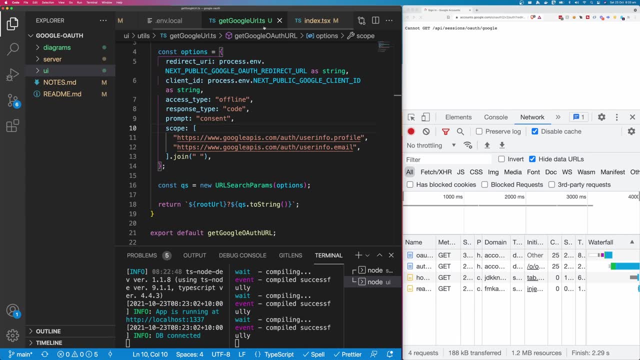 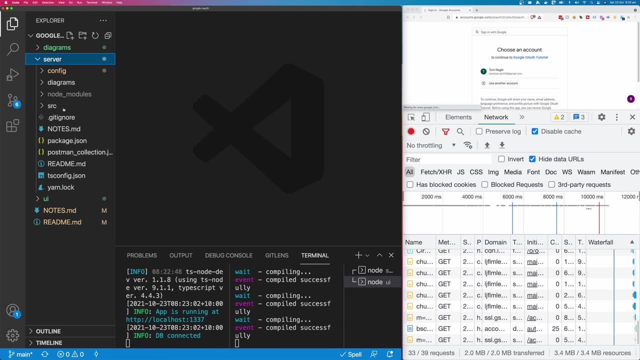 The reason this is returning a 404 is because we obviously haven't created this endpoint, So let's go do that now. So I'm going to close out all my UI, because we're finished with this for now, And come into server And I'm going to open up source. 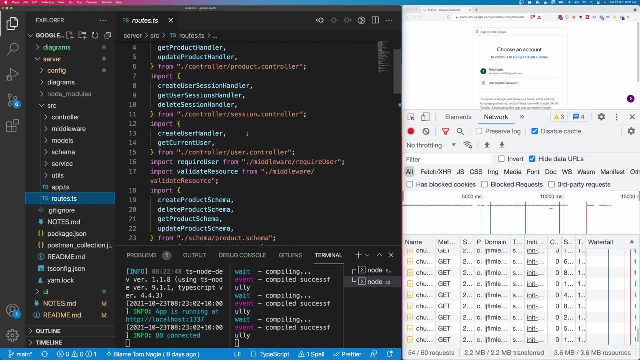 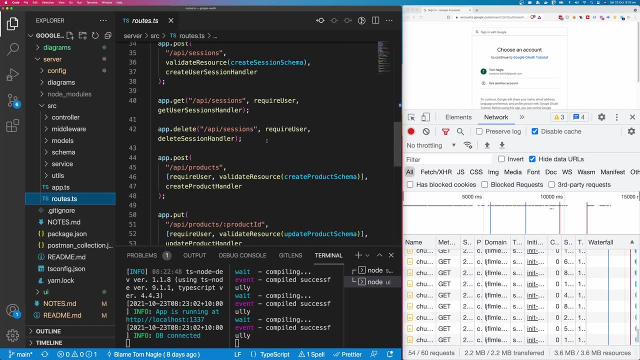 And I'm going to open up routes And I'm going to define a new route And this route needs to match that get request. So I'm going to say: appget Slash API, Slash sessions, Slash OAuth, Slash Google, And we don't want any middleware on this request. 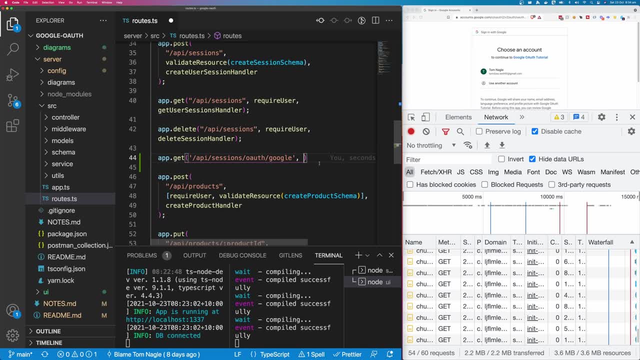 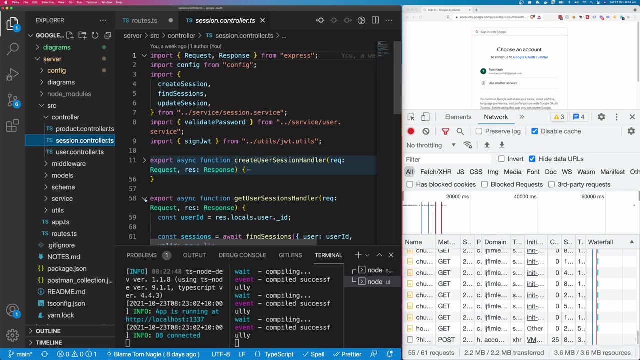 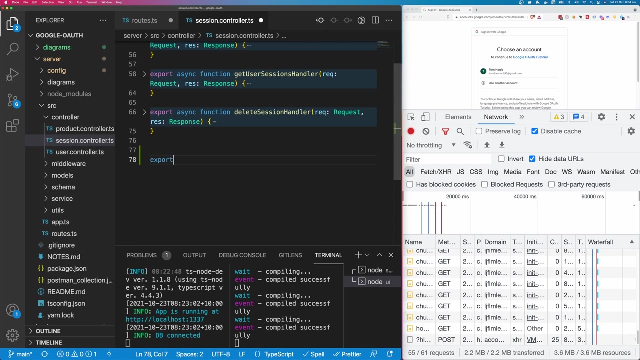 So we want to create a handler that says Google OAuth handler. So let's go create this handler, And I'm going to create this inside of my sessions controller. I'm going to collapse all of this And I'm going to say: export async function. 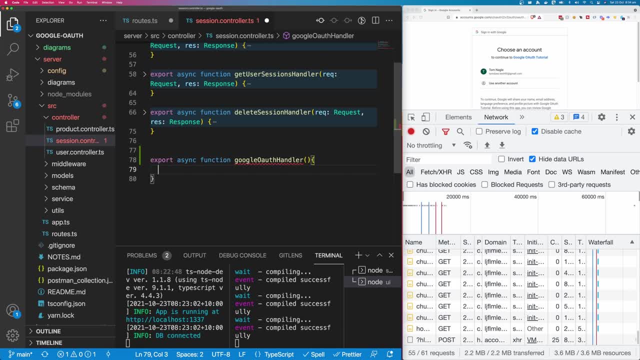 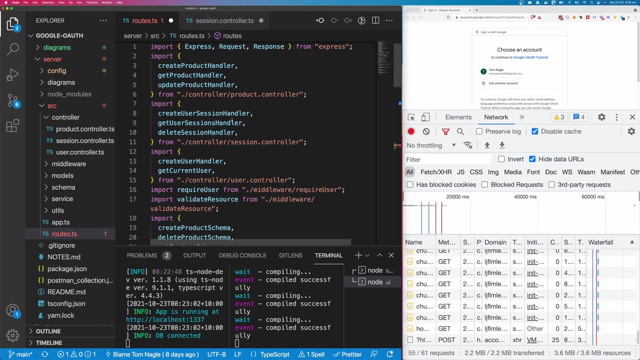 Google OAuth handler And we have a request and response here, So I'm going to copy that from above. So I'm going to import this handler inside of the routes And this comes from the session controller. So I'm going to import it here from controllers- sessioncontroller. 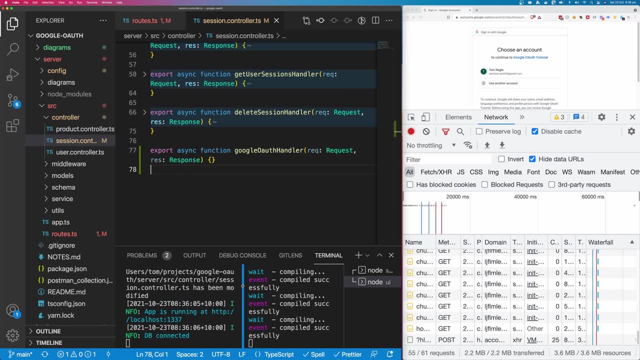 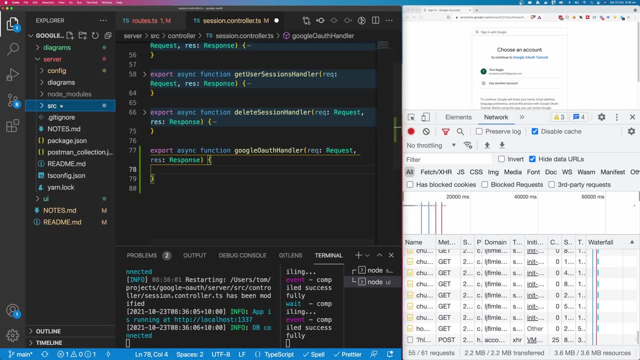 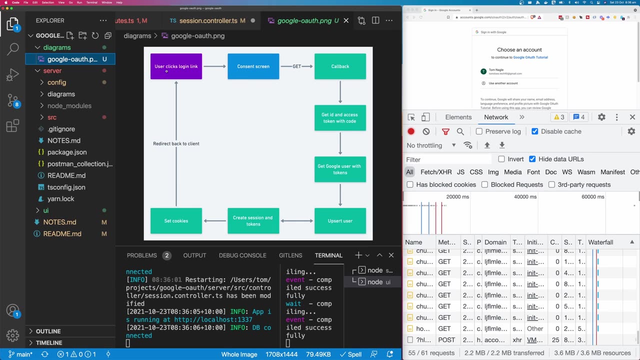 And it looks like our routes are happy. So before we go any further, let's have a think about what it is that this handler should do, So we can refer back to our diagram to have a look. So we've done the consent screen. 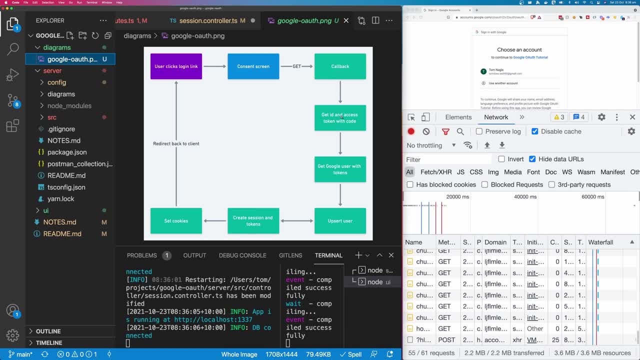 We've done the login link And now we're working on the callback here, So we're going to get the ID and access token from the code. Okay, So we know we need to get the code And we looked at this URL before. 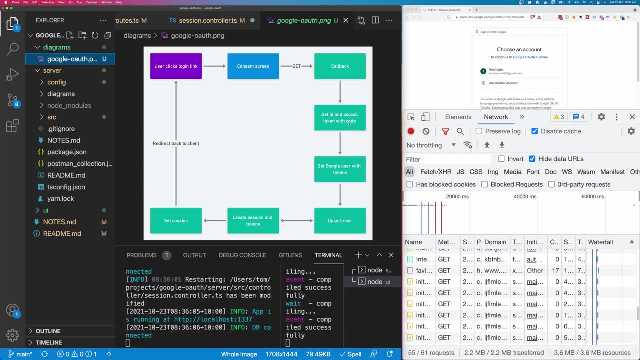 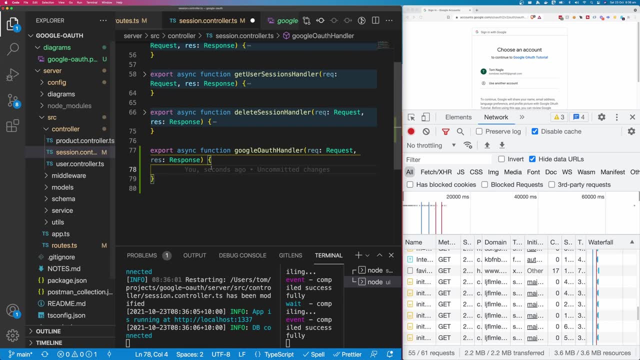 We know that that code exists in the query string. We obviously need to get the code out of the query string, And then we need to make a request to get the ID and access token. So let's go write that down. So we need to get the code from the query string. 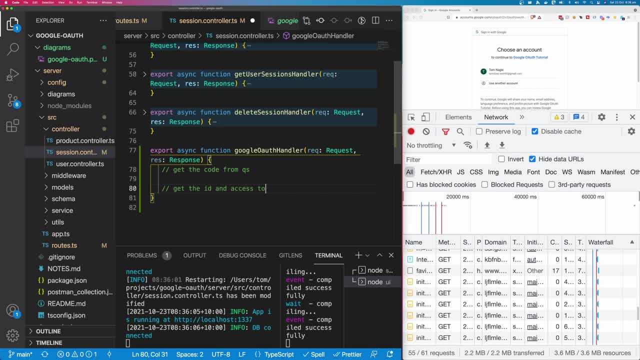 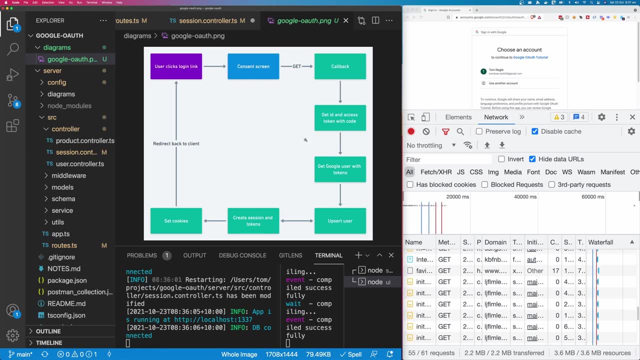 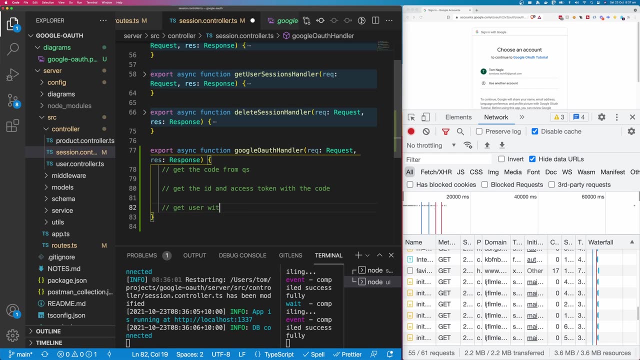 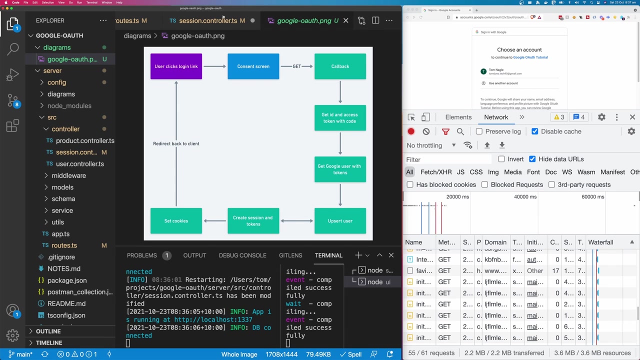 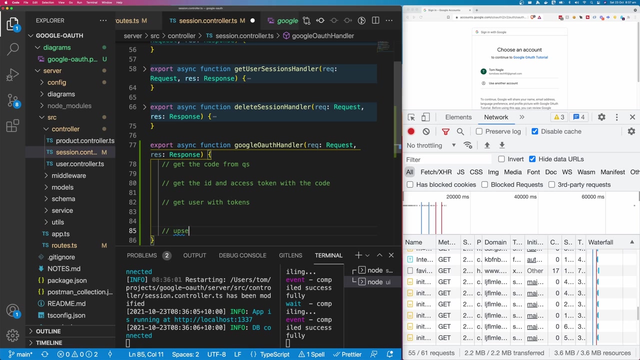 And then we need to get the ID and access token with the code. Okay, Then we need to get the user with the tokens. Okay, Let's say, get user with tokens. Then we need to upset the user and create a session. So we're going to upset the user. 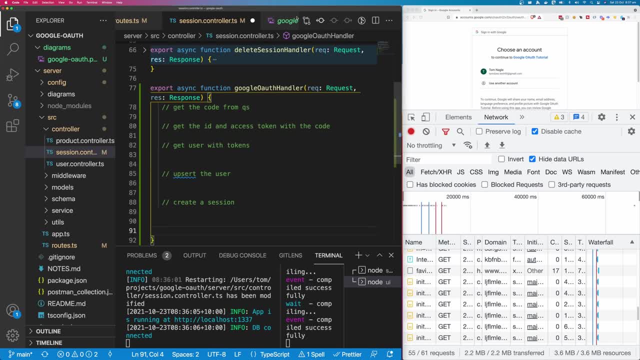 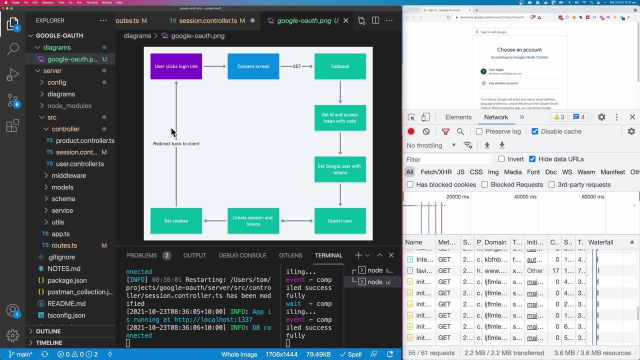 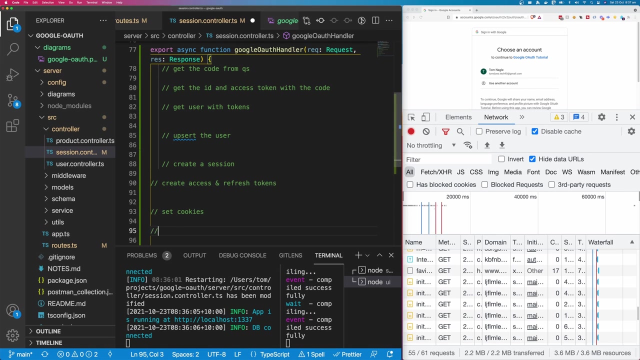 We're going to create a session, Then we're going to create access token, Access and refresh tokens, And then the final part here is we're going to set a cookie And then we're going to redirect back to the client. So set cookies. 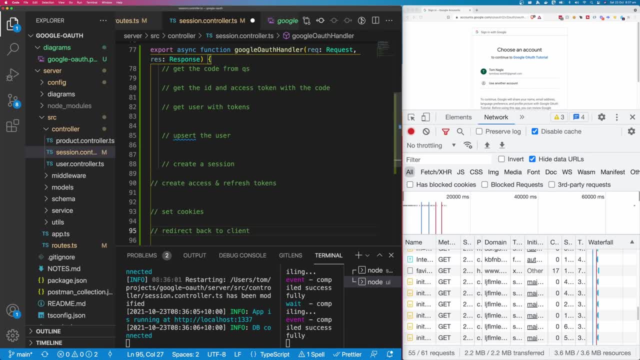 Redirect back to client. Okay, This looks good, So let's go start filling this out. So I'm going to say const code is equal to requestquery And we know this is going to be a string, So let's type this as string. 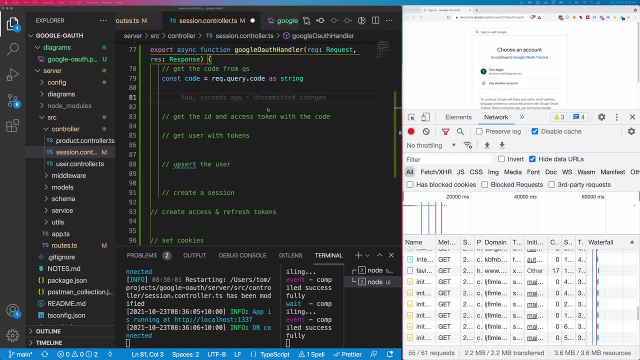 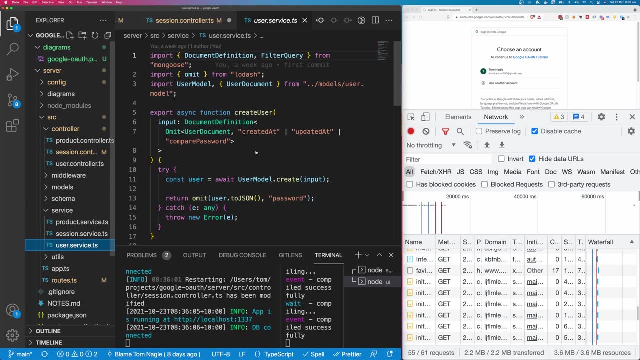 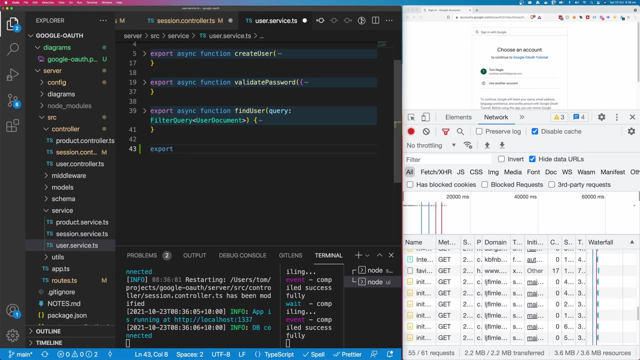 So get ID and access tokens with the code. So to do this, I'm going to create a service inside of user service. I'm going to come into user service And I'm going to say: export async function. Get Google OAuth tokens. 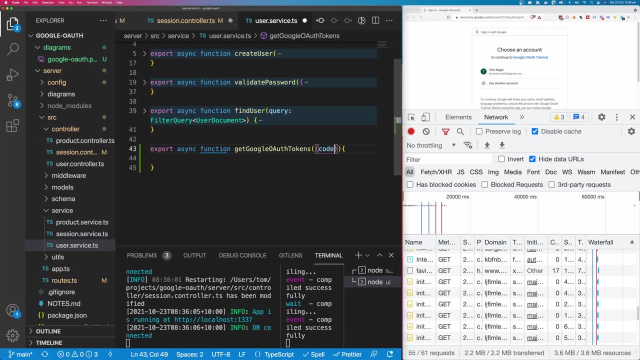 And this is just going to take one argument, And that is the code. And then we can type the code here. Code is going to be a string, So we need to make network requests. So before we go any further, Let's install something to make these network requests. 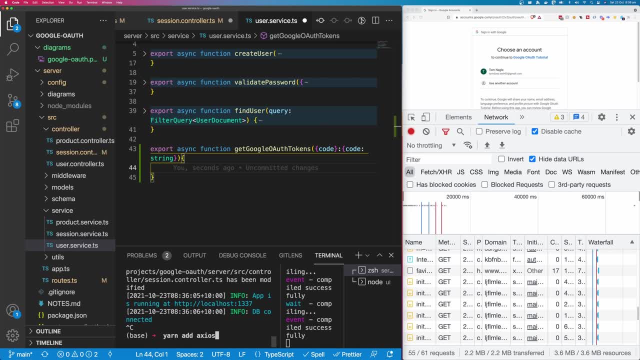 So I'm going to say yarn, add Axios. So while that's installing, I'm going to define a URL Equal to HTTPS OAuth To Google APIs Dot com Slash Token. So if you use the Google APIs MPM package, 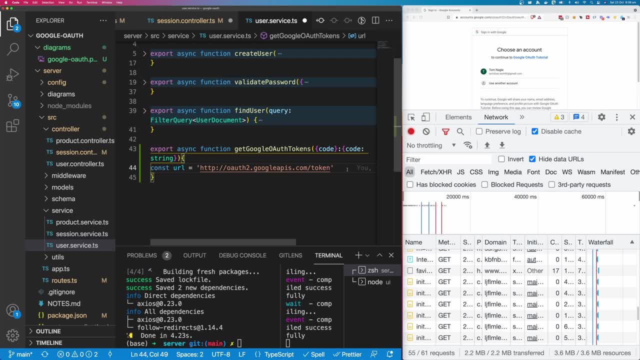 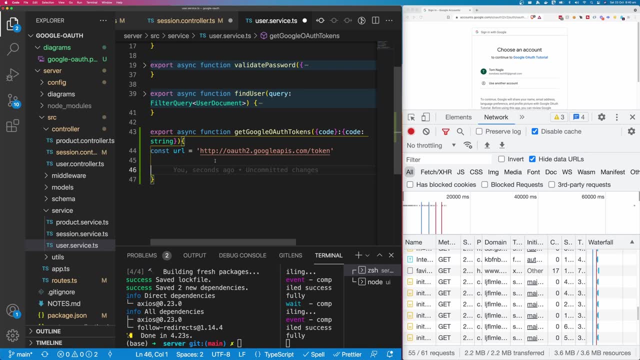 It probably has stuff to do this for you. I can't remember. It's been a while since I used it. I tend to just do this all myself Because I think it's not that difficult. Let's say, const values, And we're doing a similar sort of thing that we did before. 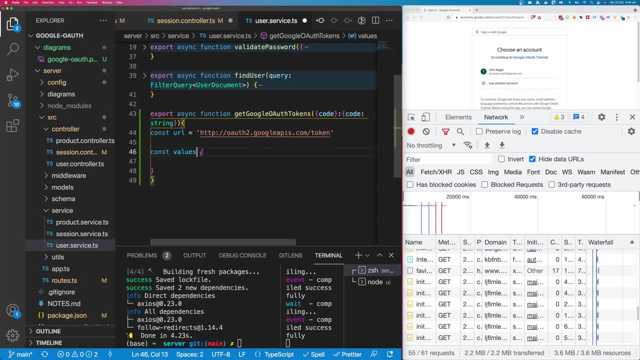 So we're going to define a base URL, We're going to define some values, And then we're going to turn those values into query strings, And then I'm going to send a request off to Google. I'm going to say code: 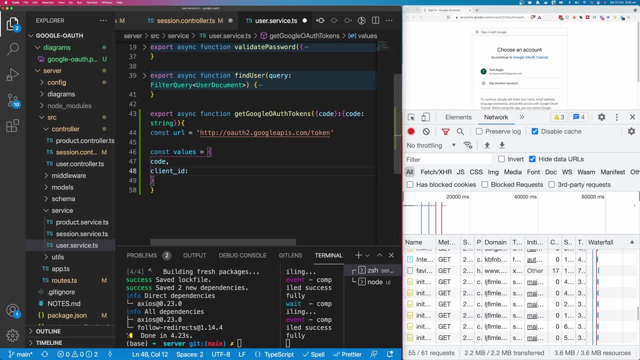 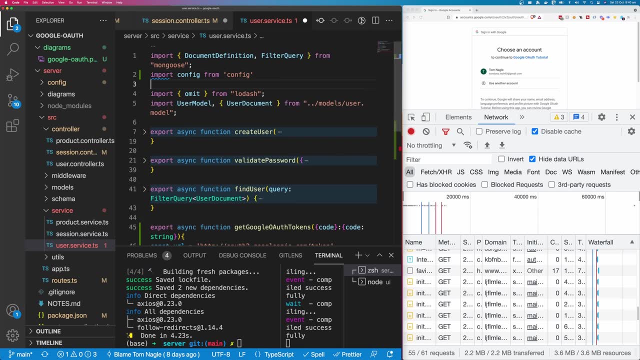 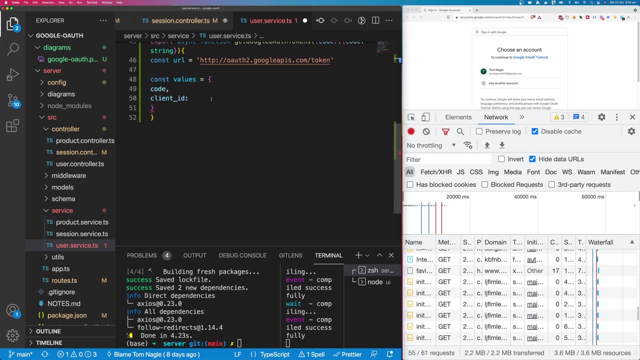 Client ID And we need the config module for this. Let's go make sure we've imported configs. Import config From Config And we're also going to import Axios From Axios While we're up here. So I'm going to say config. 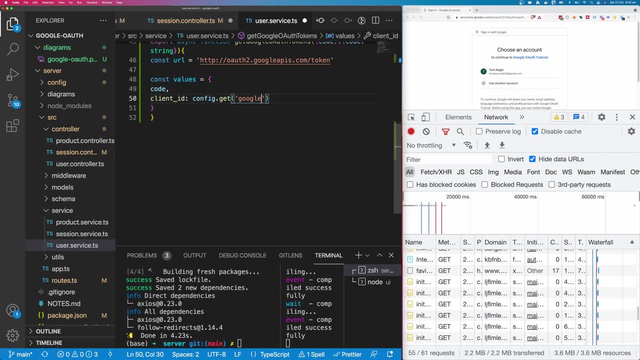 Dot get And we call this Google Client ID. We need our client secret. So I'm going to say client Secret. I'm going to do this The same thing: Config Dot Get Google Client Secret. 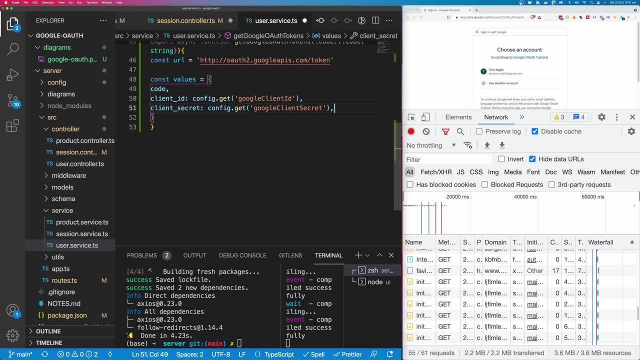 We need our redirect URI. So I'm going to say redirect URI. It's config Dot- Get Google O or Redirect URI. And our grant Type: Config Dot- Get Google O or Redirect. 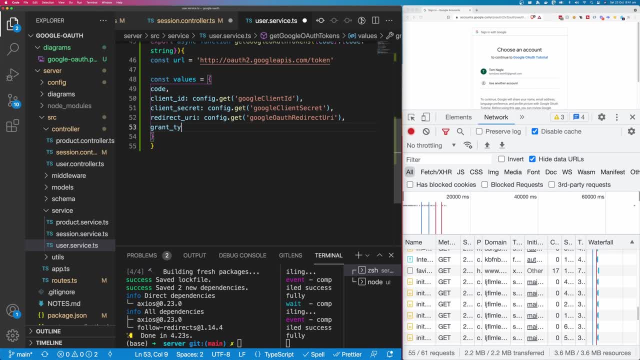 URI And our grant Type, Get 14.. It is going to be Authorization Under score code. Okay, So these are our values. So now let's use these to make a network request And, as we know, network requests can fail. 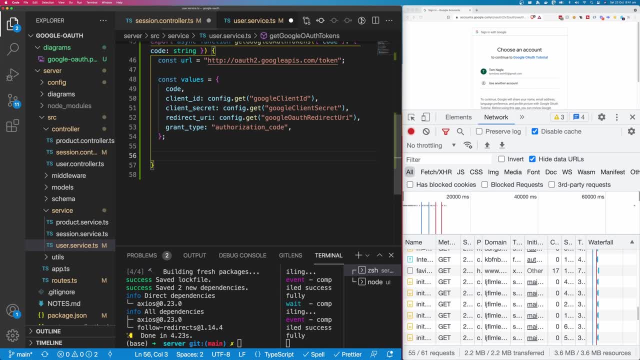 So we need to wrap this in a try catch block. So I'm going to say try And catch the error down here, Define error as any. Up here I'm going to say, try, catch, Let's check this out. So let's see this. 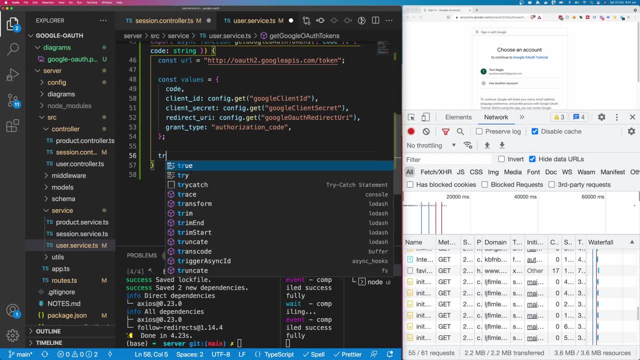 Look at this. It's going to be Not a difficult, It's going to be Pretty easy. You're making a lot of noise Change to Pretty easy. I've got eight Has changed out. I've changed it. 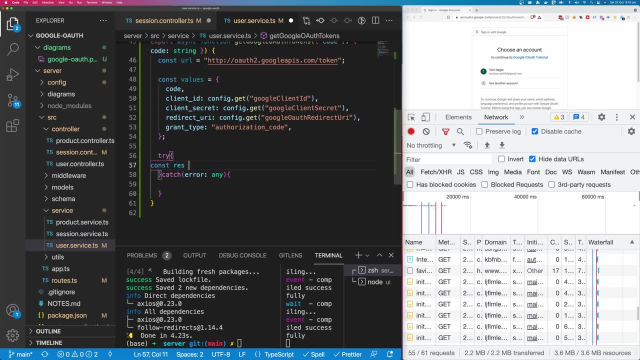 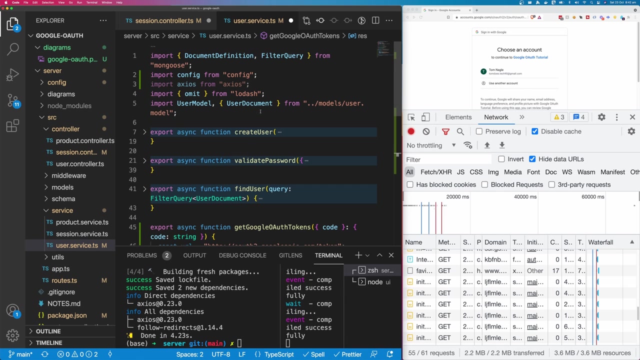 Now Up here I'm going to say const res equals: await Axios dot post And we're going to post to our URL just to find up here, And our URL is going to have a body of QS dot stringify. And if you remember before, QS comes from the query string package. 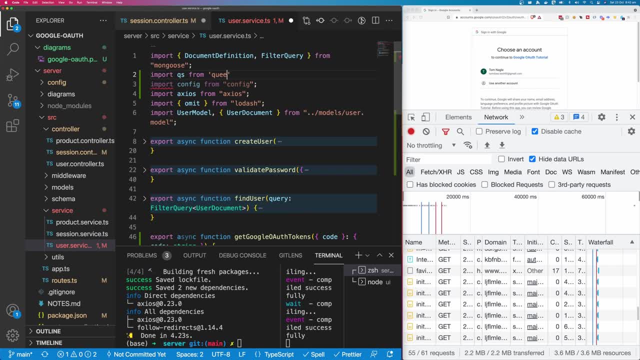 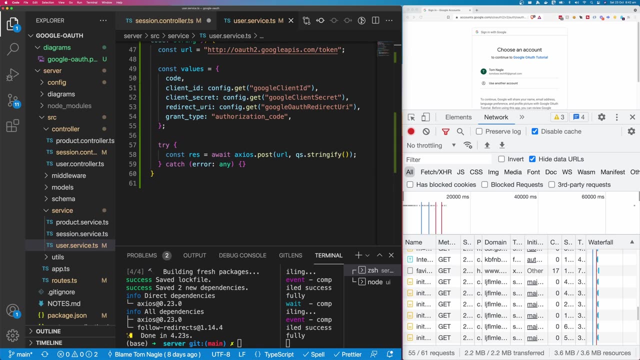 So let's import that. And when I said it was deprecated, I mean that it's deprecated on the client. You can still use this inside of node And this comes from QS. sorry, And I also need to set some headers here. 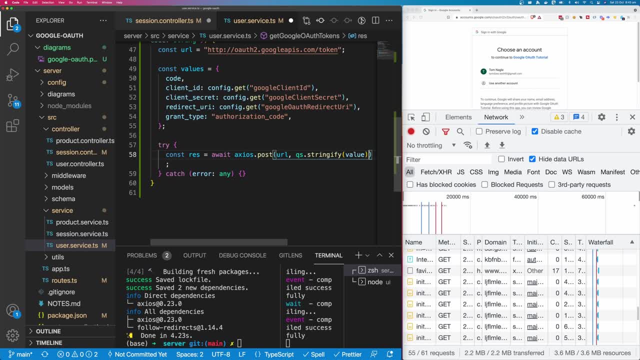 We need to pass in values into our QS, dot stringify, And we need to set some options. And in options we need to set some headers, And the one header we need to set is going to be content type. So I'm going to say content type. 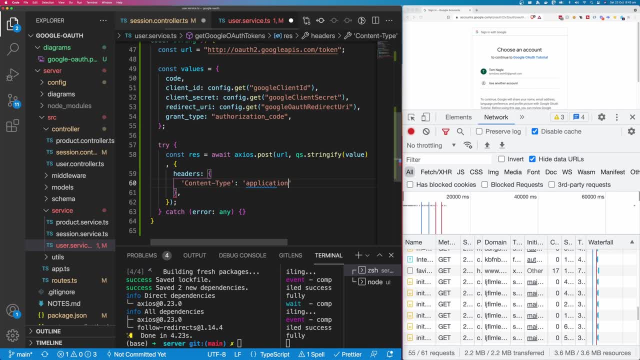 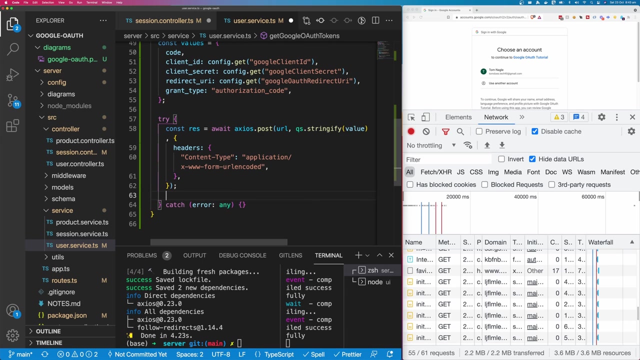 And this is going to be equal to application slash x www form URL encoded. So this is just going to tell Google OAuth APIs how we've packaged up this data. So we've done it via URL And finally we're just going to return res dot data. 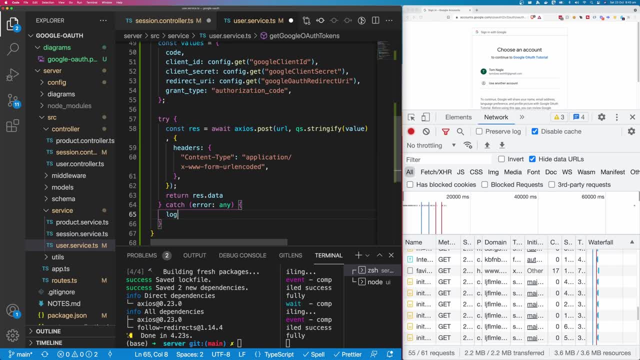 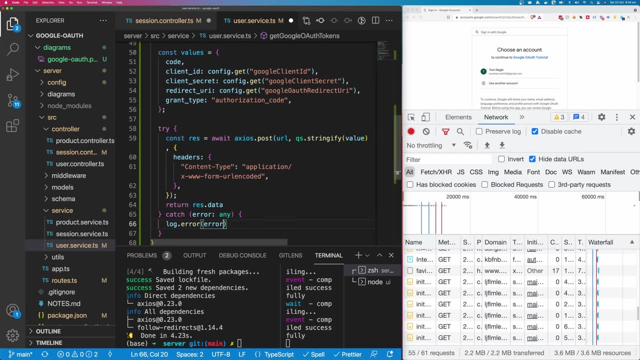 If we have an error message, we want to log that error. So I'm going to say log, I'm going to import my logger dot error, I'm going to put in the error here And then I'm just going to say: failed to fetch Google OAuth tokens. 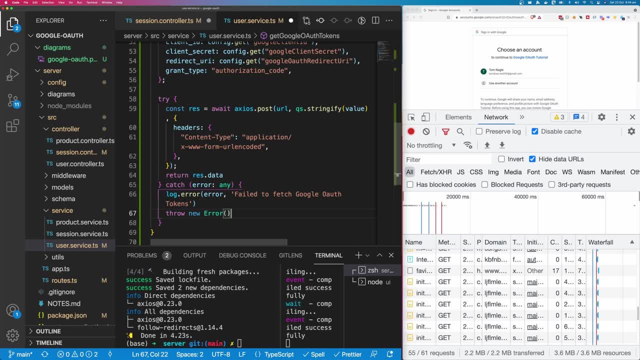 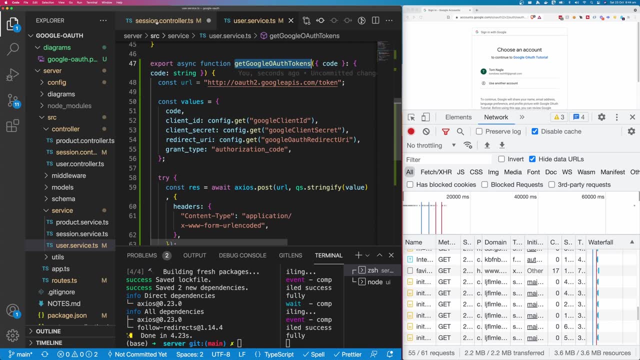 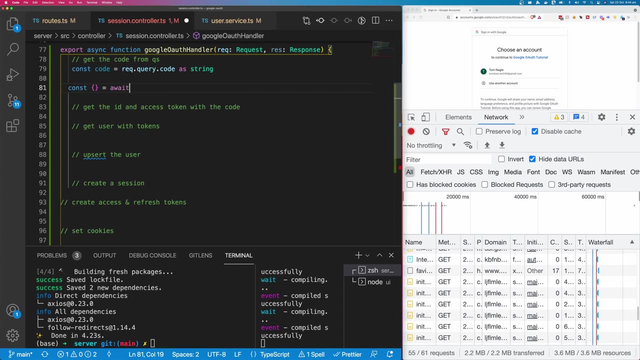 I'm going to throw new error, error dot message. Okay, this looks good. Let's go use this function inside of our controller. I'm going to say const And then I'm going to destructure here. I'm going to say equals, await- get Google OAuth tokens. 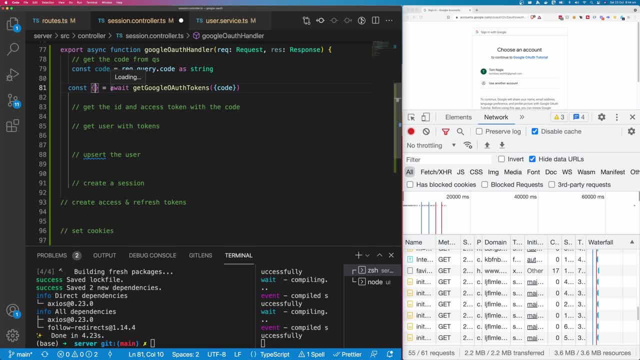 And we just have a code here So we know this function returns an ID And then we're going to say return access token And it also returns an access token. So we've done this part here. We can console, log these here and just make sure this works. 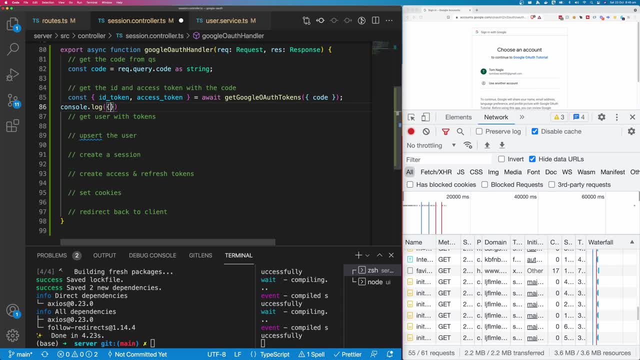 I'm going to say console log. I'm going to add the entire object to the console log. Start the server back up. Now I'm dev, Okay. So now that the server has started back up, we can click the login with our Google account. 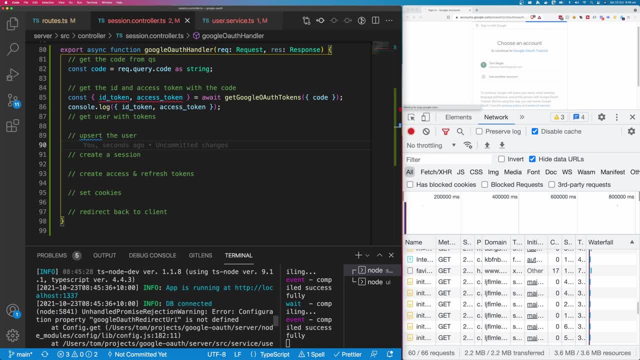 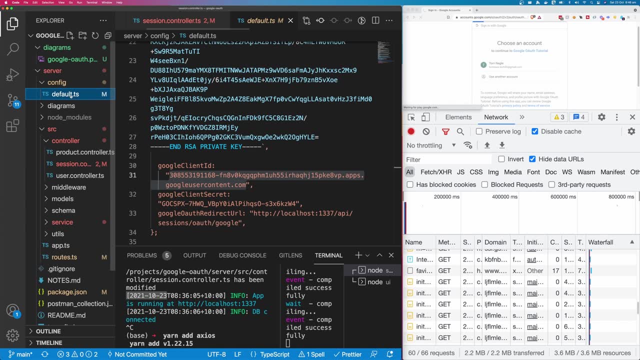 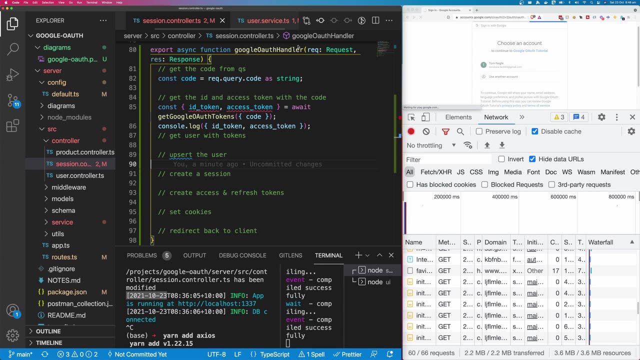 So we have an error here. It says Google OAuth redirect URL is not defined. So let's have a look inside of our config module in default And we have Google OAuth redirect URL here And I assume I just spelt this wrong. Go back into this function. 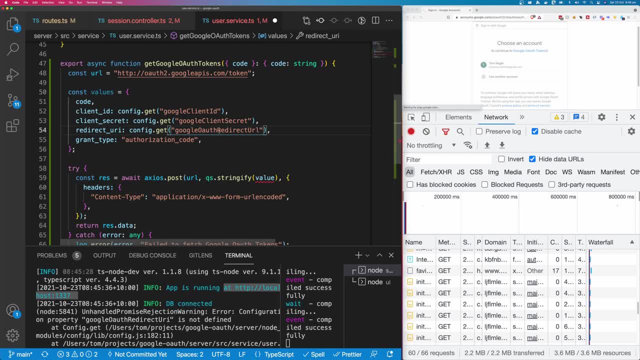 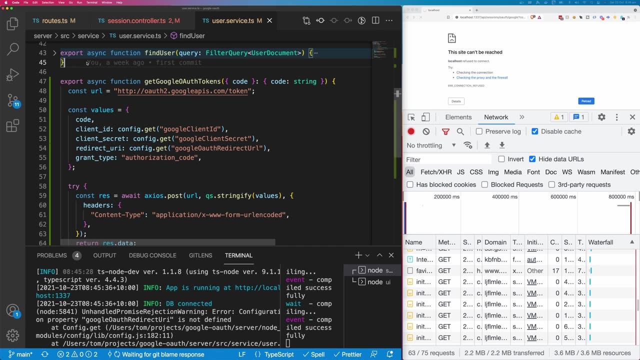 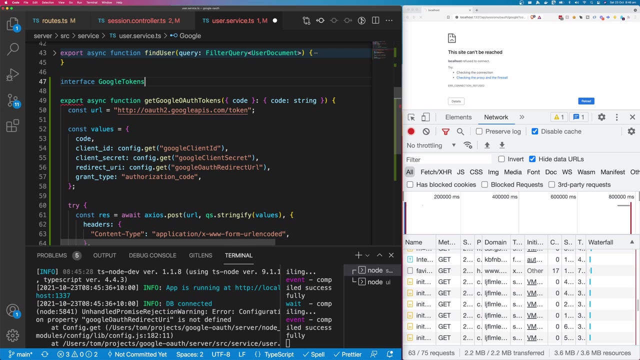 Okay, that was URL, not URI, And we've also called this value, not values. And let's also tell TypeScript what this function should return. So I'm going to say interface, Google tokens, result, And this is everything it's going to return. 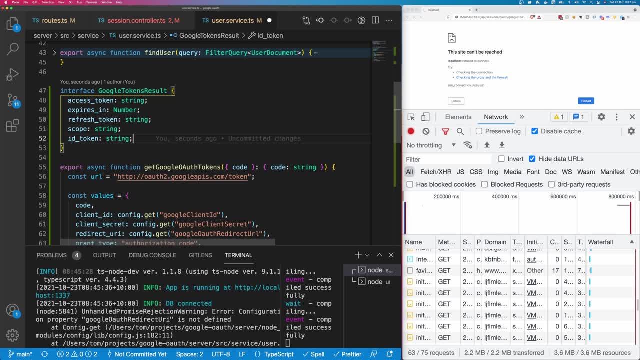 It's going to return. It's going to return an access token, an expires, in which is going to be a number, refresh token, scope, and an ID token. The two that we care about is this: access token and ID token. 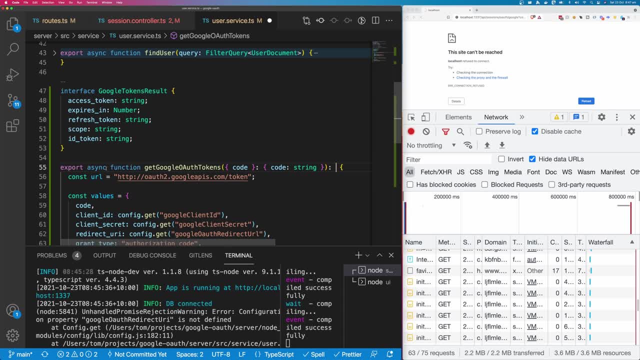 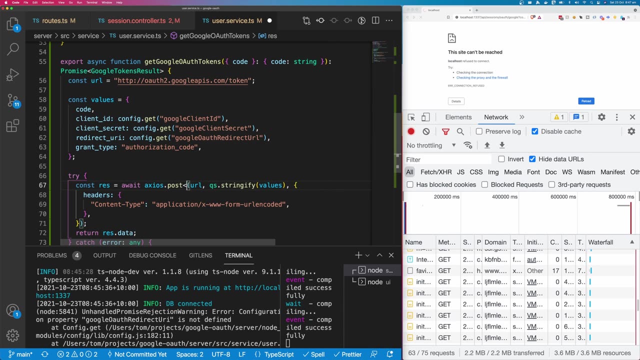 So let's come type this: So we have an async function here, So we know this is going to return a promise, And then we know the promise is going to return this object here. So let's also tell Axios what it is that we're expecting the request to return. 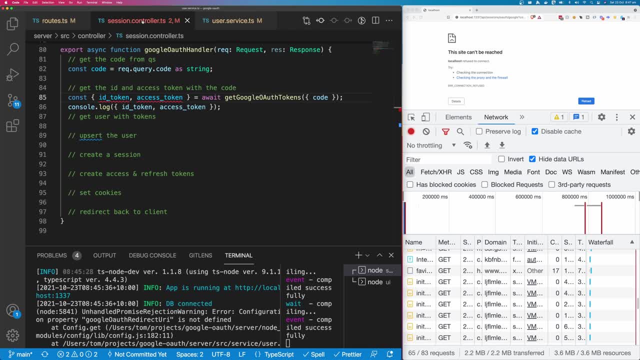 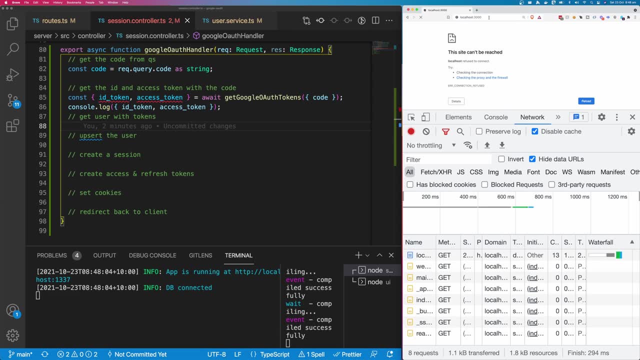 So I'm going to use this generic. I'm going to pop that in there. So we failed hard on the server, So I'm just going to restart it here. So let's click log in with Google. again, I'm going to give my consent. 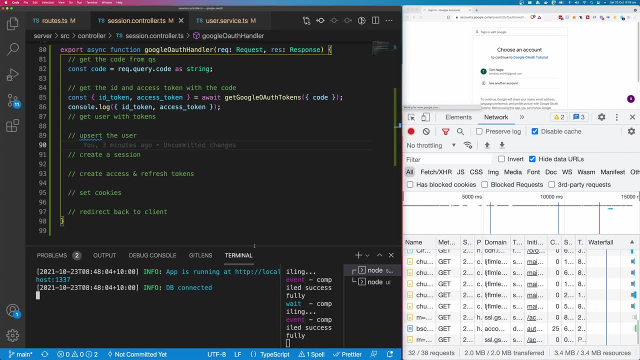 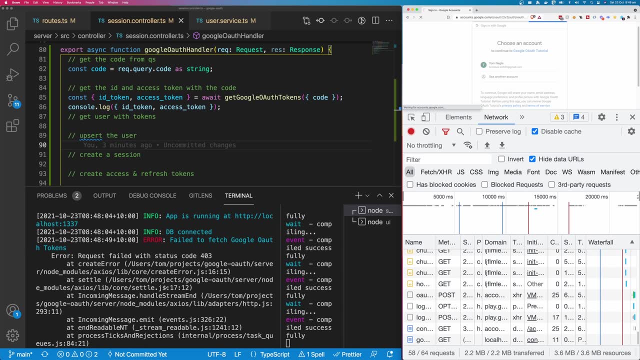 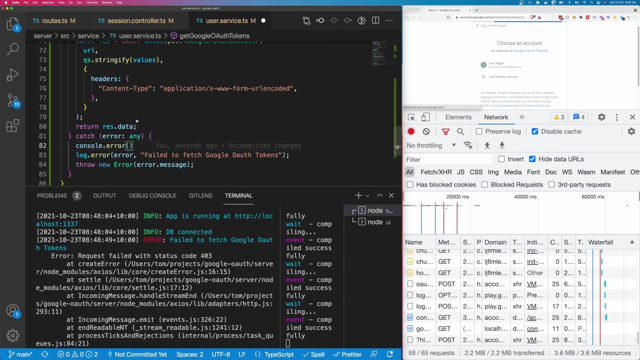 And we should expect some tokens to appear in the console here. So we have a 403 error here. So this means that we've sent our post request in user service And Google APIs has returned a 403, which is unauthorized, So I'm not sure why it sent this response, but we're going to figure it out. 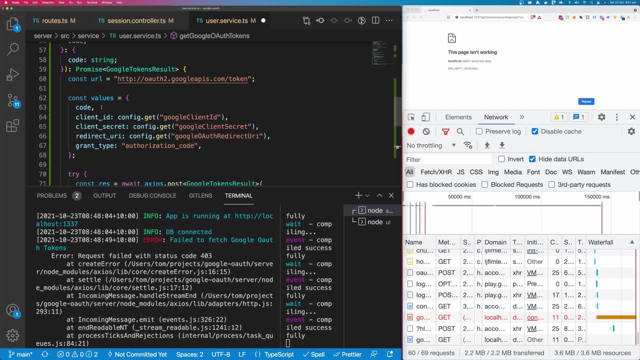 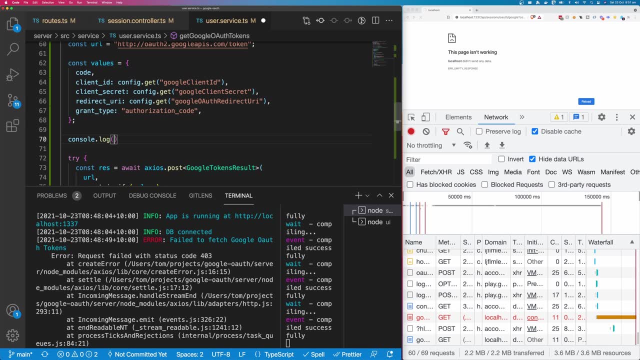 So the first thing I'm going to do is to check the response. So I'm going to check these values here and they all look correct. but let's console log them out. Console log values. make sure they're all good, And then the next thing I'm going to do is I'm going to add a consoleerror here. 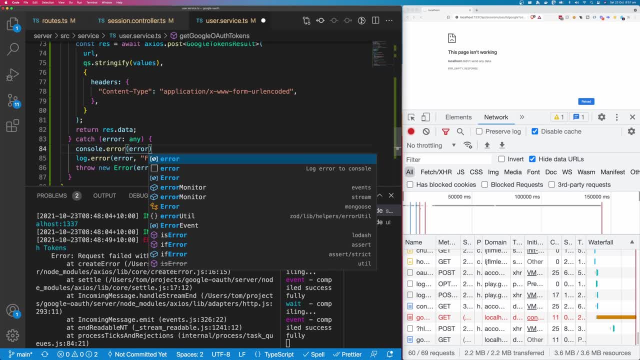 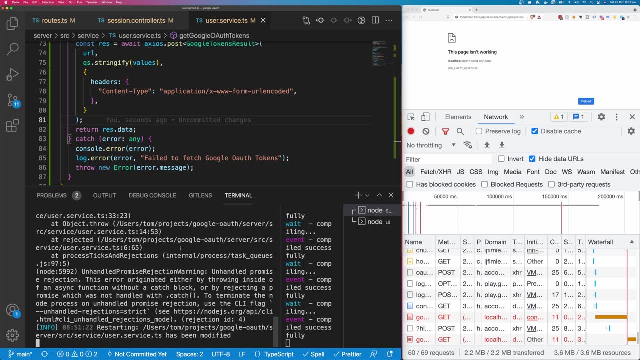 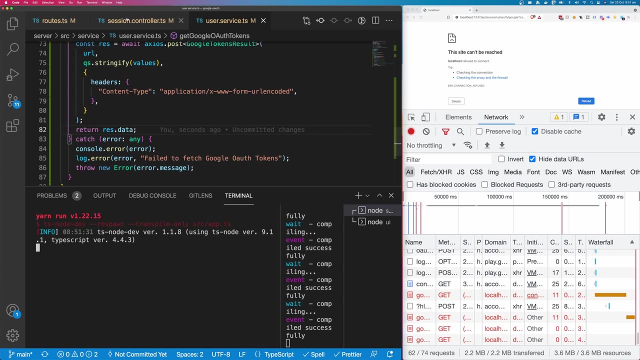 And I'm just going to console error And we're going to put our error in here. Let's save this and we can try again. Okay, And the reason we're getting an unhandled rejection is because in our controller over here we're not catching these errors. 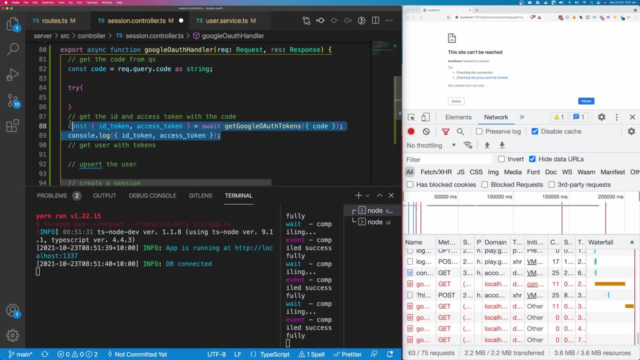 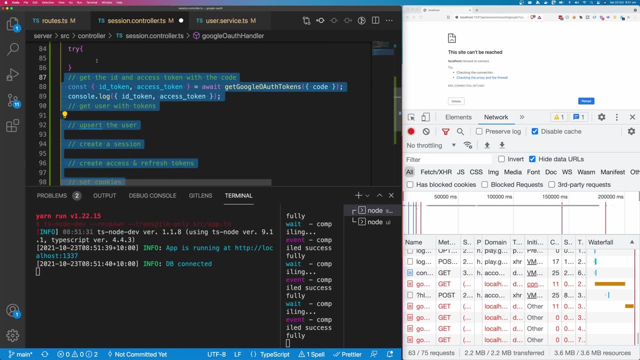 So let's do that, because having unhandled errors is very bad practice and it's going to lead to a lot of problems. So you're going to make sure you are handling these errors, And getting the errors during development is actually kind of good, because it means that you will be forced to handle them. 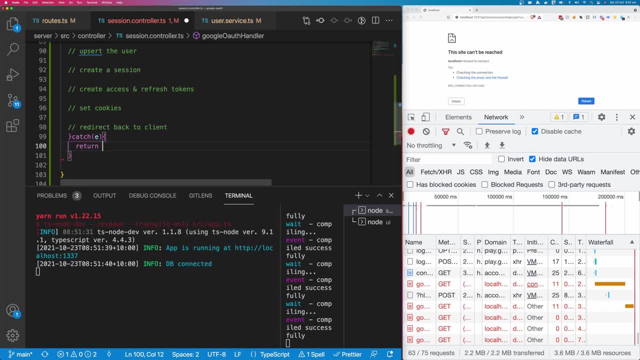 So if it does, then you're going to be forced to handle them. So if it does throw, we're just going to return and say resredirect, And we want to redirect back to the client. So I'm going to say configget. 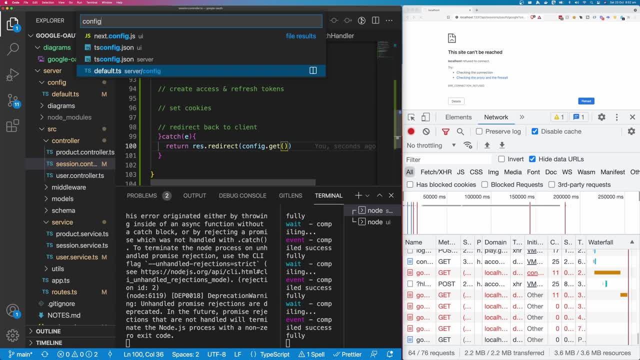 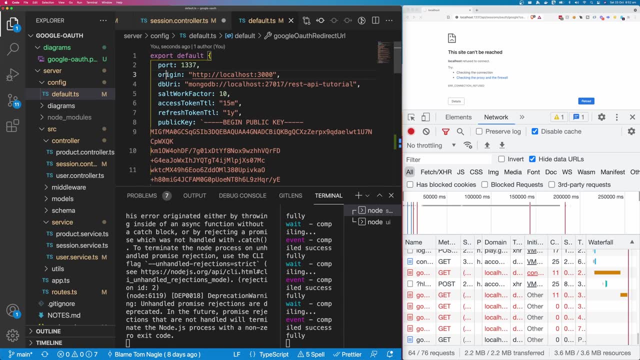 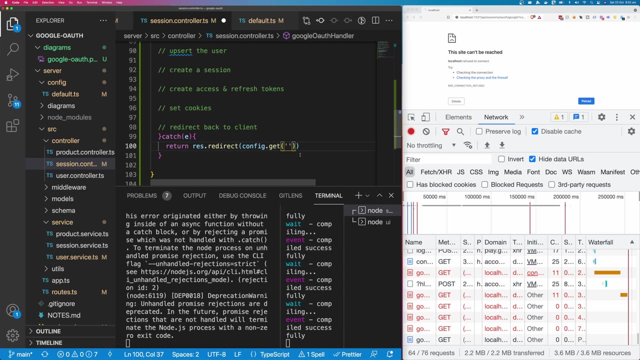 And in our config we have this origin that we use for cause. So I'm just going to redirect back to this origin here. But if you don't have this origin set up because you didn't follow my previous tutorials, that's okay. 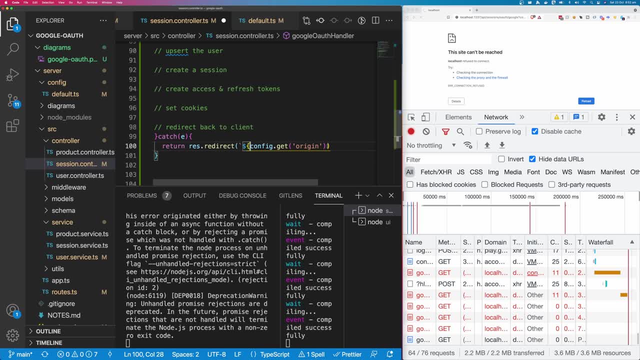 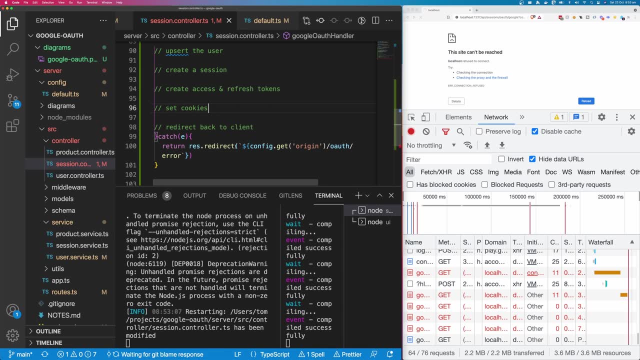 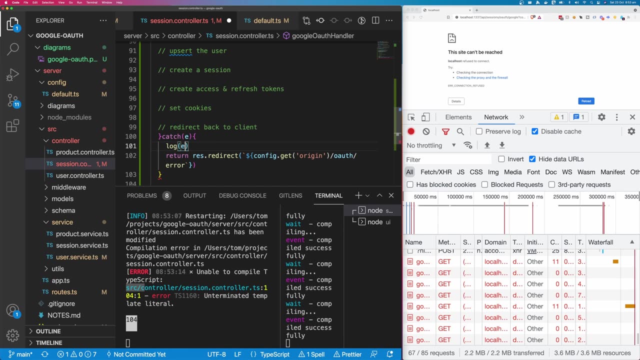 I'll forgive you, But you'll need to set up a path back to the client. So I'm going to say slash oauth, slash error, And you'll probably also want to log this error. So log, I'm just going to put in the error. 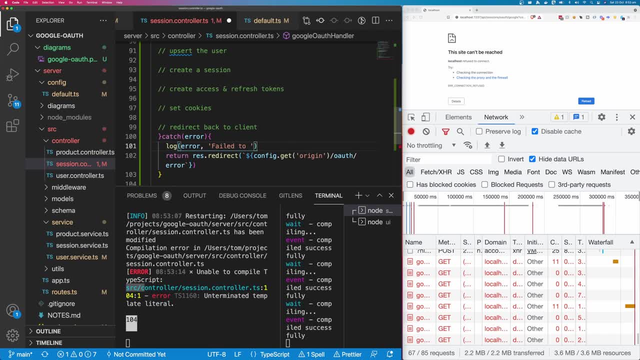 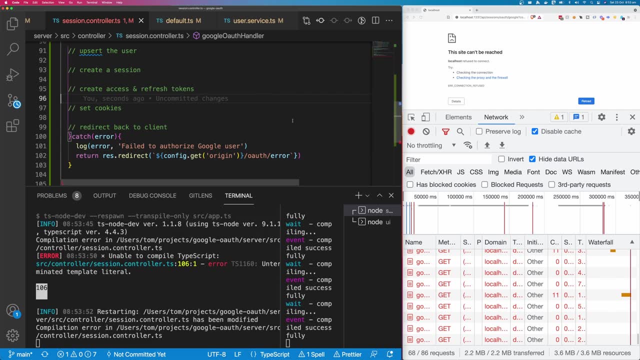 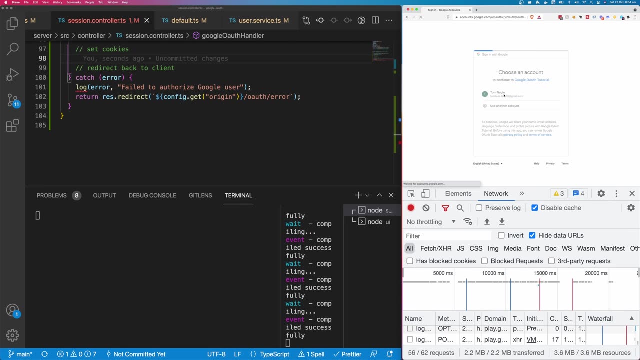 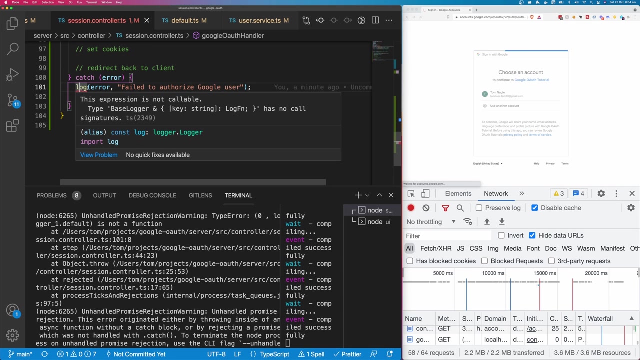 Let's be consistent here with our naming. Okay, So we've got some good logging in place Now. So let's go try this again. So we've introduced another error here We have: loggerdefault is not a function, So that's because we haven't put logerror. 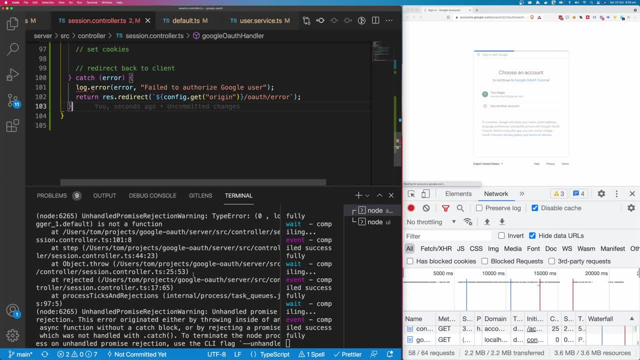 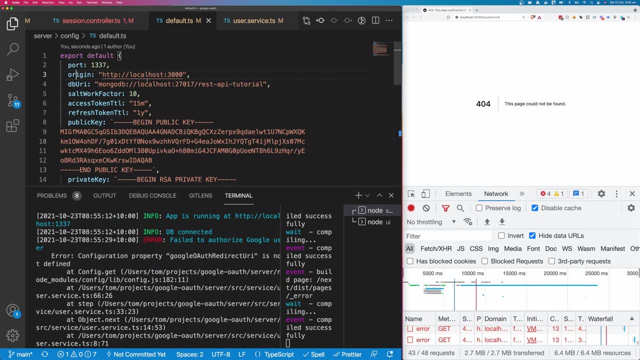 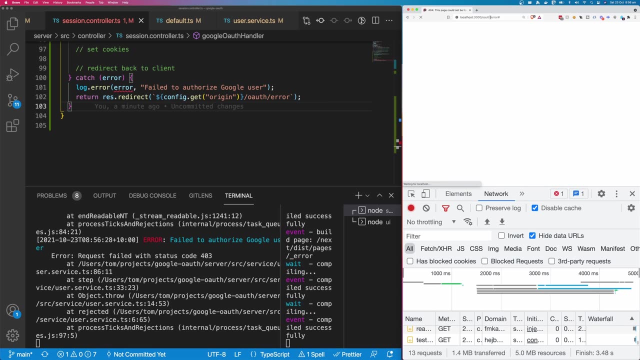 We've just tried to call the defaults export here, which is not valid. We've added a new function here, So the default is layout to the client, So we can return that, which will also see this as a new function. So that's going to do anything for you. 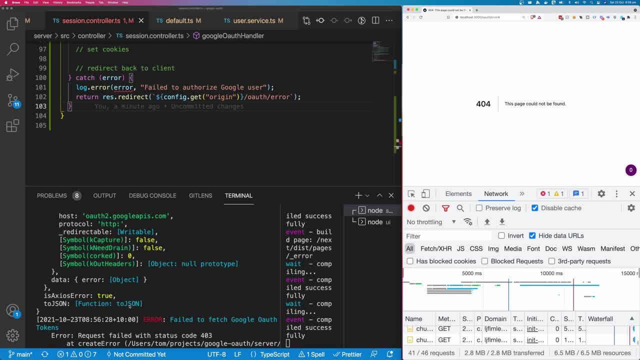 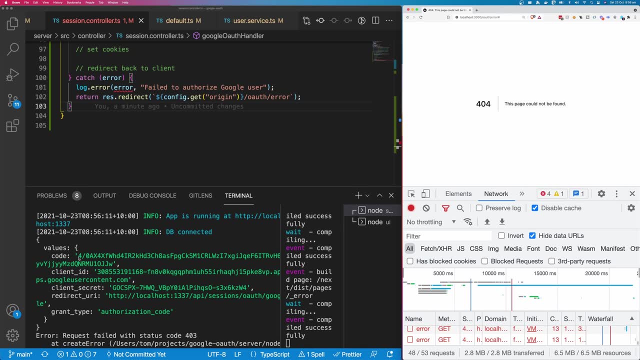 We've got this error here. We've got this client and I'm going to go back over here and we'll see how that's gone. OK, so you can see, our client has redirected back to oauth error. So that's what we expect to happen. 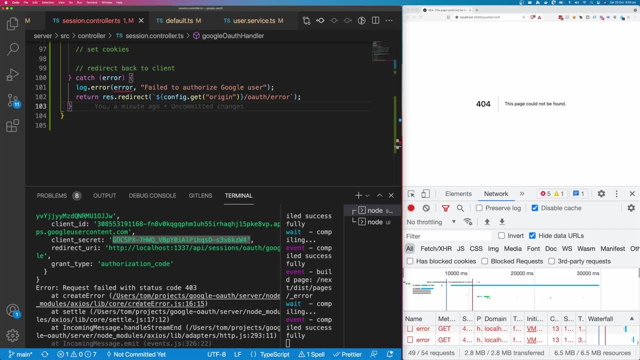 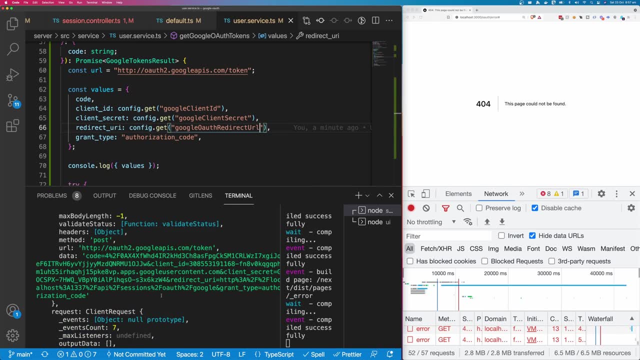 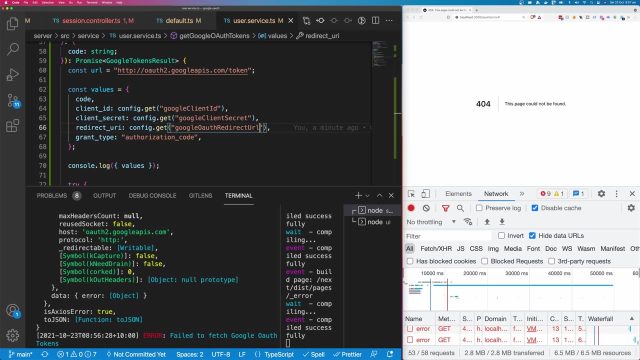 And we have a bunch of stuff here. So the reason I logged the error is because you can see down here we get a response and then we get a data object and we get error and there's something hidden in here. So let's try and get that out. 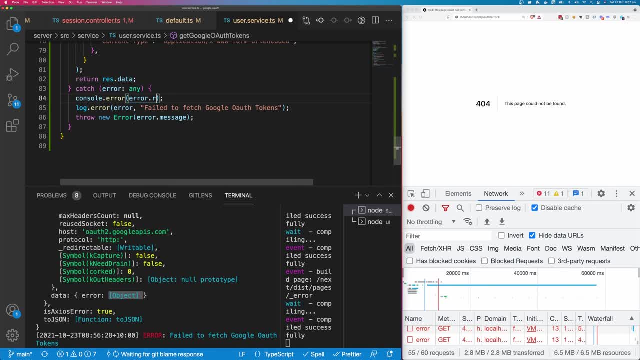 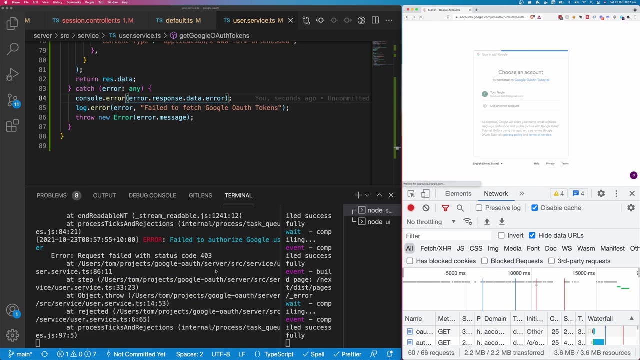 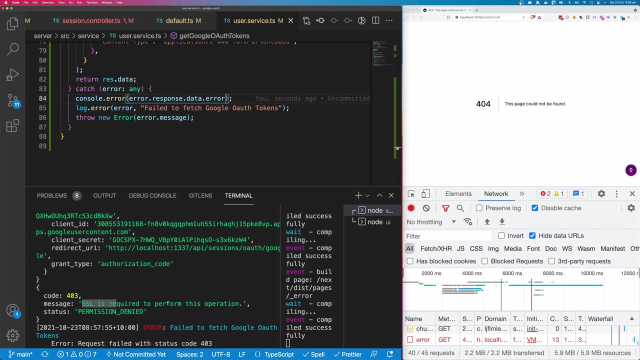 I'm going to say errorresponsedataerror, And hopefully that's the right path to the error. So we're getting 403 and we get an error message here. that is much better. SSL is required to perform this action, So my suspicion is that we're using HTTP here. 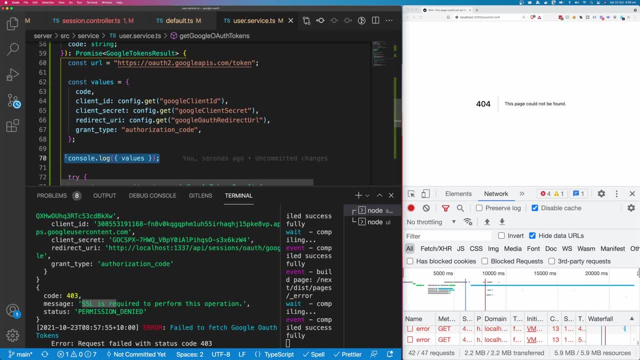 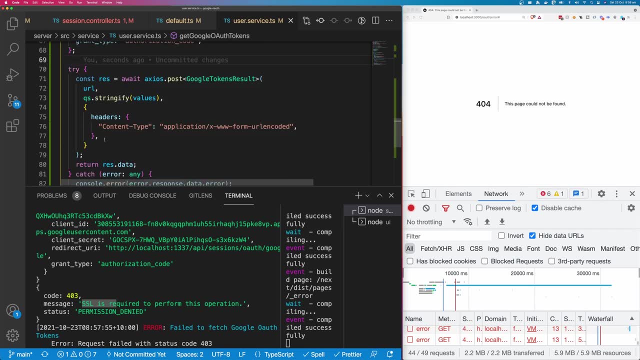 And it should be HTTPS. So this is a good example of why you should copy and paste URLs and not try to type them out yourself, because you're going to get them wrong, or at least I am anyway. All right, let's try this again. 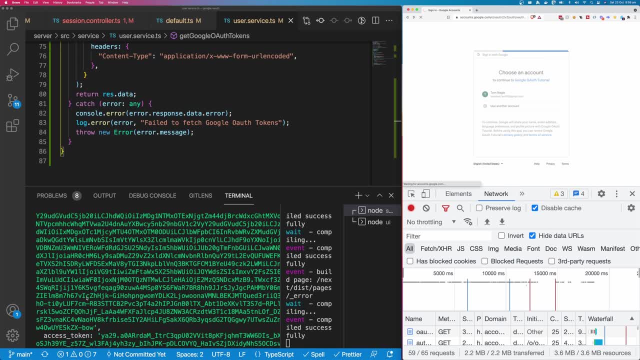 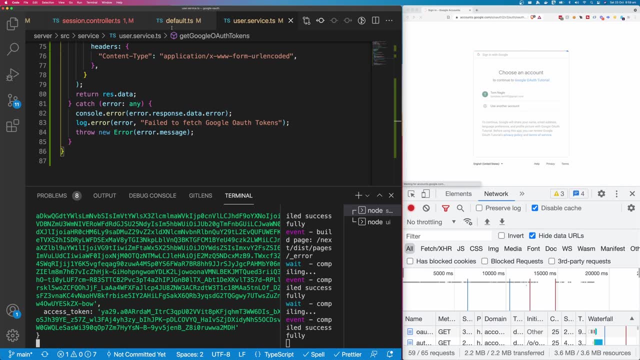 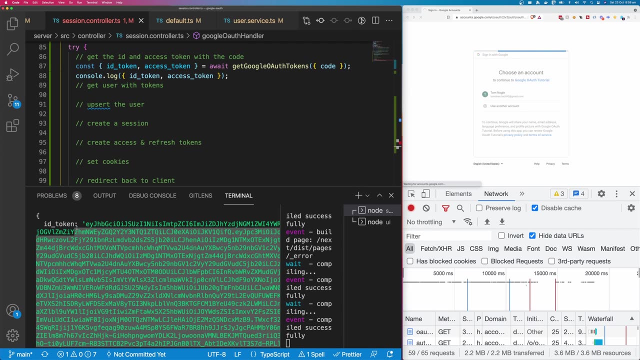 Okay, so we get an access token and we get this ID token here. So let's have a look in our controller. You can see. the next thing to do is to get the Google user. Let's have a look at what these tokens contain. 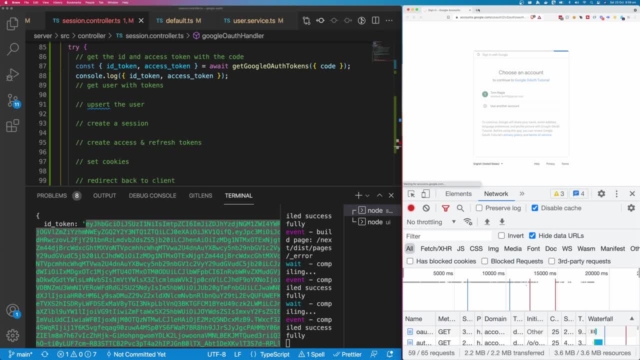 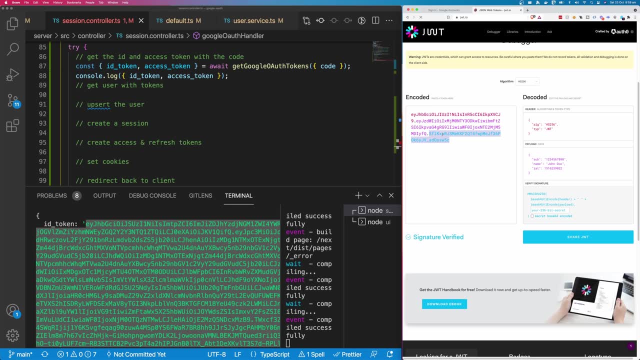 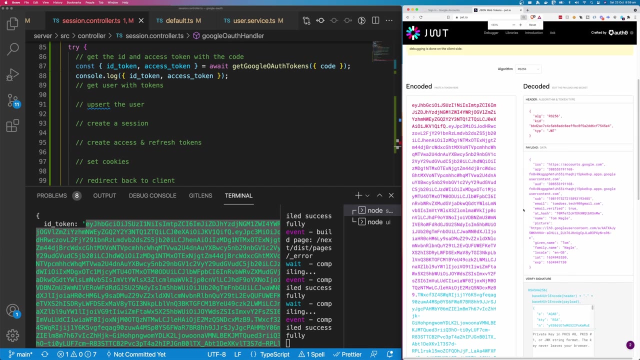 So you can see that they're Base64 encoded. So I'm going to come over to JWTio. I'm going to paste in the contents of this token And you can see here that we get a Google payload. You can see here: we have the email address. 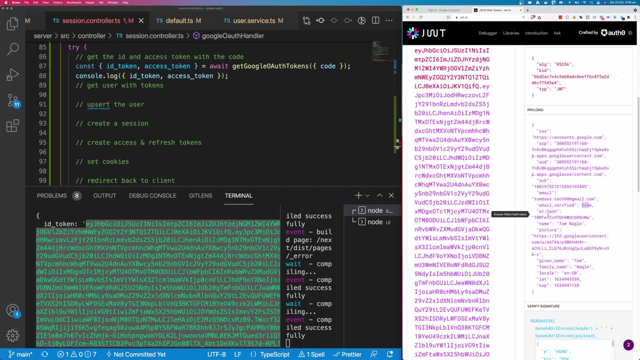 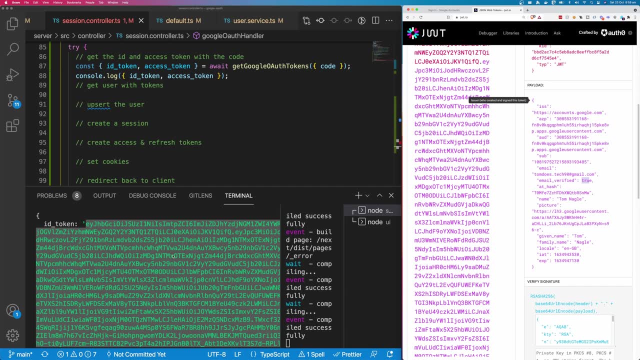 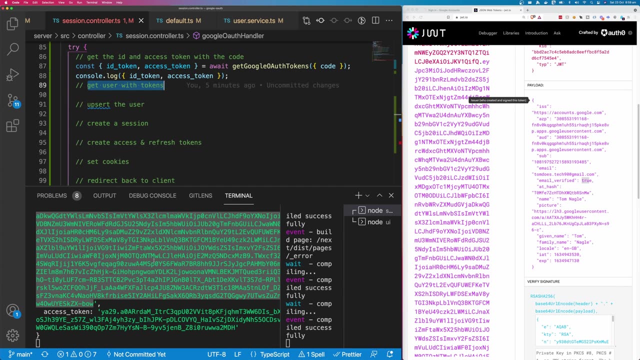 We have a email verified Boolean. We have a name, We have a picture given name, family name, all this good stuff here. So we could use this to get the user. That would be a valid approach And, in fact, that would be the one that I recommend you do. 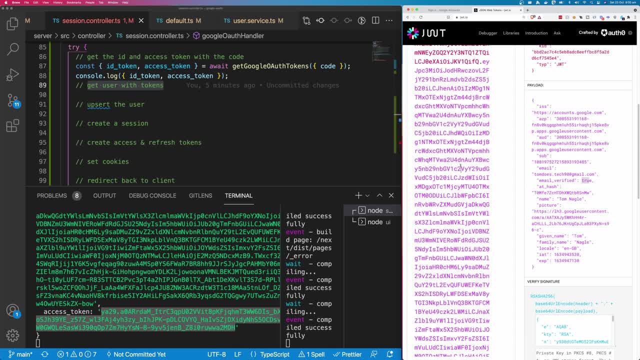 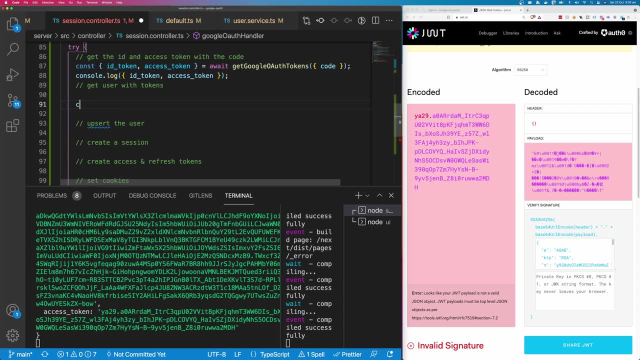 But I'm also going to show you how you can make a network request to get the user. So let's get the user out of this ID token here. So I'm going to say const Google user is equal to, And we're going to use JWTdecode. 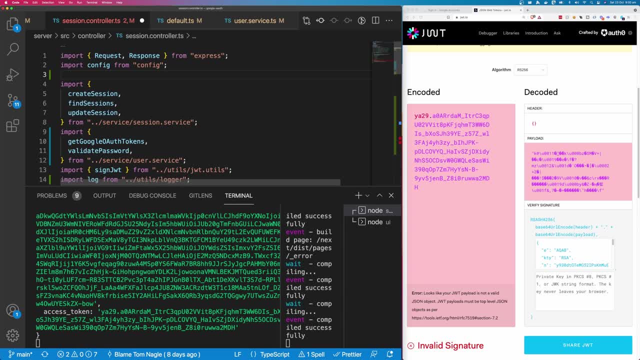 Be careful with JWTdecode because it's not going to verify the token. But we know that this token is signed by Google because we've just made this request server site. So I'm going to import JWT from흰JSON web token. So usually you would want to use JWT. 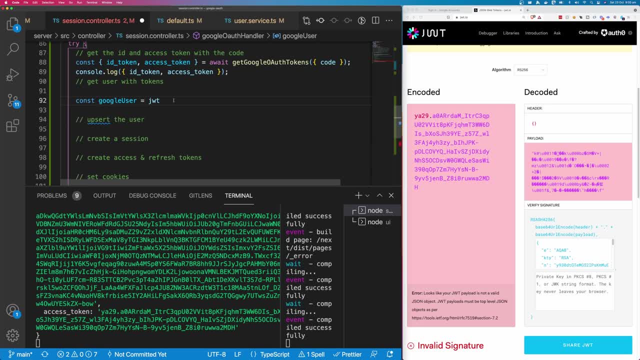 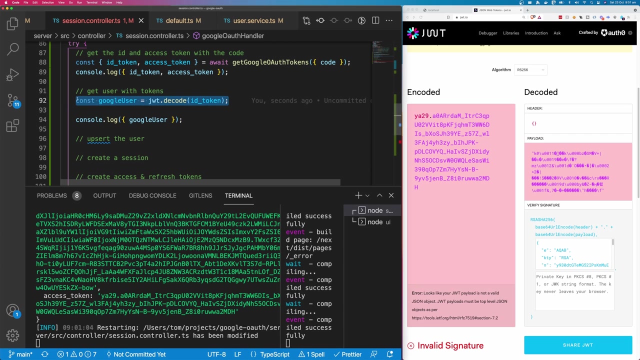 Verify, So you can verify that the token was signed with the key that you expect. it will say floatdecodecam, Let me say ID token And let's say consolelog, Google user. So this is perfectly valid. This is a good approach to this wolf implementation, but you can also use a network request to 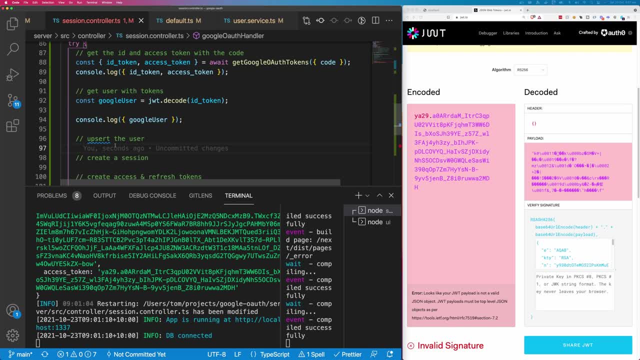 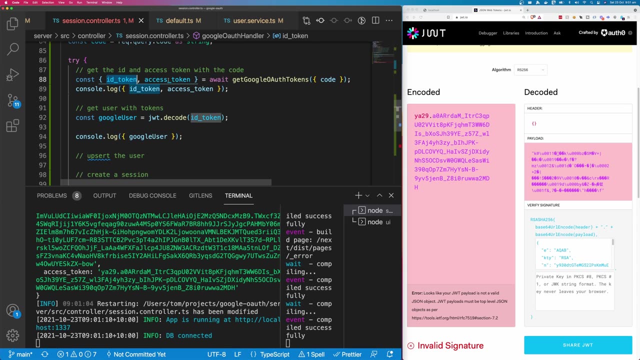 get the user. So for completeness sake, I'm just going to show you how to get that user with the network request. So the reason that you would want to do this is because if you just set these tokens on the client and then the client makes requests to your application with these tokens, you'll 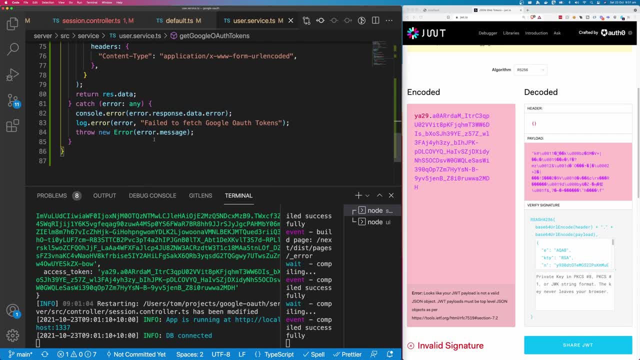 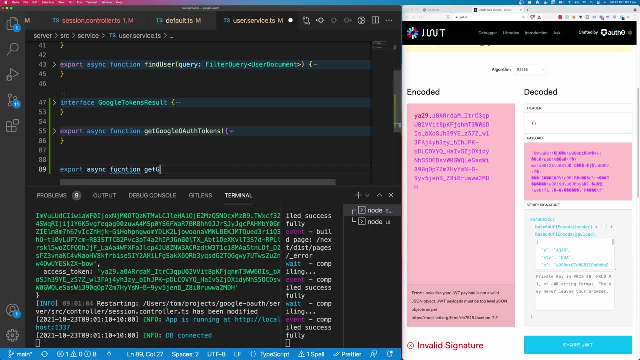 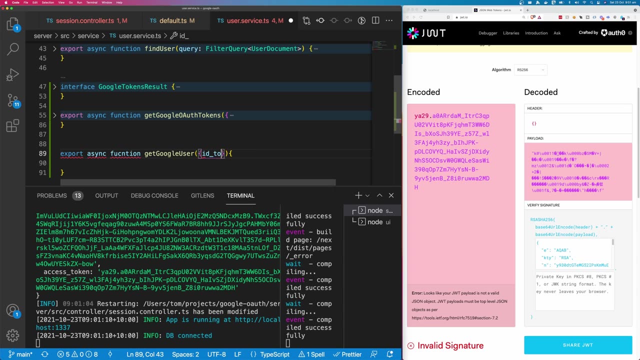 want to be able to get the user, And so you need to have a network request to do that. So I'm going to say: export async function, get Google user. And this is. This is going to take an ID token and an access token. 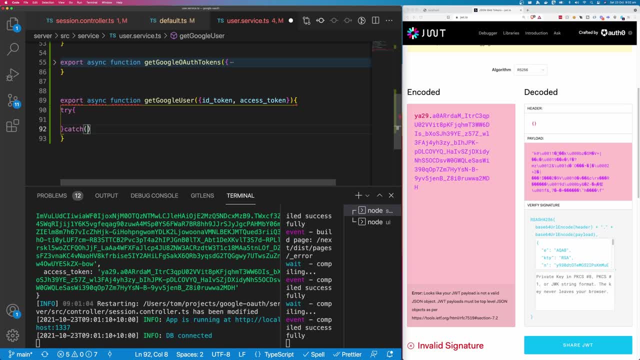 I'm going to add a try catch block here And I'm going to say: const res equals await Axios dot get. And I'm going to get this URL here: Google API Slash- OAuth two slash V1 user info: Jason access token. 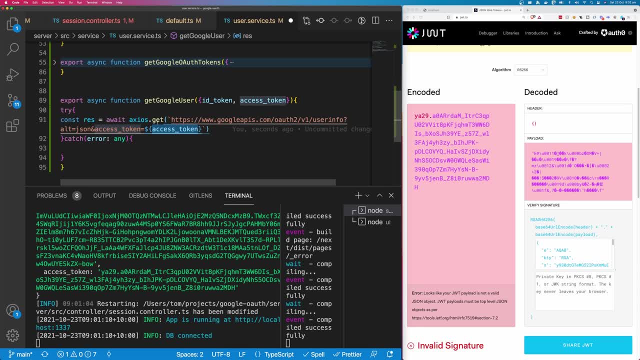 And I'm going to append the access token to the endpoint. I'm also going to set some headers, And the header that we're going to set is authorization, And we're going to add bearer And ID And ID Token. 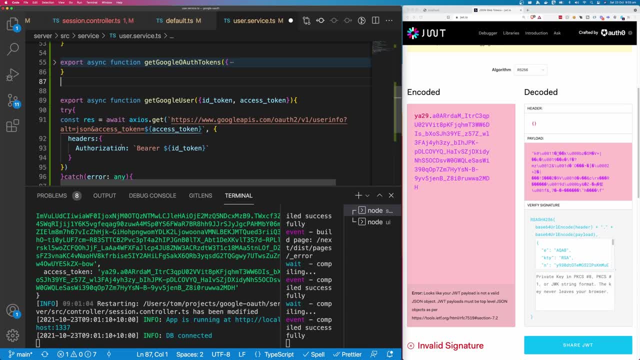 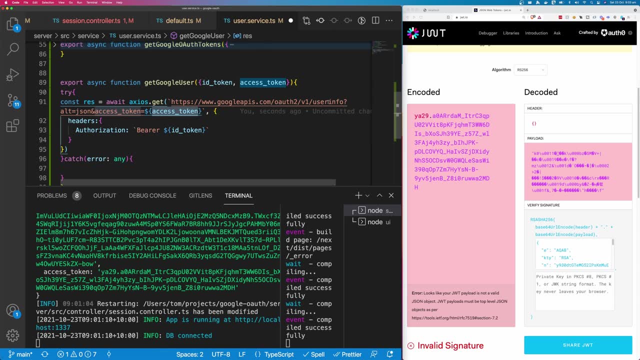 So we're going to use the ID token to verify that we are who we are And we're going to tell Google we want to use this access token to get the user info And, because we added user info to the consent screen, we're going to have access to this. 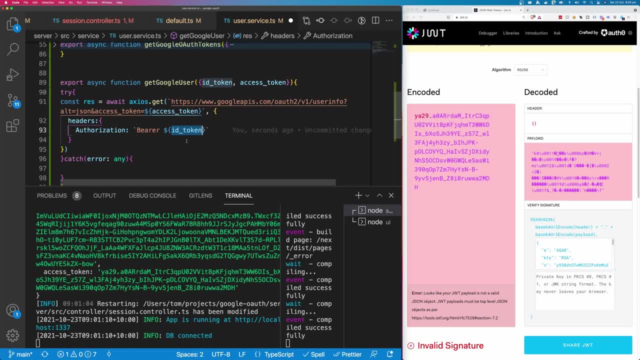 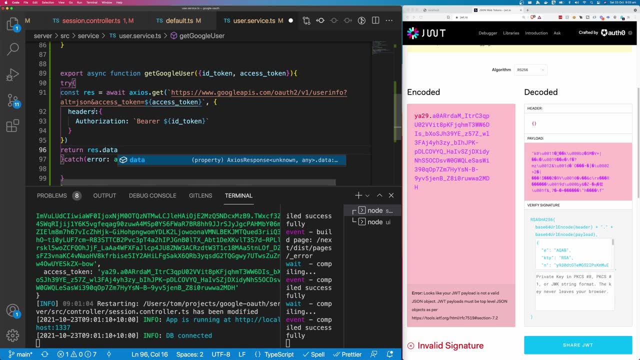 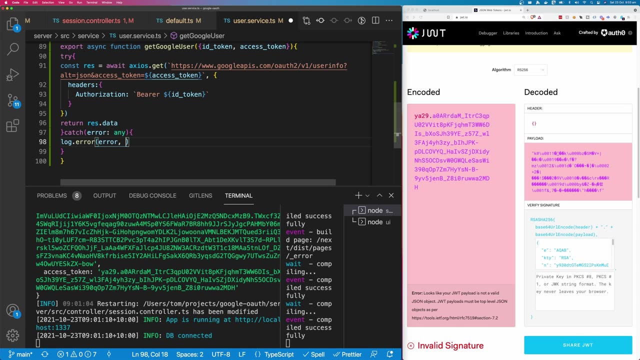 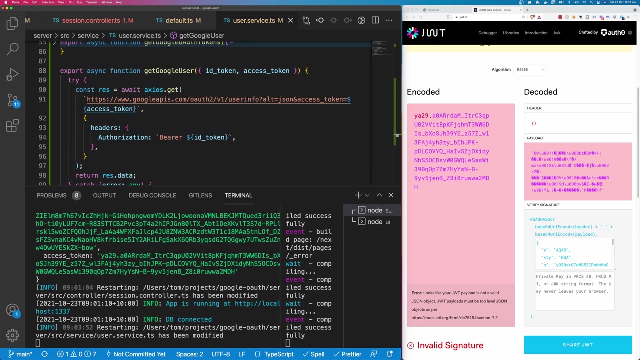 given these tokens here. So now let's just return res dot data. Let's catch our error here. So I'm going to say: log dot error. Add the error: Error fetching Google user. I'm going to throw the error And let's also type this here: 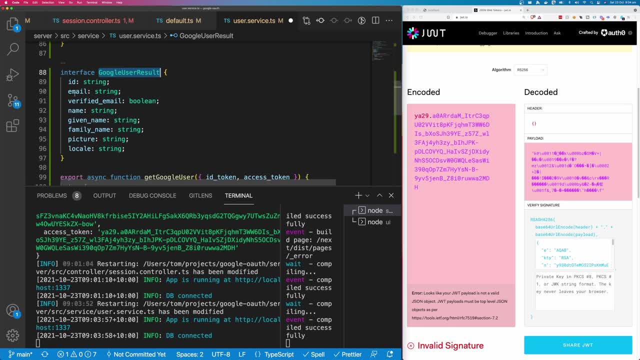 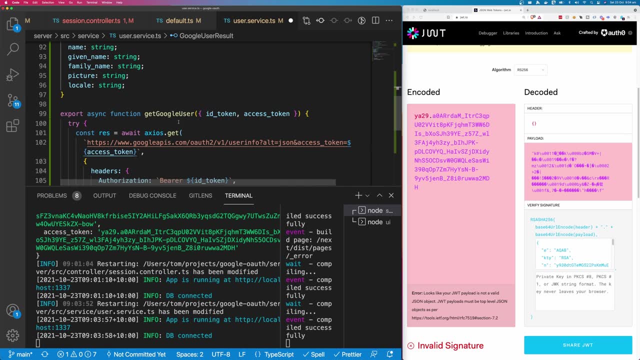 So I'm going to use this pre-prepared interface here So you can see we have an ID, Email, Verified email name, Picture And local. So we're going to say that this returns a promise And the promise includes our Google user result. 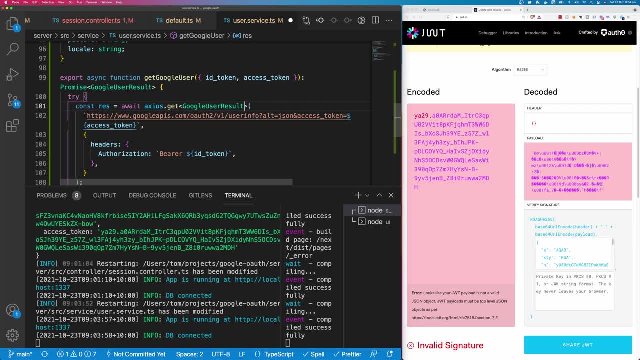 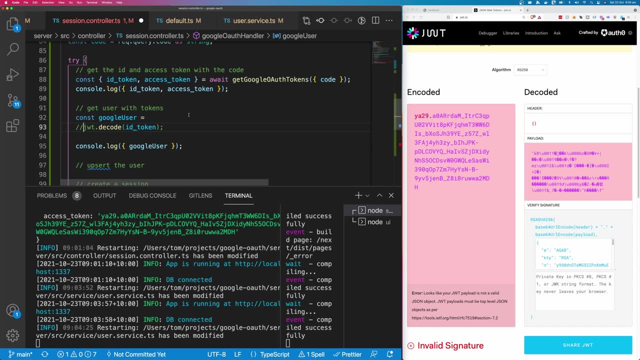 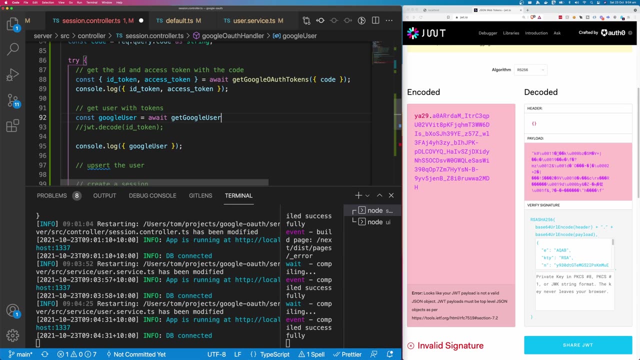 And we're going to do the same with our Axios get. Let's come back to our controller And I'm just going to comment this out here And I'm going to say: Google user equals await, get Google User, And we're going to pass in our ID token. 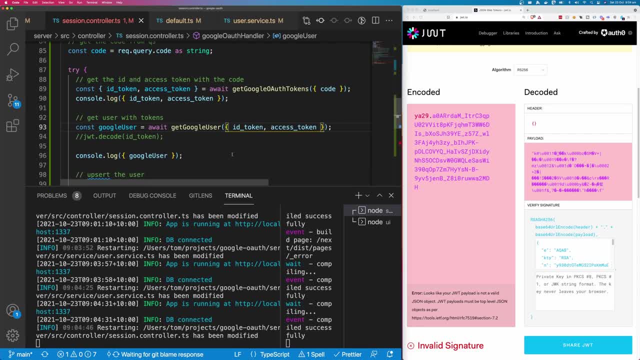 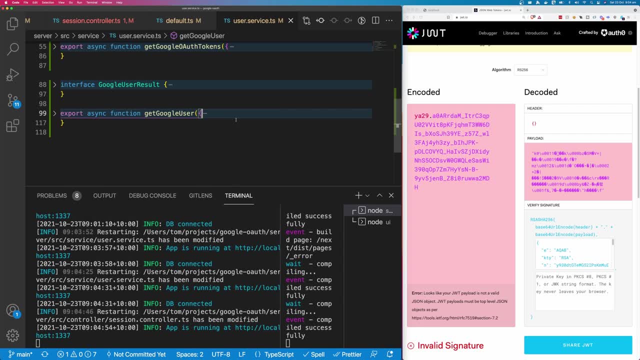 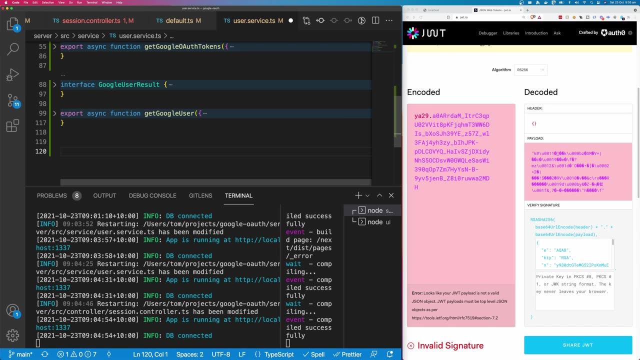 And our access token. So let's move on to upsetting the user. So I'm going to come over to user service And I'm going to create a new service for finding and updating a user. So I'm going to say: export async function. 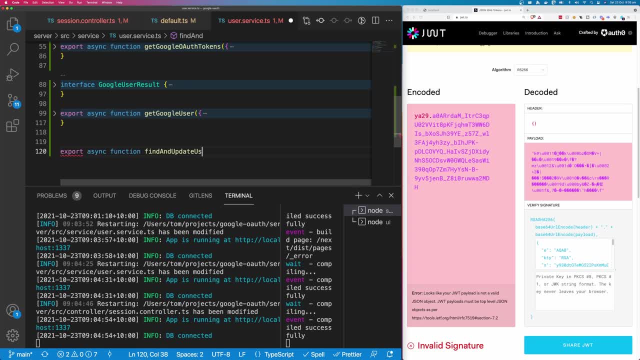 Find and update user. So we're going to have a query, We're going to have an update And we're going to have some options. I need to move these into the argument, So let's type this out. So our query is going to be a filter query. 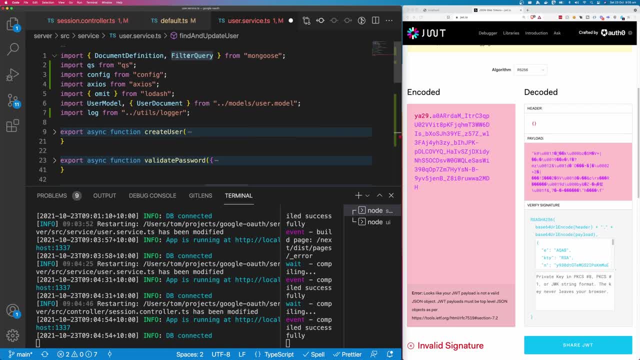 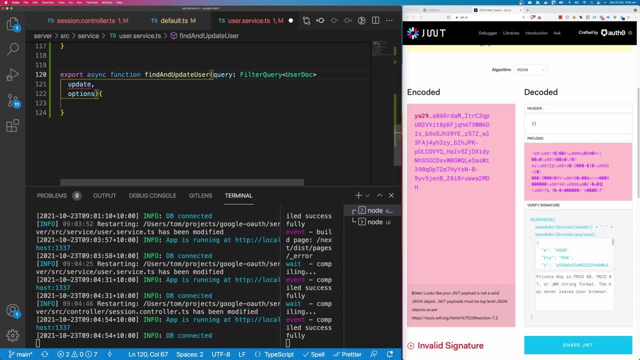 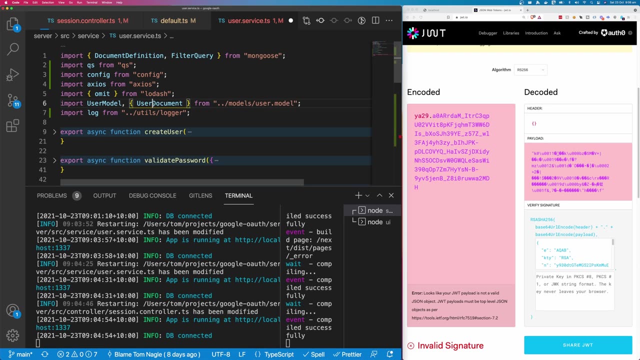 And this comes from Mongoose. So you can see, here we have filter query And we have user document And if you haven't followed the previous tutorials, user document here is just an interface that extends mongoosedocument. Our update is going to be an update query. 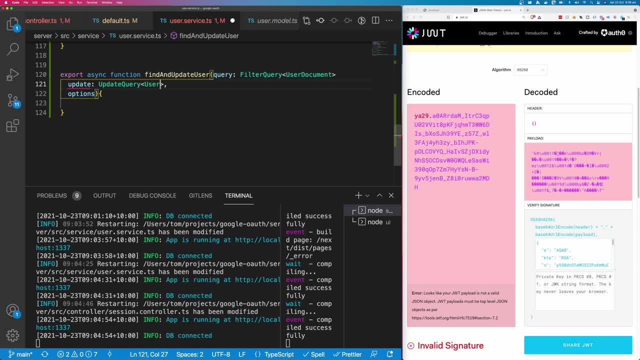 And this is going to take our user document as the generic input And our options are going to be query options, And let's default this to an empty object, Because you don't have to have your query option set. So let's return here. 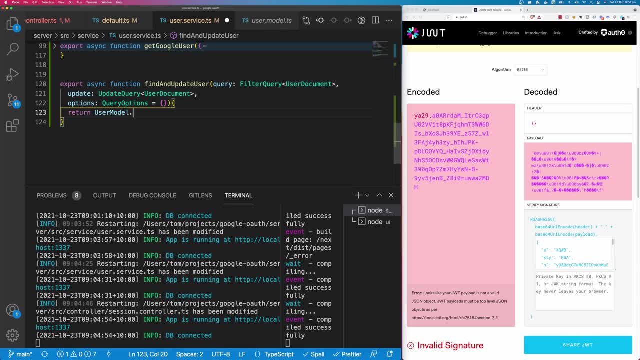 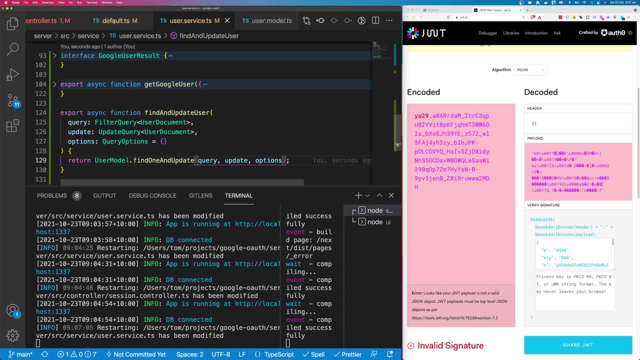 User model. Dot find one and update. So we're going to pass in our query Our update options And our options. So let's go use this function here to upsert our user. You may be wondering why I didn't create a function for upserting a user. 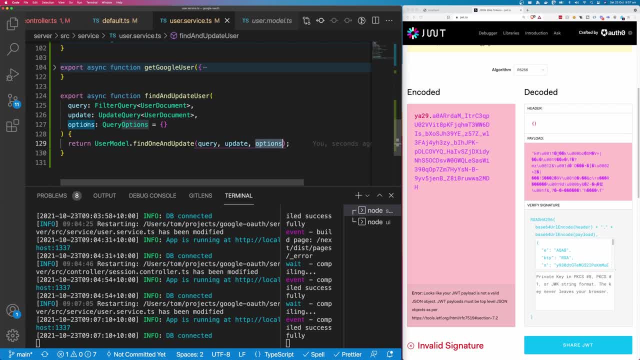 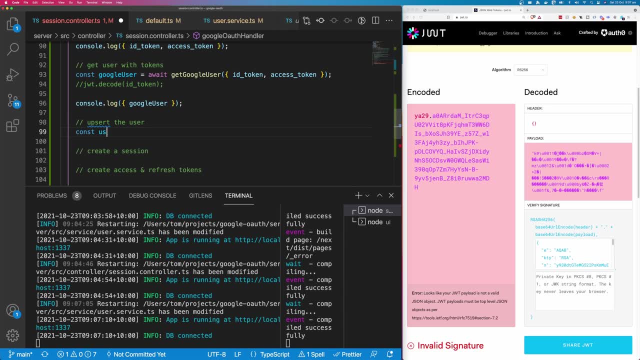 And because upsert is just an option on our options object here What we're actually doing is updating a user. So I'm going to say: const, user equals, Equals, wait, Find And update user. So we want to find the user by the email address. 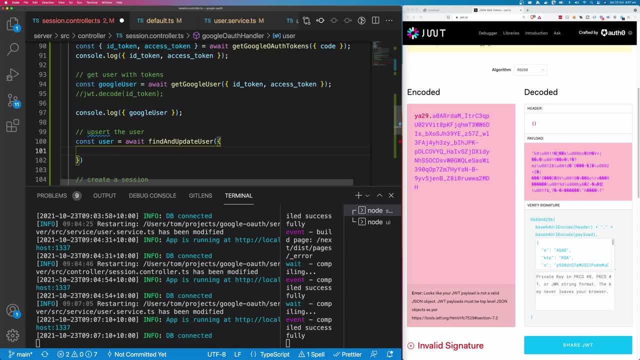 So the issue with this is that if you use a provider that doesn't verify email addresses- Apparently something like Discord doesn't verify email addresses- You could get somebody to create an account with an unverified email address And then they could log into your system with that user. 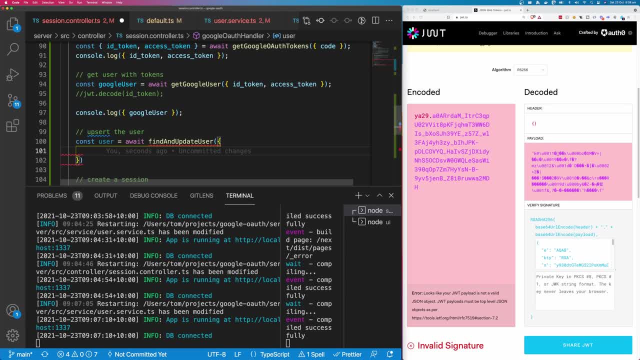 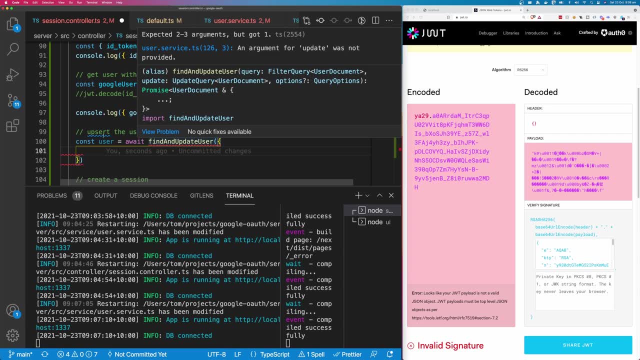 So you need to make sure that you're using a provider that validates email addresses if you're going to do it this way. If you want to, you can also save the Google ID And you can verify them via the Google ID, But that could result in duplicate accounts. 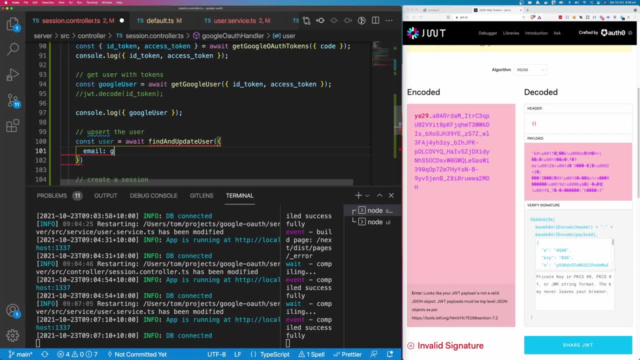 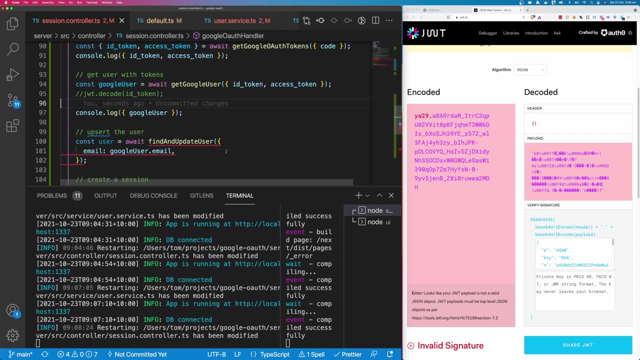 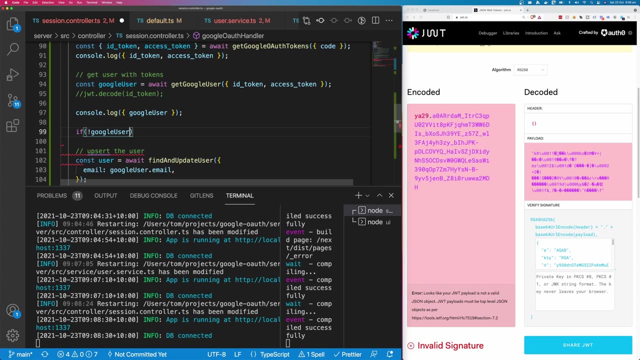 So I'm going to say email And then I'm going to say Google User Dot email. And to double check this, I'm just going to say Up the top here, If Not, Google User Dot Verified email address. 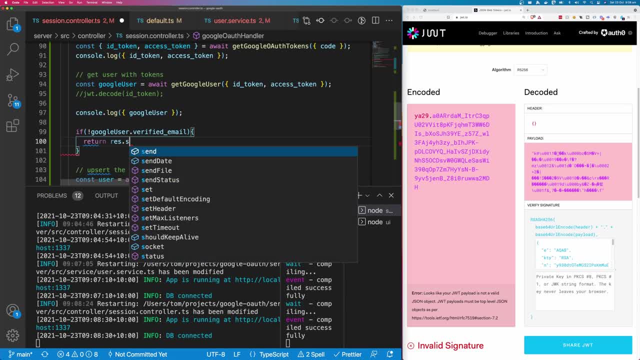 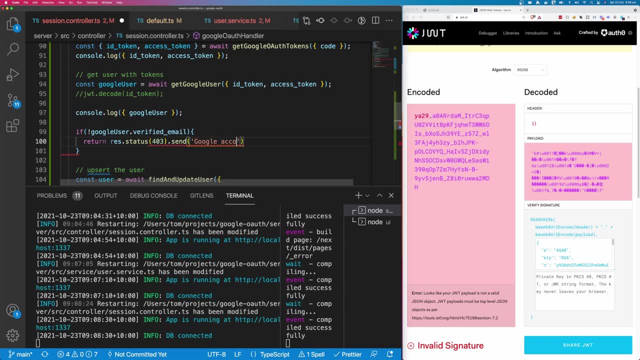 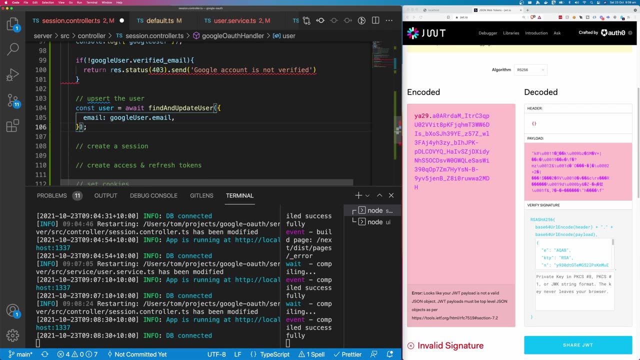 Then we're going to throw an error. So I'm going to say return Res Status 403.. Send: Google Account Is not Verified. So we're just enforcing that the user has verified the email address And I'm also trusting that Google has done this process correctly. 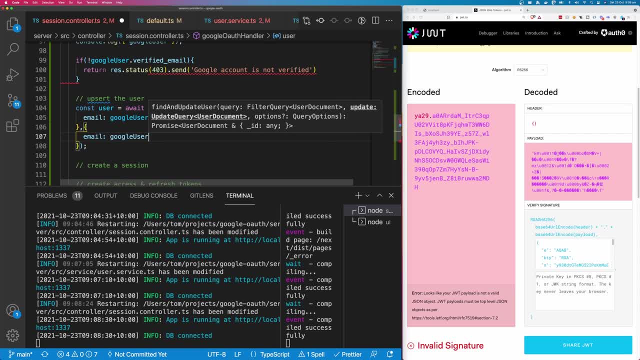 For email, Google User Dot Email. So you may be wondering: we're finding the user by the email, But then we're also updating the email And this is because we're going to upsert. So if the user doesn't exist, we need to provide this email address here. 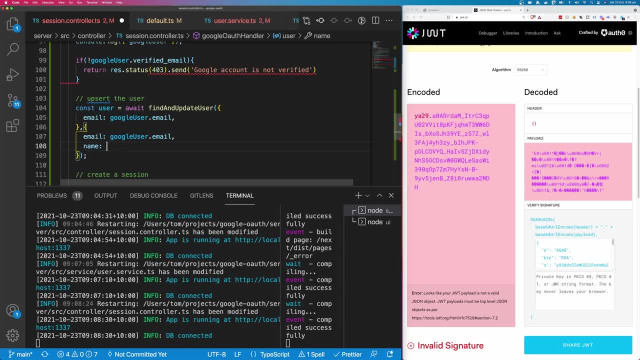 So we can create them with that email. I'm going to say name: Google User Dot. Name Is Google User Dot Picture And we don't have this picture on our model, So let's add that. 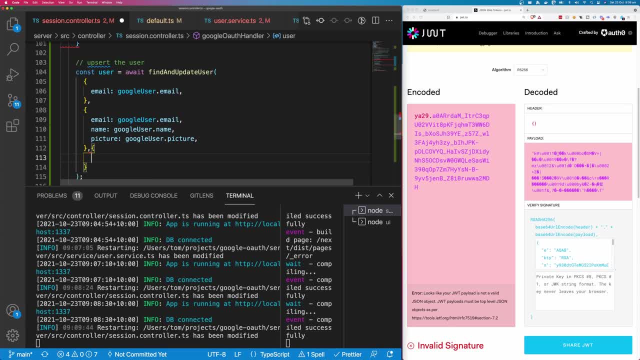 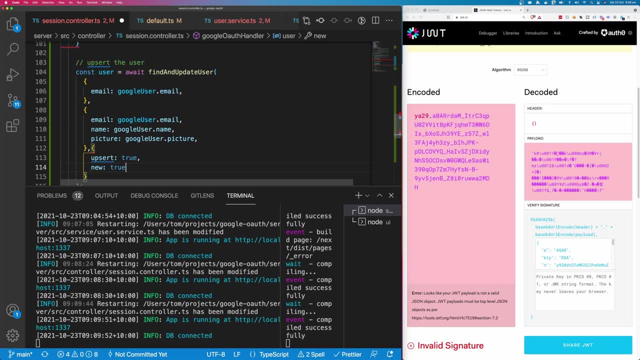 But before we do that, let's add our options. So we're going to say upsert Is true And new Is true. So new just means that it's going to return the new document, given that it's updated this user. 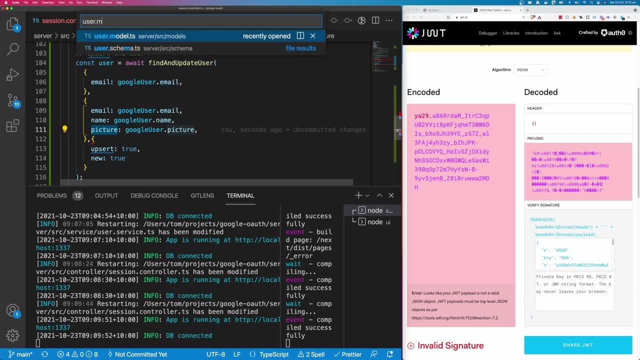 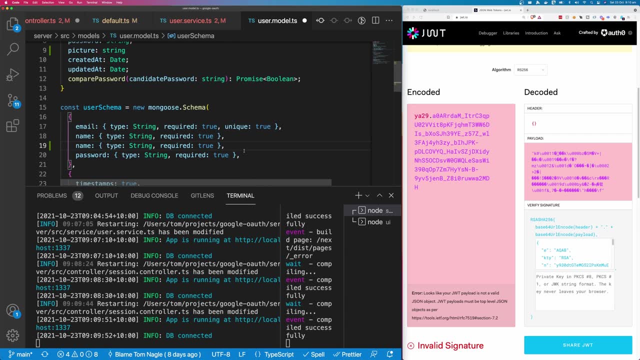 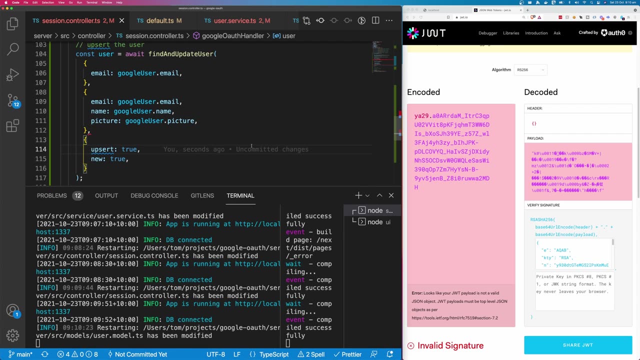 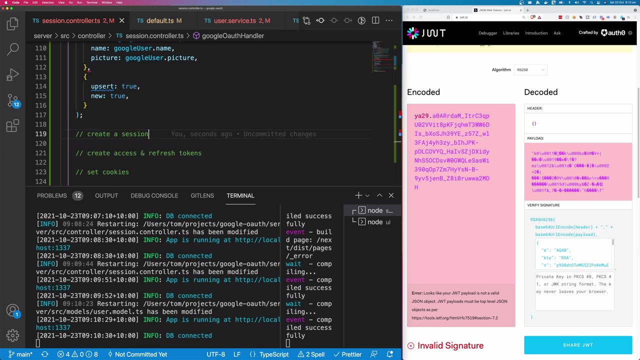 Okay, So let's add picture to our user model. Picture is going to be a string And it's not required. Save this. Okay, So let's assume this has worked correctly And we're going to move on to creating our session. 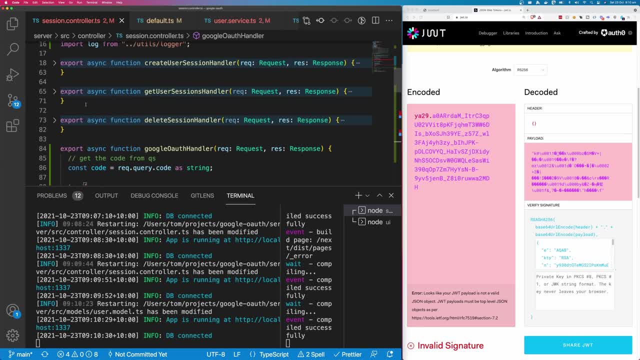 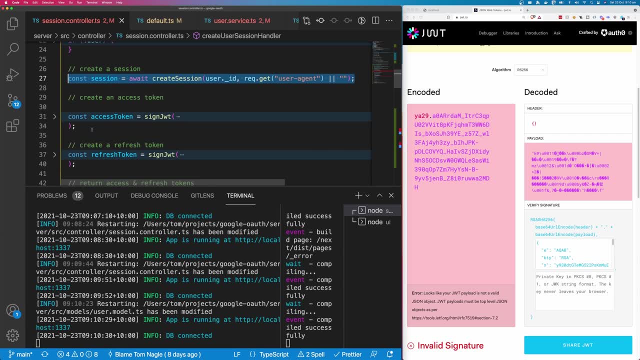 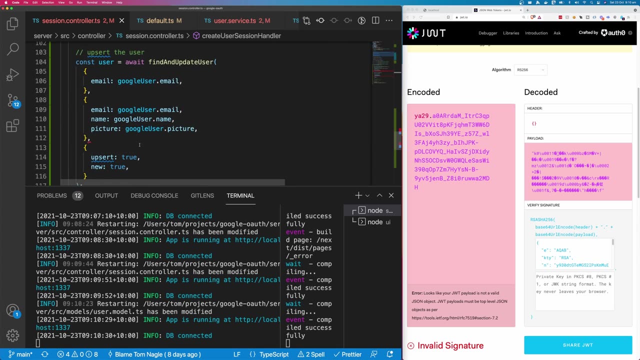 So we've created a session before. Create user session handler. So let's copy this here. In fact, let's copy all of this here. We're going to create a session, create access token and create a refresh token. This all looks good. 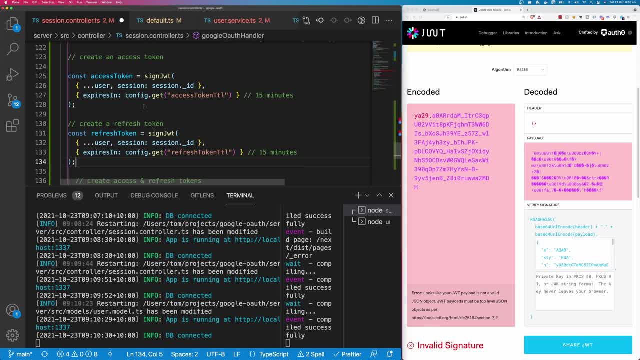 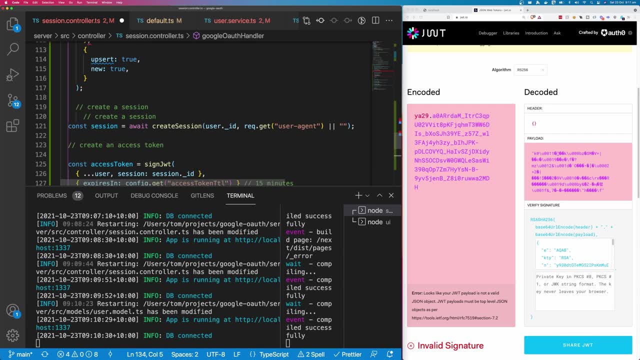 I'm going to copy this And paste it down here. So we have this create session service that we created earlier And it's going to create a session for that user ID. We're going to add the user agent to the session so we can see where the user logged in or what browser they logged in with. rather, 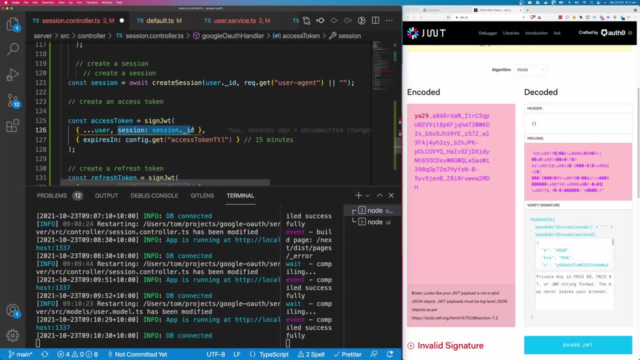 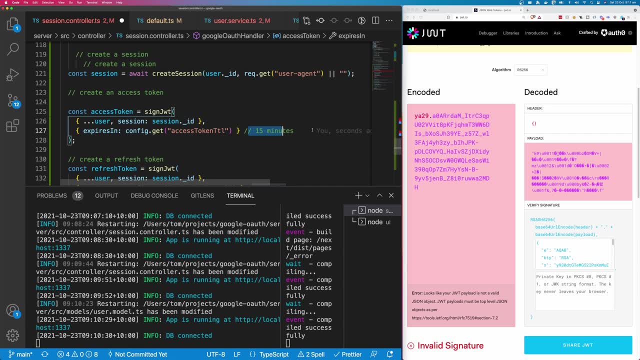 We're going to create an access token with the user. We're going to assign the session to that access token as well. We're going to say that this access token expires in our access token time to live, which is currently set to 15 minutes. 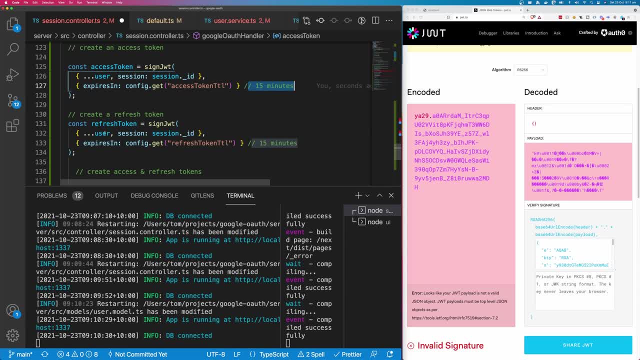 We're going to create a refresh token, We're going to spread the user, We're going to add our session ID, We're going to add expires in and our refresh token time to live, which is not 15 minutes, It's actually one year. 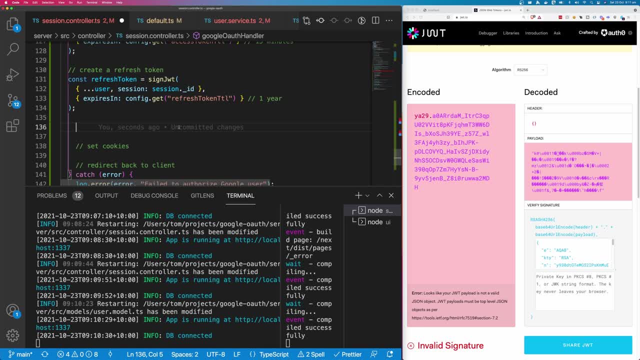 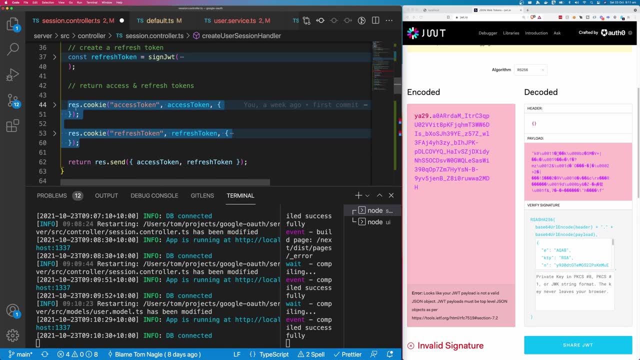 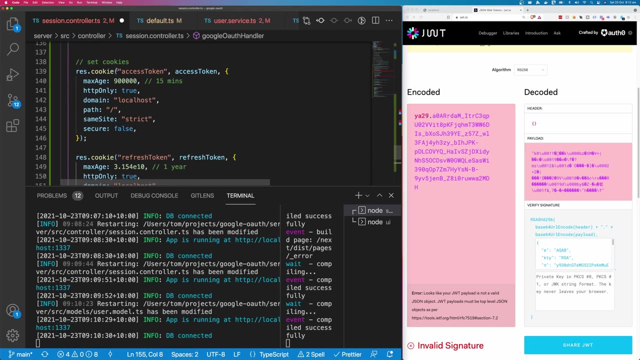 So we've done this part down here. Now we need to set cookie And if I remember correctly, we have already set cookies up here And we have. Let's paste this in here. So we're going to say rescookie in. 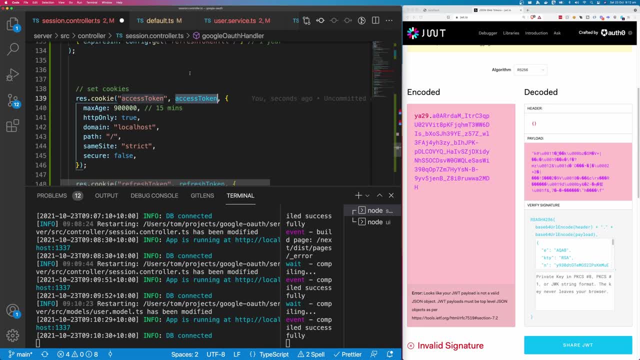 So we're going to say rescookie. I'm going to call this one access token. We're going to assign the access token that we created up here to the value of the cookie. We're going to set its max age to 15 minutes. 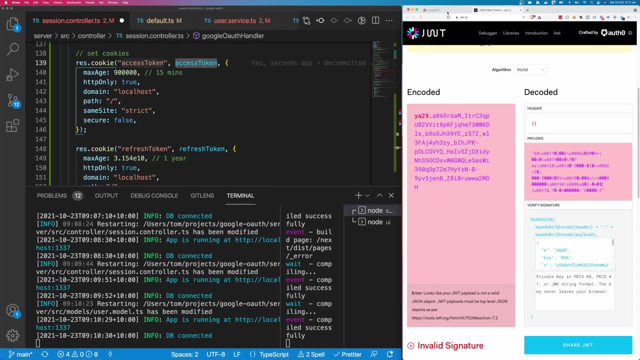 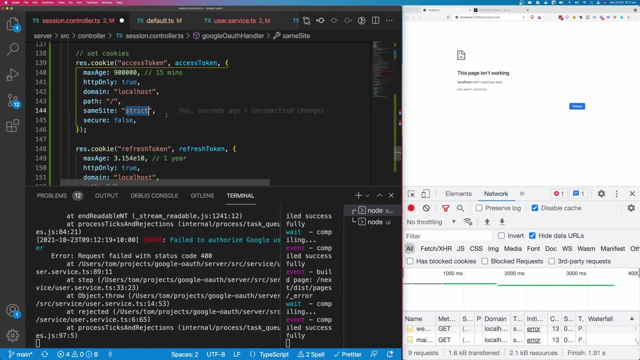 Hp only is true. Domain is set to local host, because that is what we're using. You will want to get this from config. We're going to set same site to strict And then we're going to set secure to false. We're going to do roughly the same thing with the refresh token. 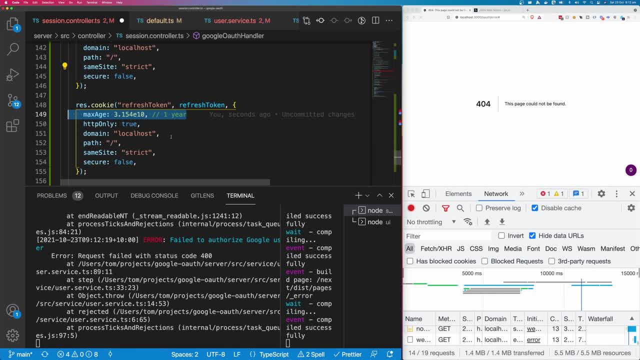 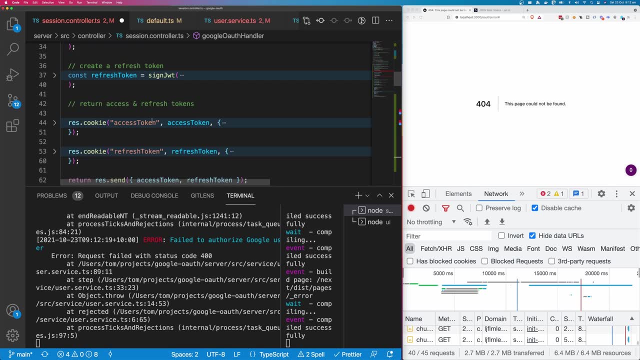 We're going to say max age And we're going to set this to one year, And then the rest of the options are the same. So we copy this from above, which means that all of these options are being duplicated in this get user session handler. 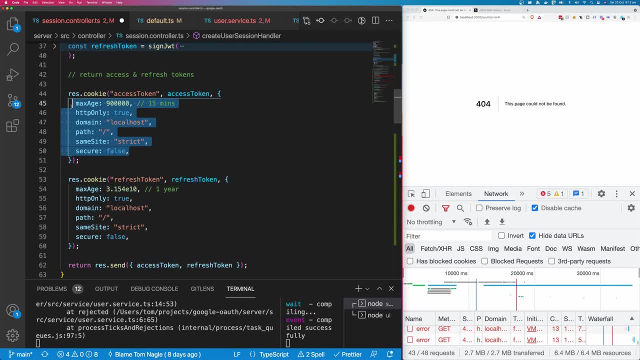 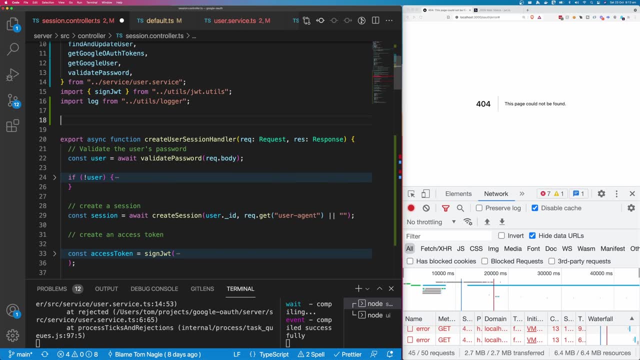 So let's copy out these properties and make some constants So we can guarantee that when the user logs in with username and password and with Google OAuth, that they get the exact same session tokens. So I'm going to say const access token Cookie options is equal to. 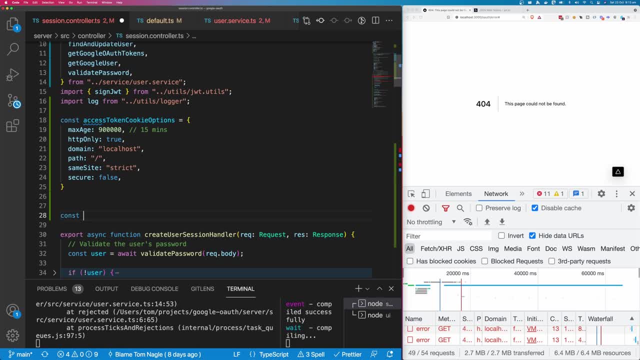 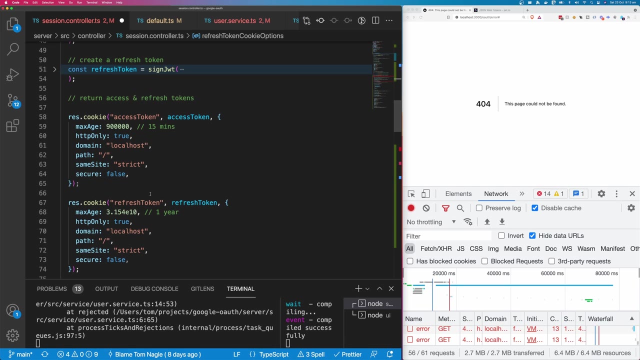 And I'm going to copy this. So const refresh token Cookie options is equal to Options, is equal to an object. I'm going to spread on the access token options And the only thing that we need to change is this: max age. 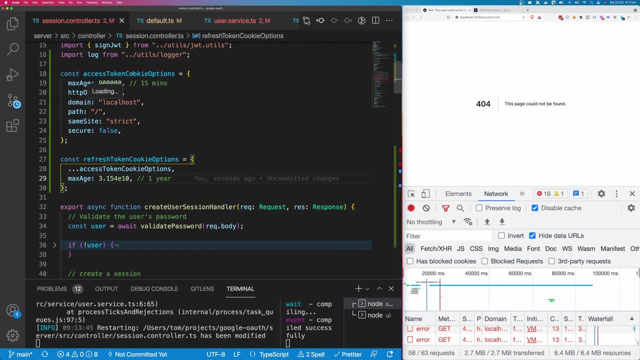 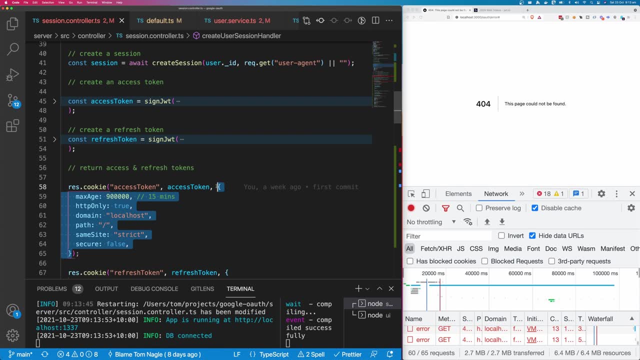 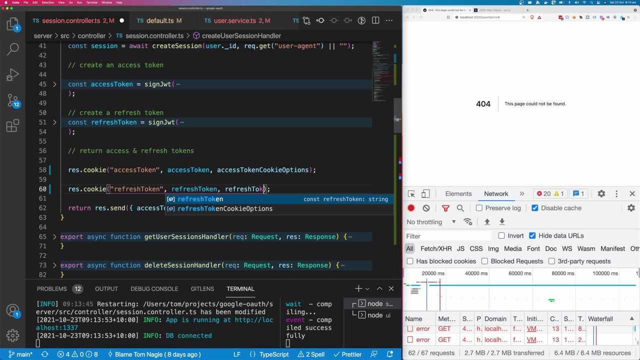 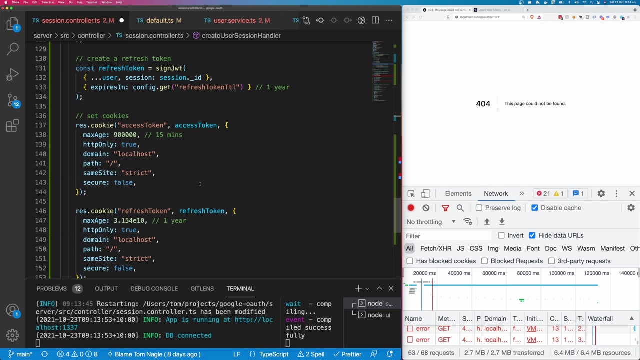 Put it down here to make sure it's overwritten from this max age And we can copy these options and paste them. Let's paste that here And we can set this to refresh Token Cookie options. Let's copy this And we can do the same down here. 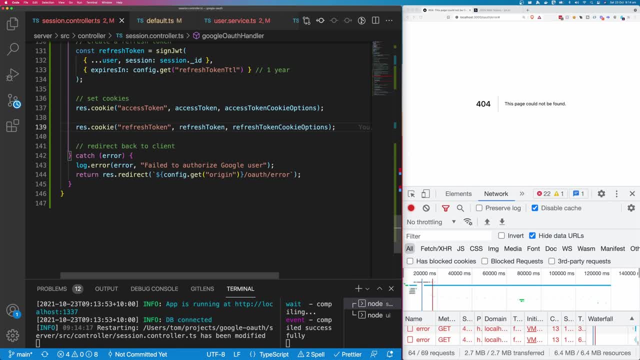 And this looks good. Okay, So the last thing to do is redirect back to the client. So I'm going to say res dot redirect And I'm going to use this config dot Get And I'm going to send them back to the origin. 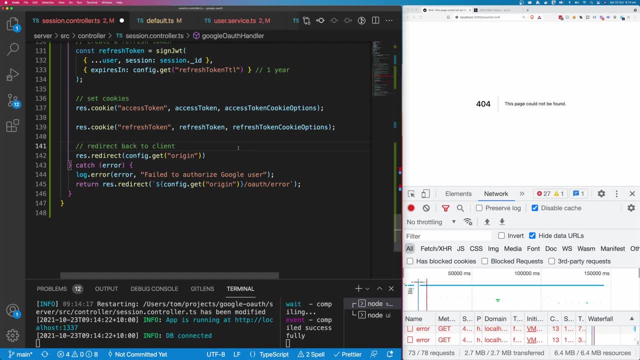 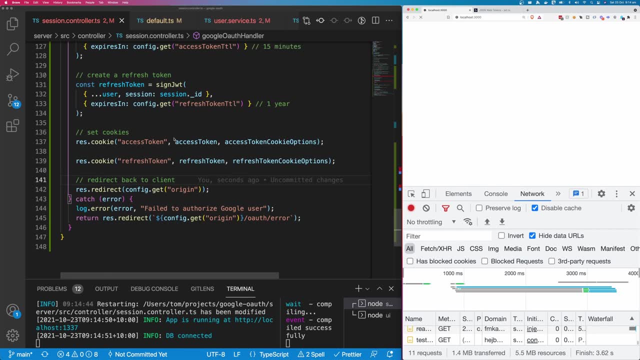 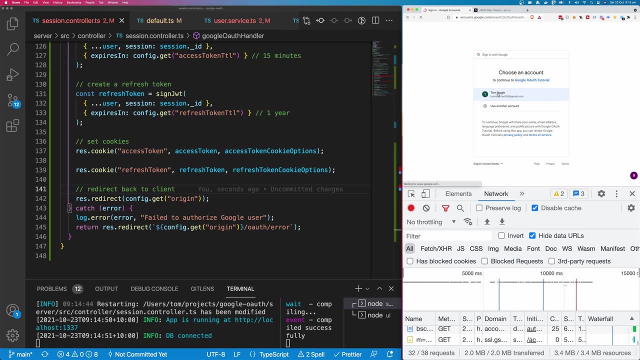 Which is just our client. Save this And we're ready to try this And we're going to hope that it works end to end. Login And you can see here that we have logged in Because we have our user here. So let's check our cookies and make sure that they're set. 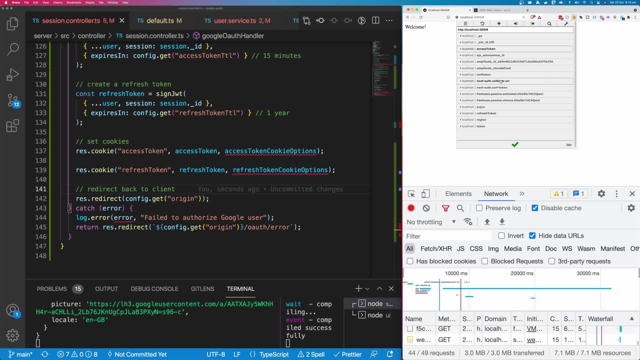 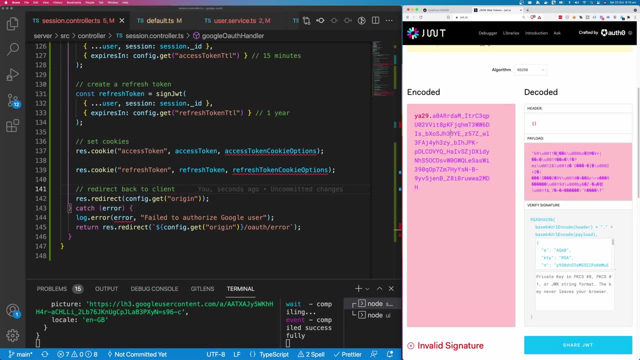 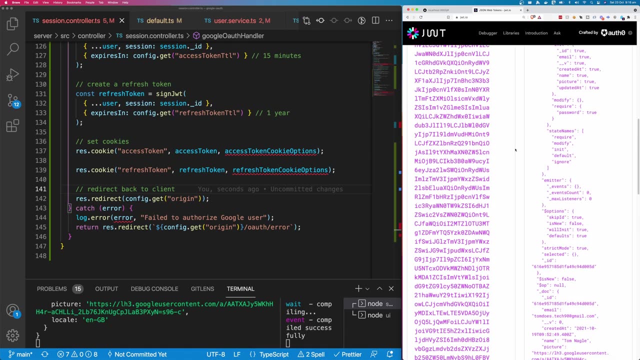 So you can see we have an access token here And we should have a refresh token as well. Yep, That's down here. Let's go to JWT dot IO And check that our access token is looking good. So you can see here that our access token looks a little bit funny. 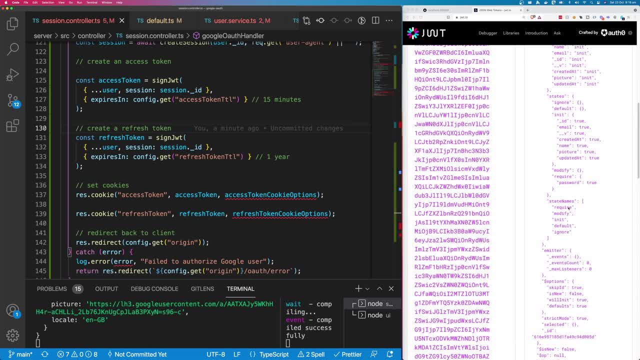 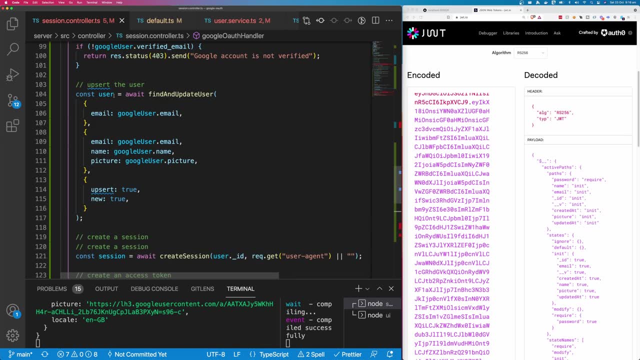 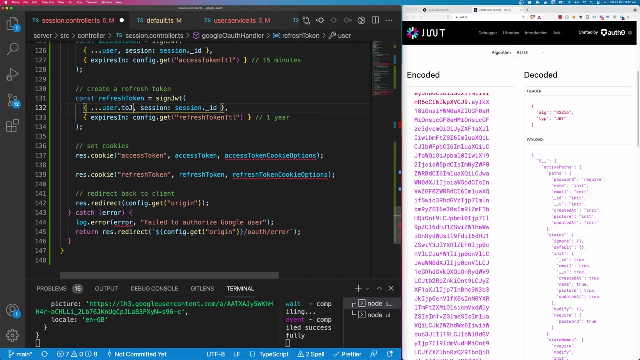 Got all this stuff in here And this here looks like we need to call to JSON on our user object. So you can see up here that we've created our user But we need to convert it to a JSON object. Let's go to JSON. 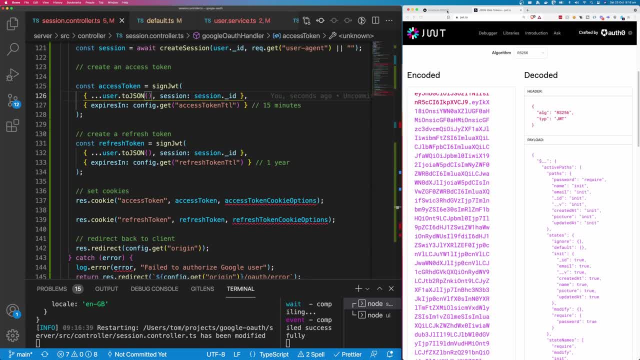 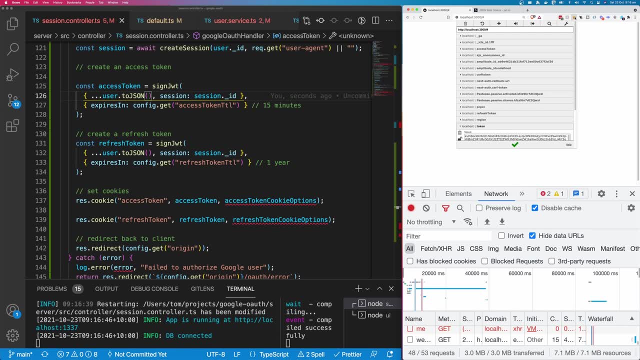 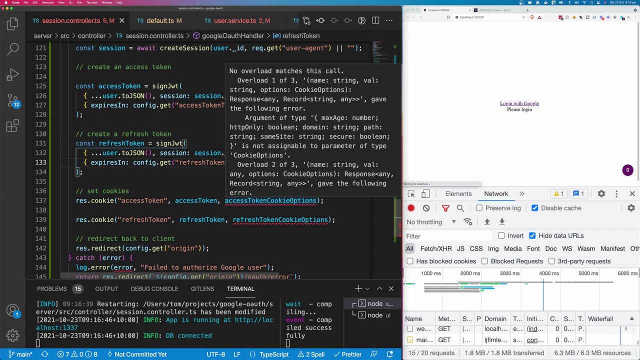 I'm going to copy that And I'm going to do the same for the access token. Let's come back to our application here. I'm going to open up my cookie editor And I'm just going to clear out all the cookies to make sure that we're logged out. 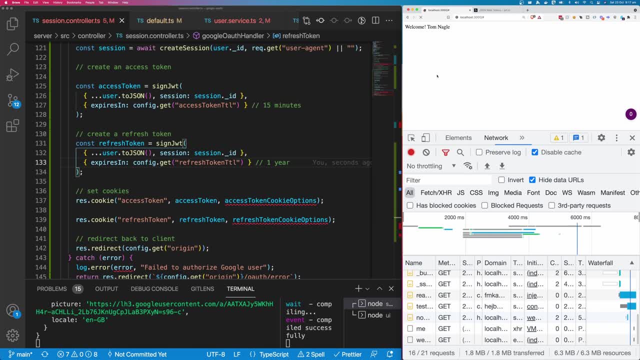 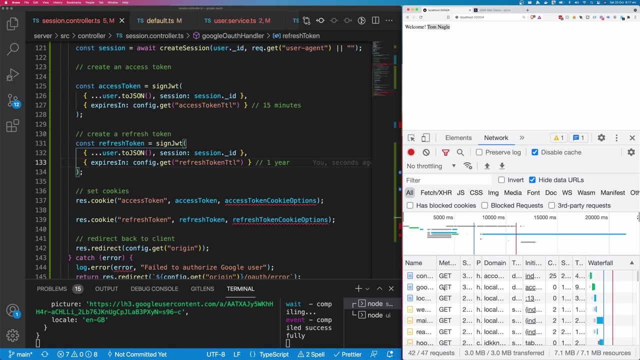 Try login again And we're logged in And we get our name here. Our cookie must be good. If you saw the login flash there, that is because if we have a look at the get request back to our local host, my suspicion is that we're not sending cookies along with this request. 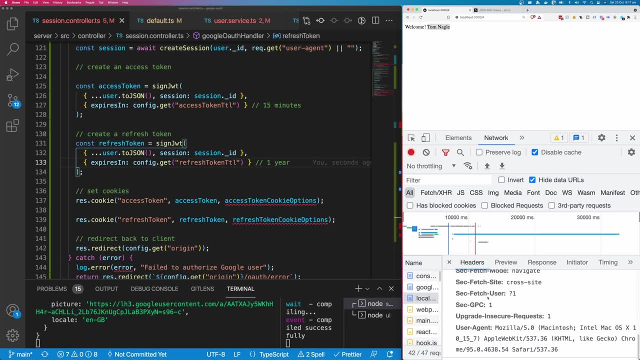 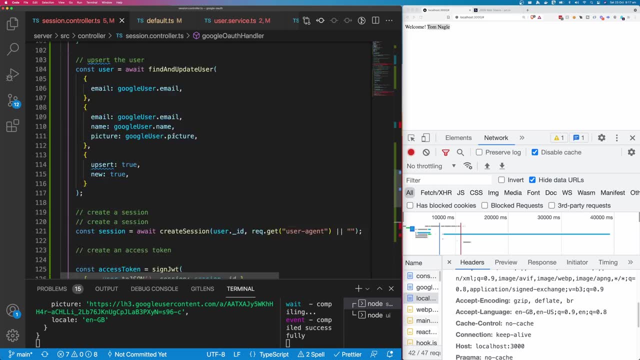 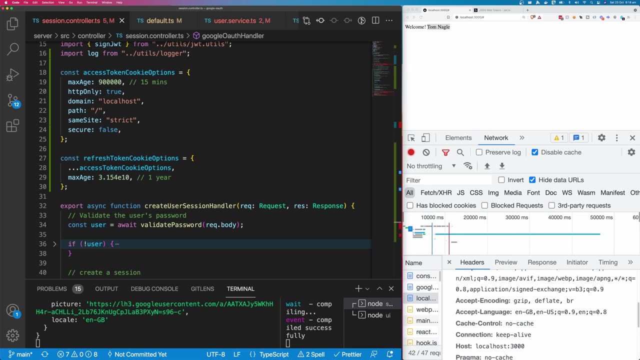 So request headers And there's no cookies here. So the reason for that is going to be our cookie policy that we have defined at the top here. So I'm going to set the same site policy to lax and see if that helps. And while we're here, let's fix these TypeScript errors we have. 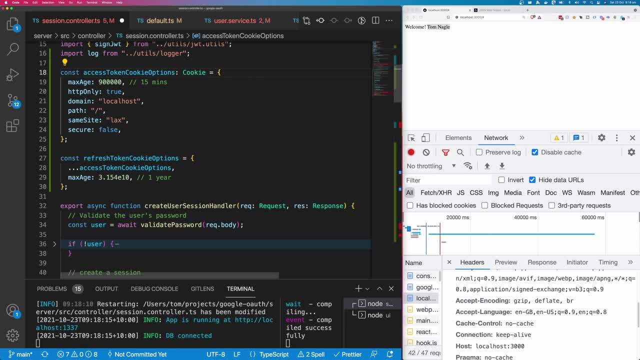 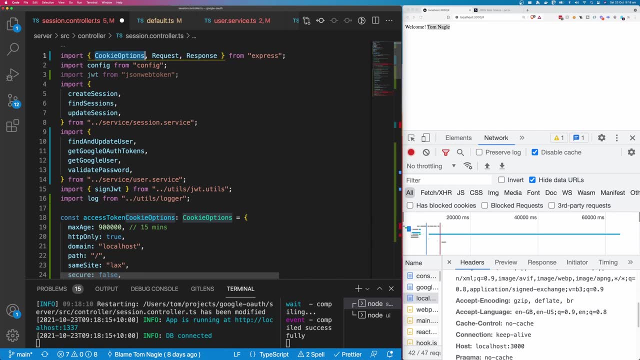 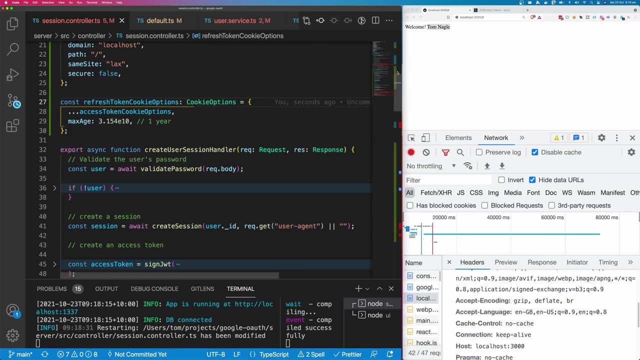 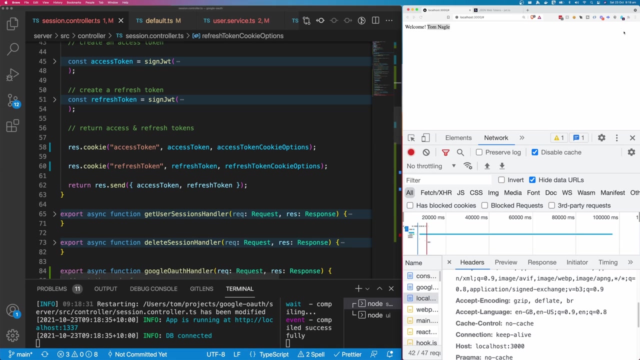 So I'm going to say these are cookie options And this just comes from Express, So you can see this is imported here. Do the same with our refresh token options And you can see TypeScript is up here. Let's clear our cookies.